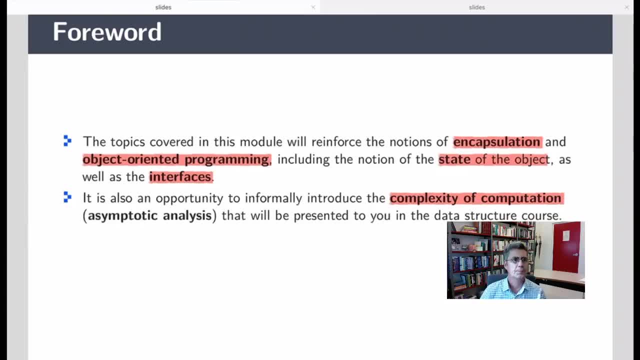 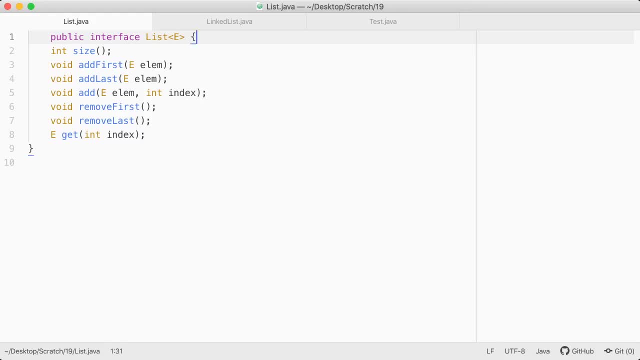 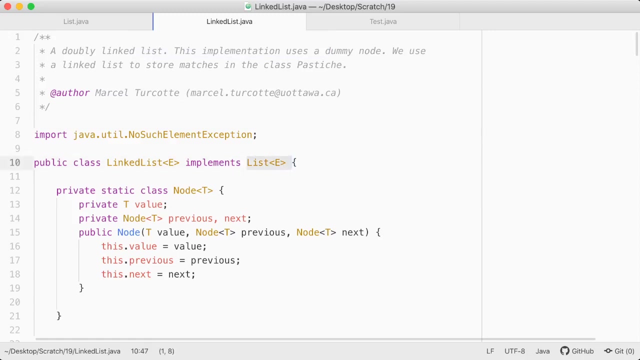 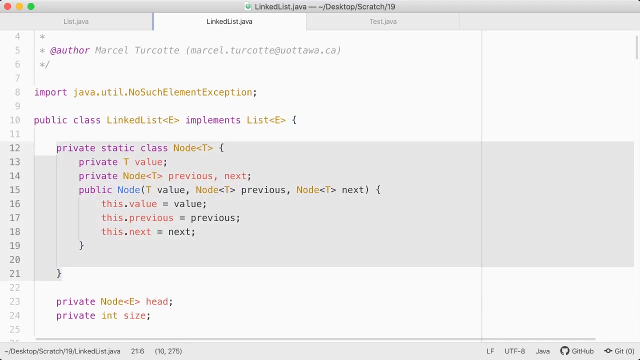 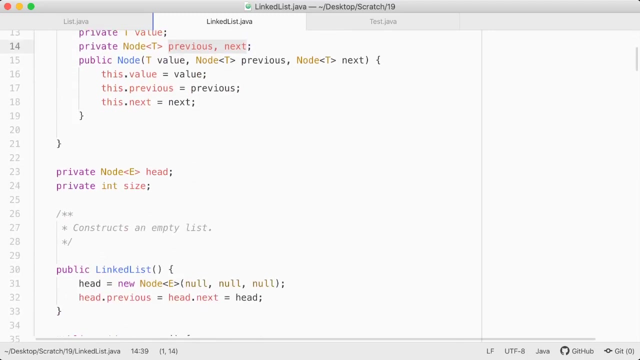 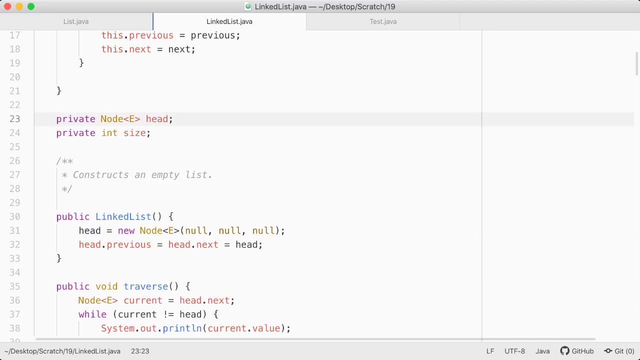 So what is it that we want to do? Let me show you. So I have the interface list and the interface list here is telling me that a list has some method size, some methods for action, adding elements, removing element and a method get that returns the value stored at the position designated by index. I see that the indentation is not as it should. So here we go. So there's an implementation of the interface list and when I'm programming I decided to reuse our last implementation for the last lecture. So this is the one where I have a class node, static nested class node, and as you can see the nodes are doubly linked. This is also the implementation that is circular and it's using a dummy node. So you see here head. 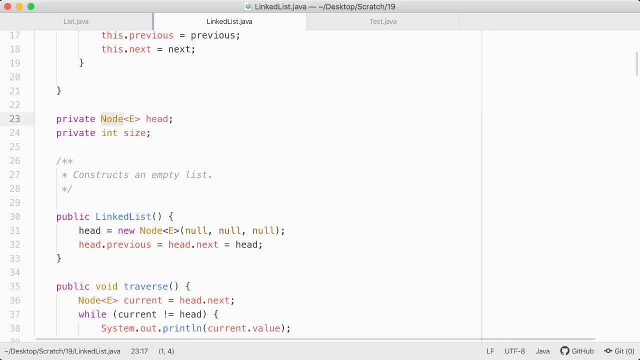 I only have one variable of type node for an object of the class linked list and so this is the one where I have a class node and I only have one variable of type node for an object of the class linked list and so this 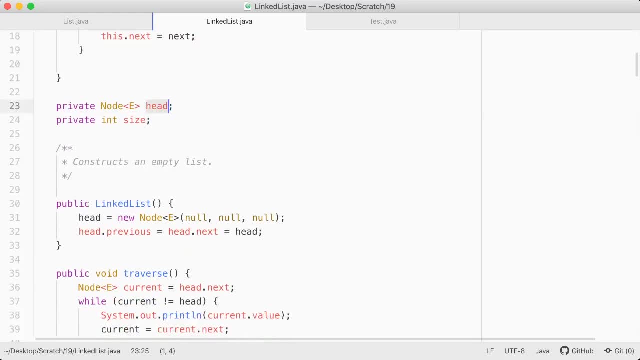 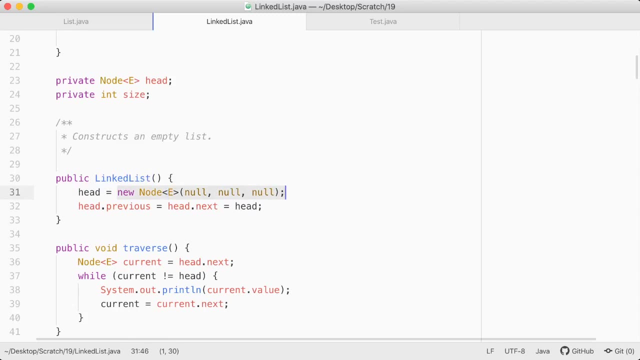 variable head will be pointing at the dummy node always. In constructor when a new list is created this is where the dummy node is created, it will never store any information. It's not designed to store information. Its only purpose is to make all the operations simpler by removing special cases. And here is the place where I make the list doubly circular so head dot next is pointing at head itself and head dot previous is 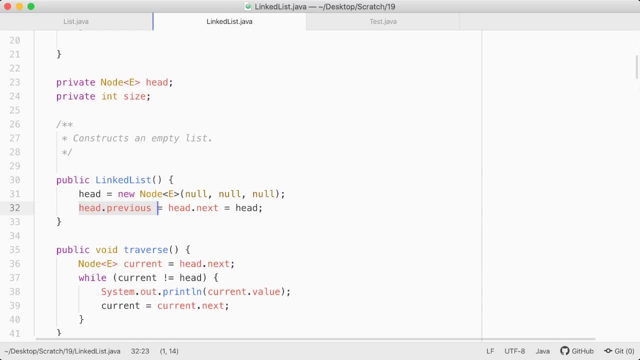 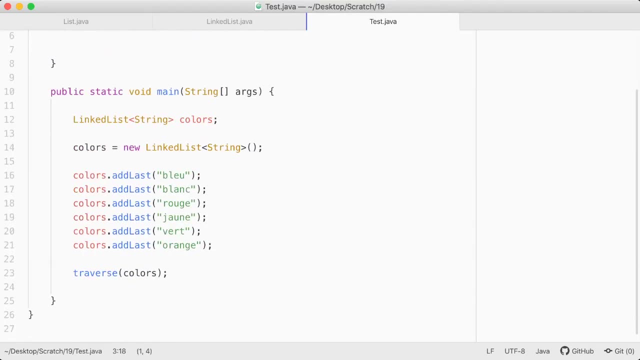 pointing at the dummy node itself and here is an example where i'm in some class called test i am declaring a variable called colors to be a reference to a linked list object creating the linked list and i'm adding some strings blue blue orange so i now have 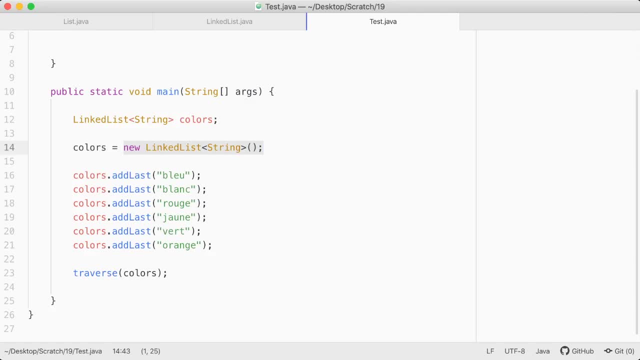 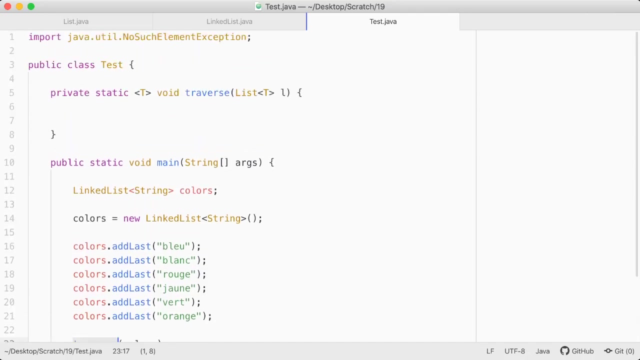 one two three four five six elements inside this list here i'm writing a method to traverse the list to visit all the element the elements and print their value i'm writing this inside the class test 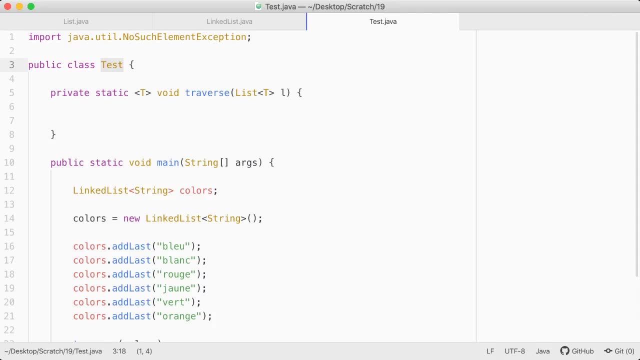 clearly i'm not inside the implementation of the linked list so in order to do my work i can only access the methods of the interface list 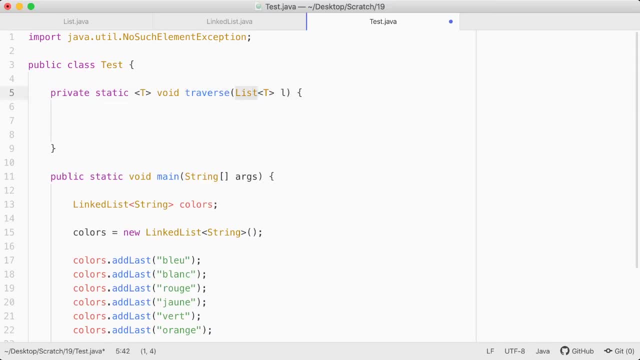 in particular in the method traverse because that's the type of the parameter so here we go for some int i equals zero i is smaller than the size of the list that's i cannot access any instance variable so i need to call the method size i plus plus 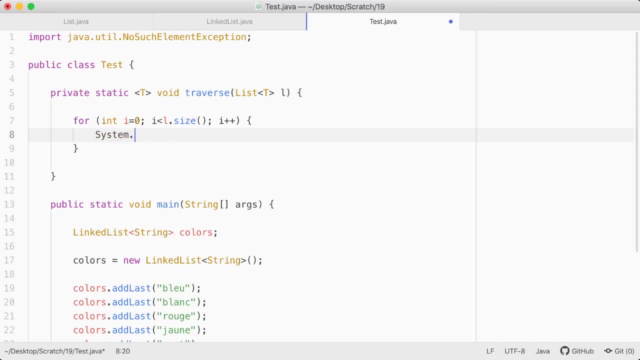 i'm going to print so system out print line and the only method that allows me to to read or or to obtain the content of an element at a certain position it's the method get so i'm using this save let's compile the test 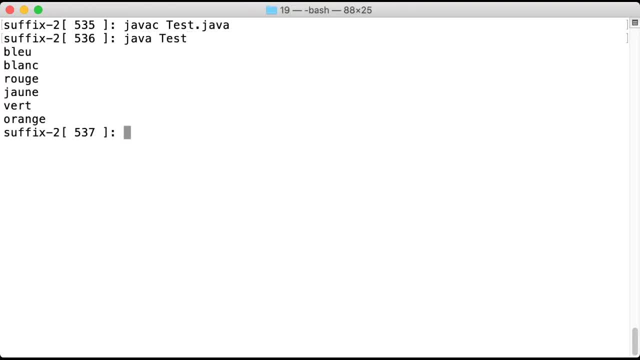 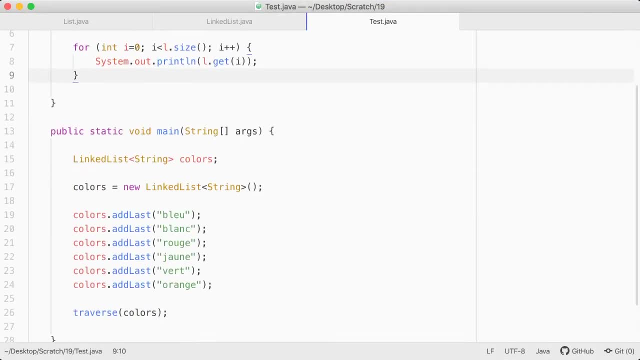 let's run okay so i simply wanted to print the content of the list i did that when i was outside of the implementation 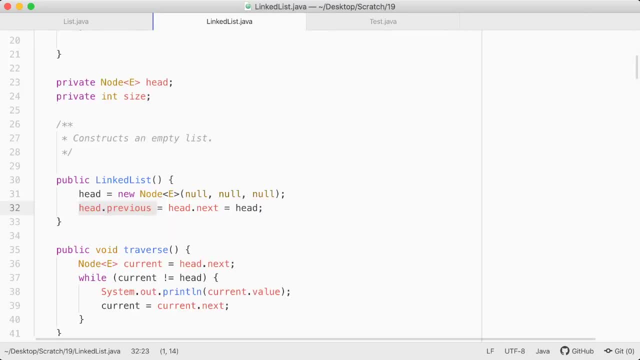 let's do the same thing inside the implementation of the list i've already i already have the code here a method traverse 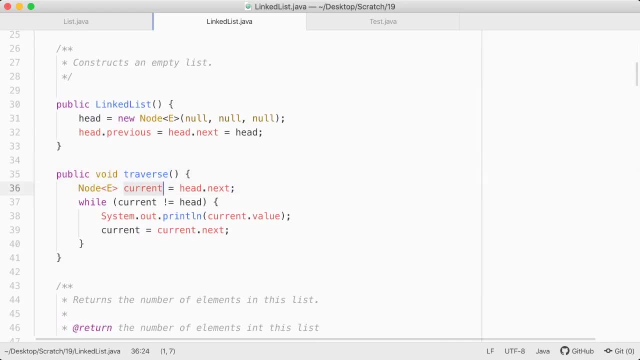 i'm using a variable of type node i'm calling it current because i'm in the implementation where there's a dummy node i will make current point at the first real node i will landed on my paisa 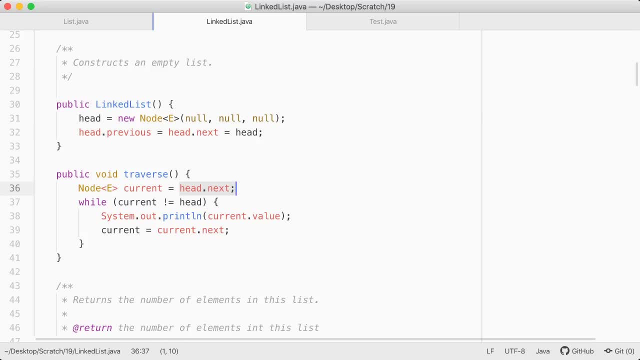 real element. I'm gonna say 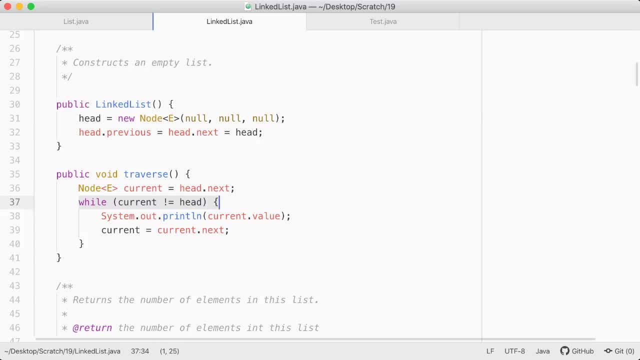 while current is different than head, go inside the loop print current.value, move forward. 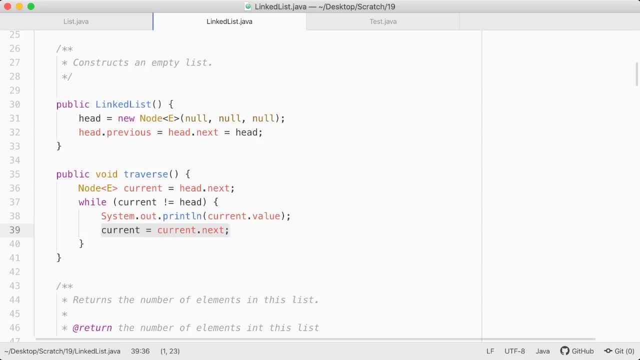 Imagine the case where the list is empty there's only the dummy node. When I say current equals head.next, head.next is pointing at the dummy node itself. 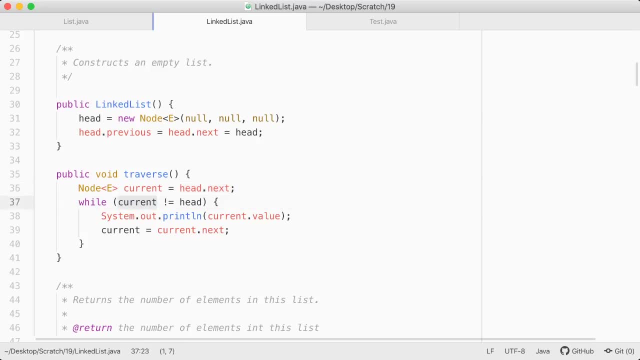 When I test this, current is pointing at the dummy node, so therefore current different than head is false, so it does nothing. 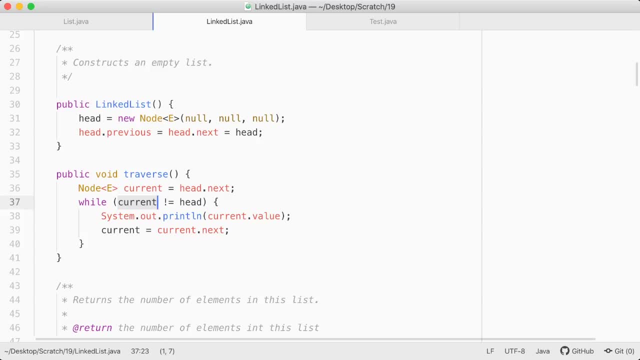 If there's only one element, current equals head.next, current will now be pointing at that element. Here, current is therefore different than head. We print current.value, we say current equals current.next we're moving forward in the list and now because there was only one element, it was the last one of the list current.next was pointing at the dummy node so therefore when I test is current different than head it says false and we exit. So you see the picture. This will work all the time if the list is empty if it has one, two, three, four elements, it will print them all. 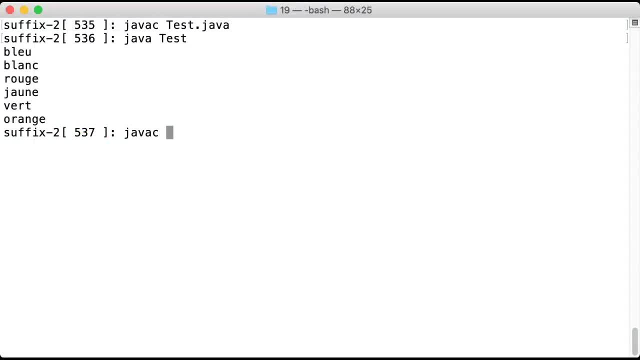 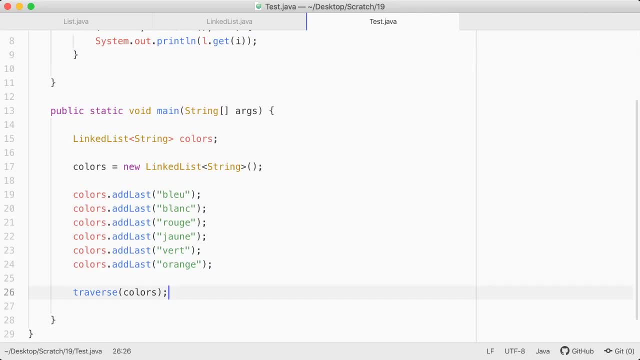 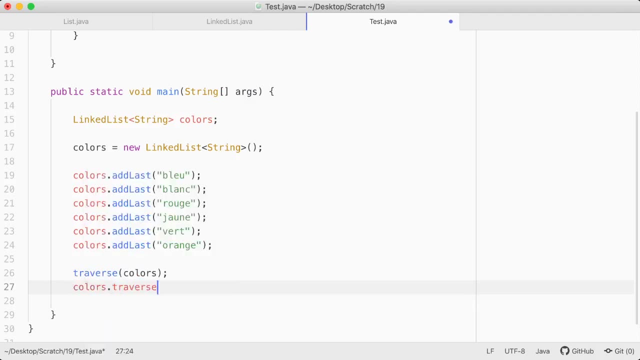 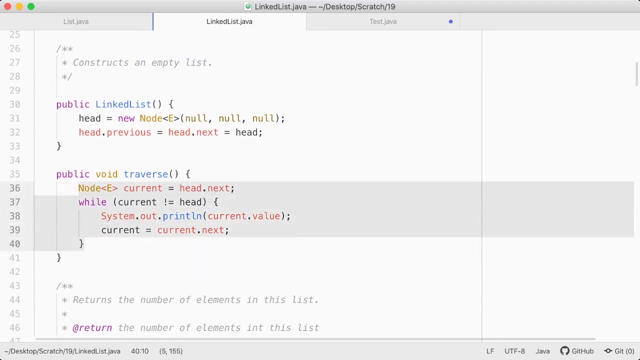 Okay let's compile our linked list.java. That compiles very well. Let's go here so here colors has a method called traverse and we're calling it okay so it's we're calling the method traverse of the object designated by colors here because I'm writing the code inside the 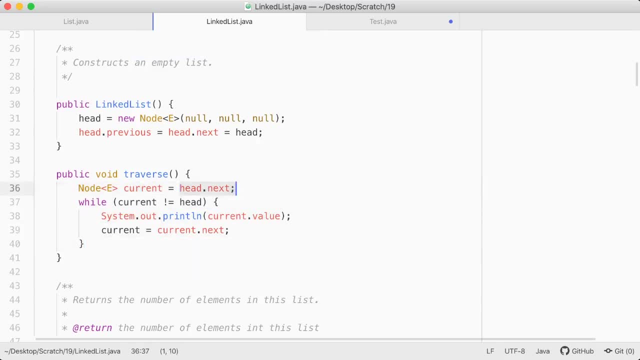 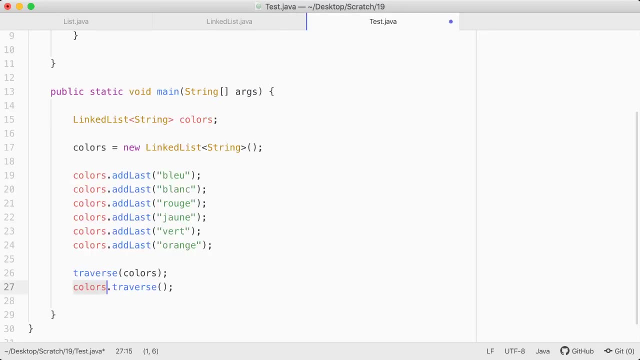 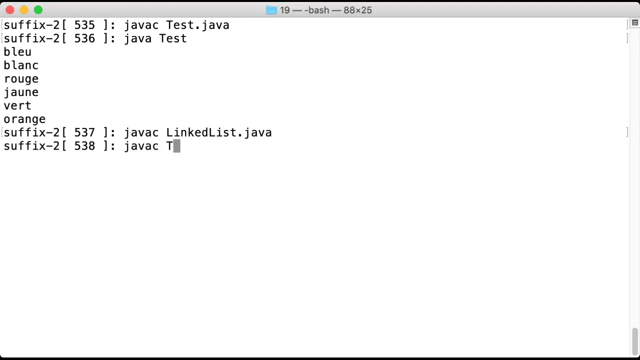 implementation I do have access to head dot next and I don't need to use the method yet let's save this let's compile the test java C test Java Java test okay 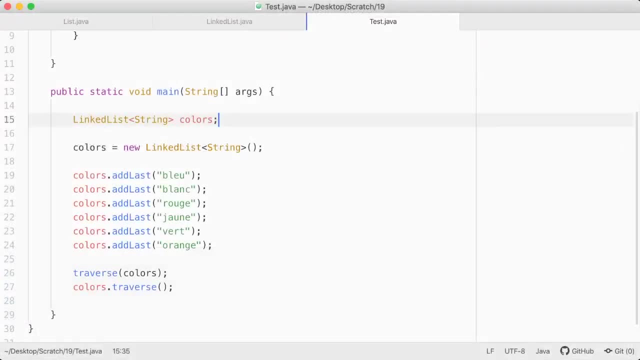 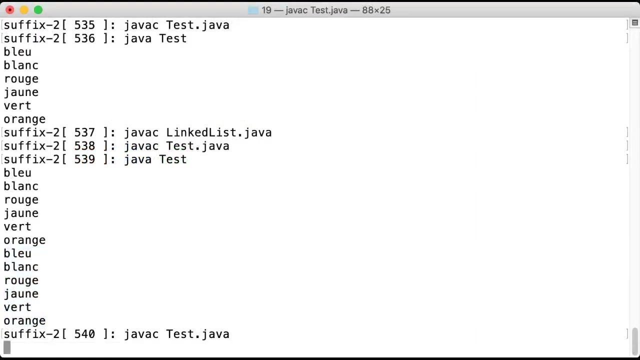 so you see we could have done a better job here let's fix this system out println outside system out println inside so that it's pretty let's skip a line like this compile our test run this 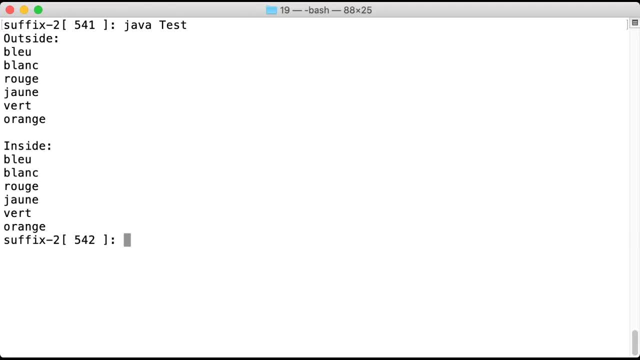 , okay so outside and inside are doing exactly the same work we're printing all 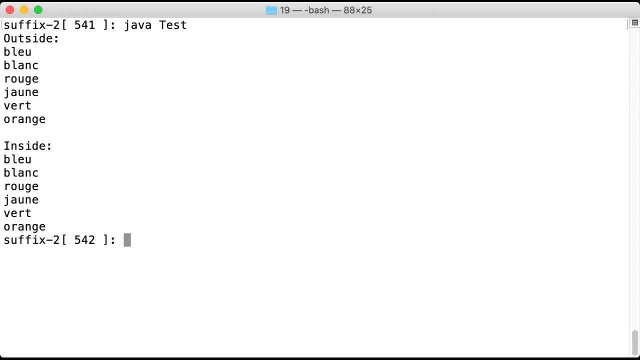 the elements and now what we are interested in is to talk about the 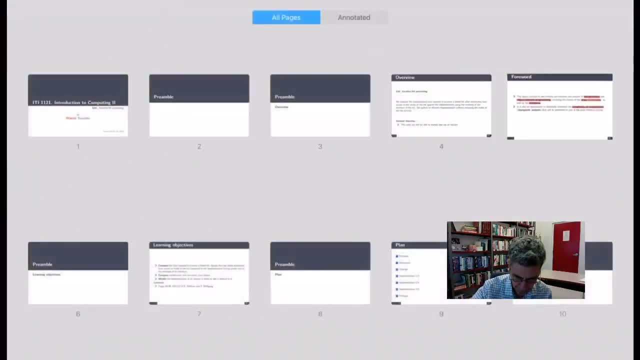 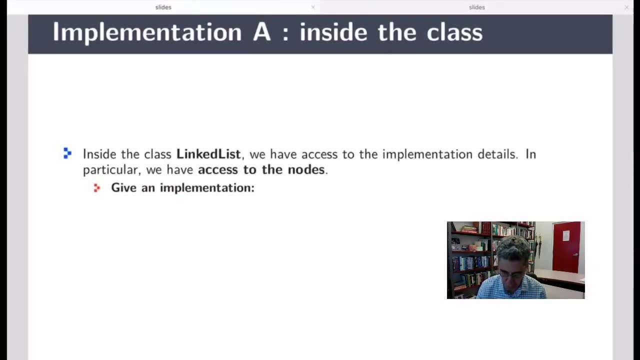 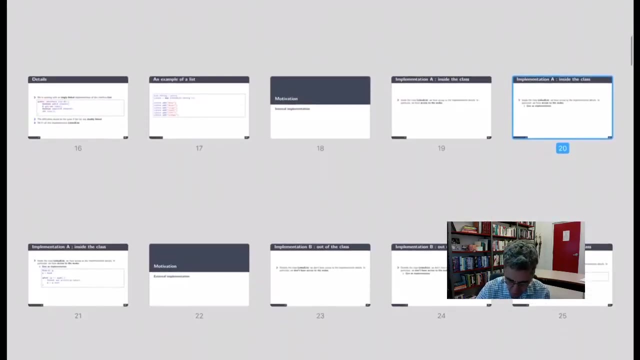 efficiency of these methods ok so we I want you to think I want you to possibly pause the video and I want you to think about which implementation is 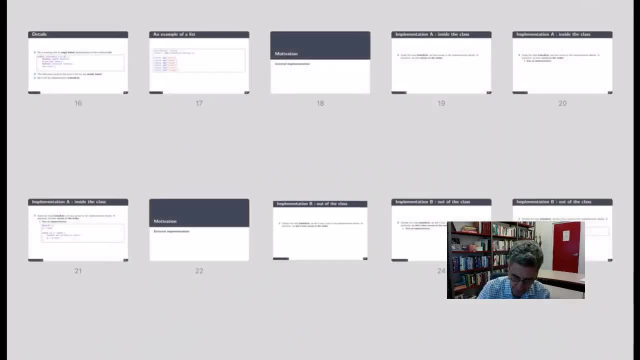 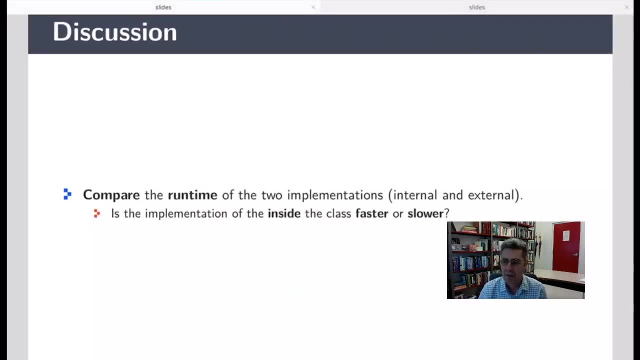 the fastest one okay so I'm currently looking at a slide for our discussion so I have an implementation where I was accessing the elements but I'm outside of the implementation and I have an implementation where I'm inside so I'm inside of my Europe and then behind this is an implementation and I'm inside 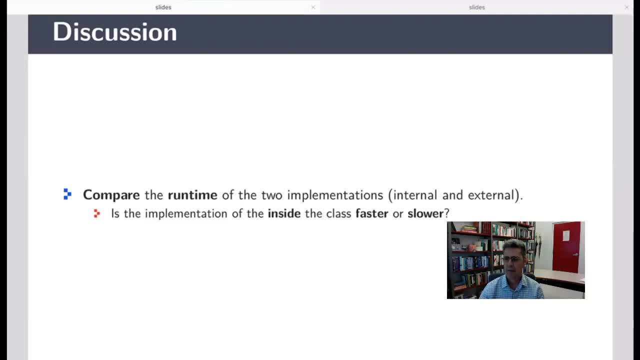 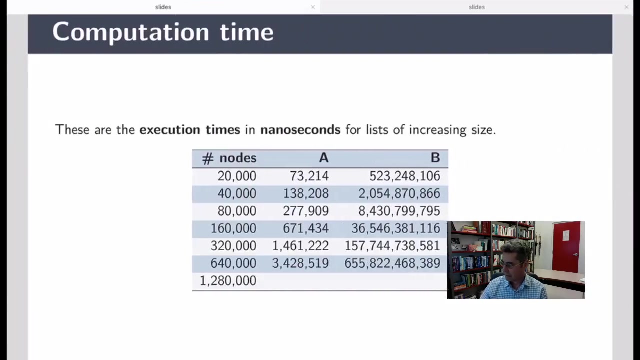 of mine this is the prevention method for this project and what we want to know is the task step one is actually faster than the other is one significantly faster than the other and what we want to know is is there one that is faster than the other is one significantly faster than the other and if so what's the reason behind us we're going to truly understand what's the reason behind this here this is run time for some tests that I did so here the execution time is in nanoseconds what I'm calling 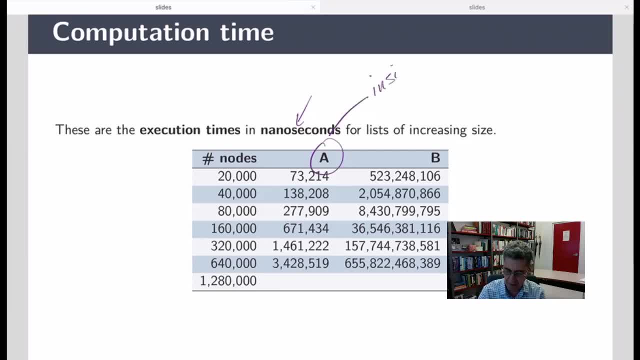 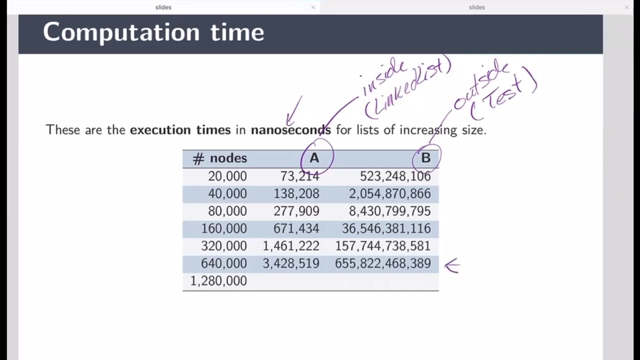 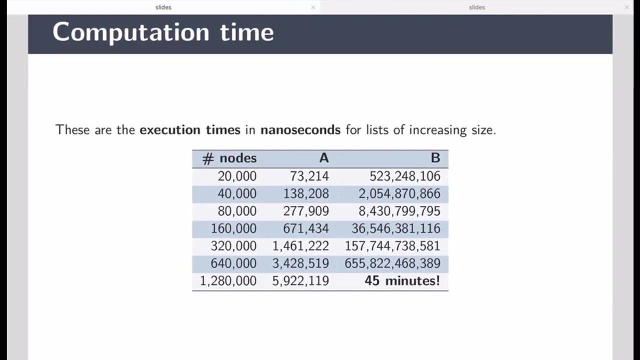 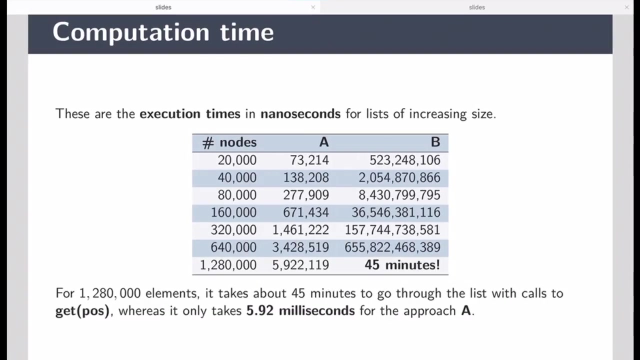 a is inside what I'm calling B it's outside this is the one that was written in the class test this is the implementation that was written in the class linked list itself okay so you you already you should appreciate that the differences is actually quite significant and we are we want to know we want to understand why this is the case okay if I move forward a little bit you're gonna see that when we reach one million two hundred and eighty thousand nodes the implementation inside the list takes five point nine two milliseconds whereas the approach when where we are outside takes 45 minutes okay so here this is in test versus linked list as I said pause the video if you need make sure that you have a good go at finding by yourself the reason for this absolutely huge difference here think about this we're implementing some game the list contains several polygons that are rendering the scene and in one case we are able to do this operation in five point nine two milliseconds so it should be almost instantaneous in the other case forty five minutes we would not sell any copy of that game that that's a failure so what I'm interested in is that is actually a mathematical relationship I want you to tell me the time that it takes for this 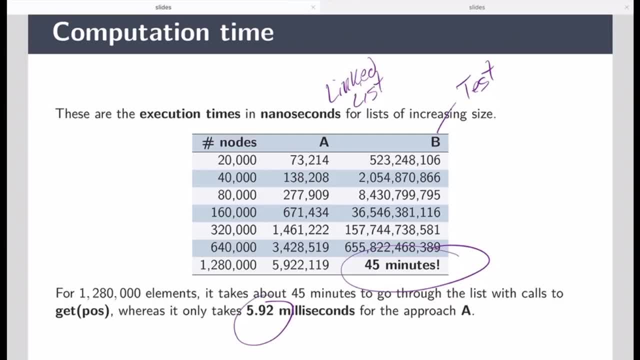 implementation varies in the following way let me show you how I created my um my my example here 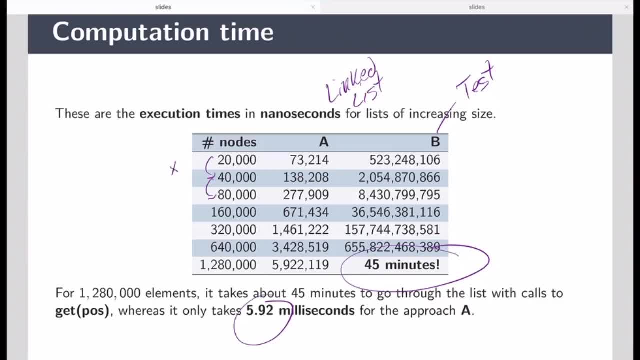 every time I am multiplying by two the size of this list 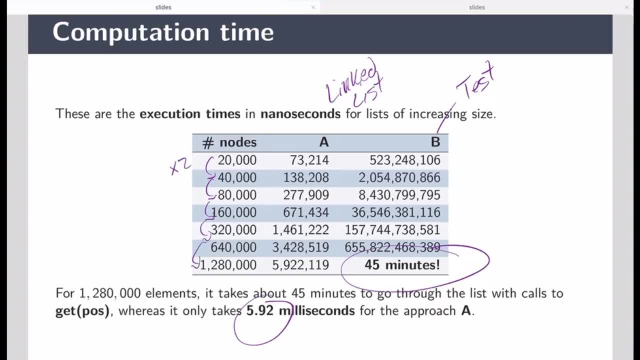 and as you can see for the implementation inside the time is more or less doubling as well 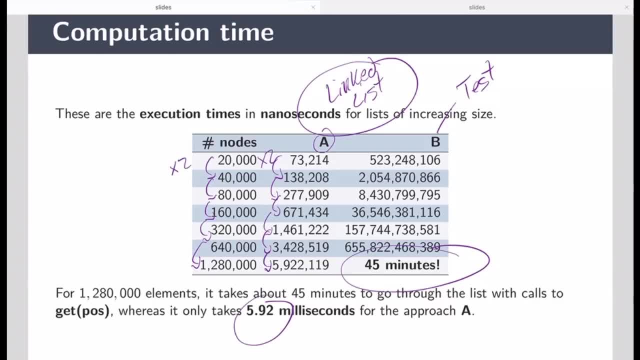 which is optimal every time I'm making the list twice as big the time that it takes to traverse the list is twice as long however if you look at 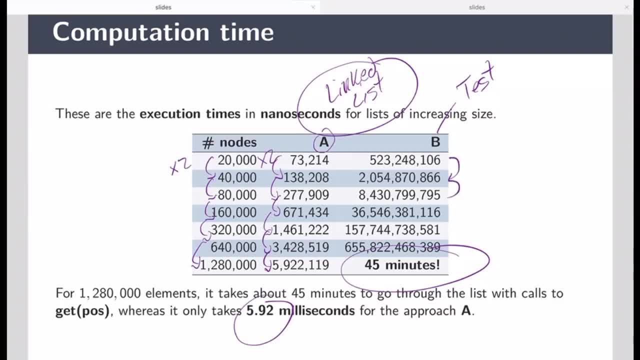 implementation B you will see that the time is actually multiplied by four each 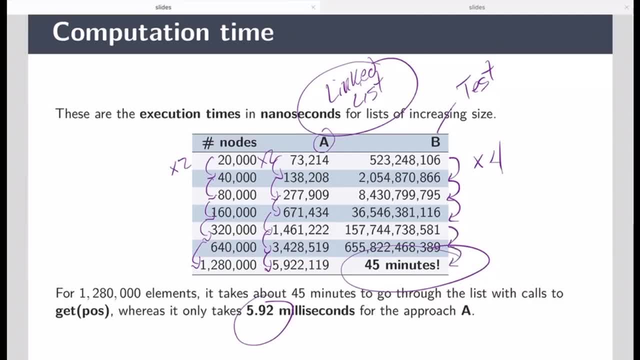 time do you see why can you think of an explanation for this for sure the implementation outside is required to make calls to the method get 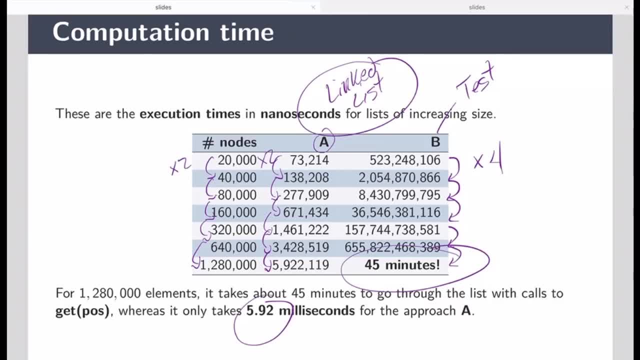 let's forget about its implementation for a second if it was only the overhead created by making a method call I would expect that this overhead would be visible. 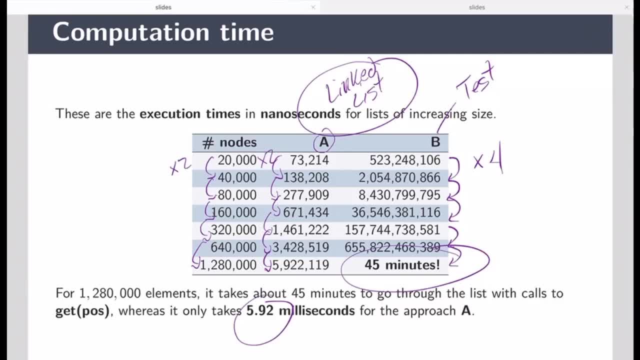 very small actually the solution that I will provide you in a few minutes will actually make several method calls from outside but it will be as fast as the one inside almost as fast 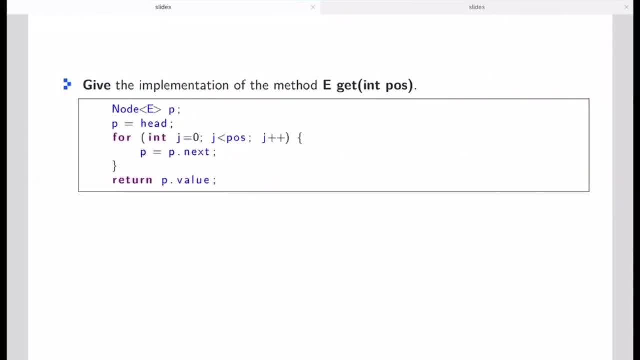 let me show you the following ok so you will remember that the method get has the following implementation every time there is a call to get P is positioned to head and 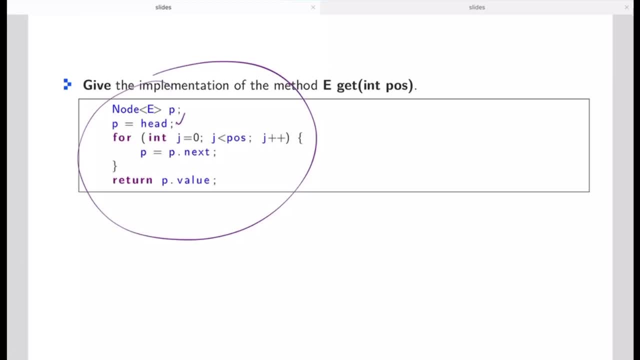 here in the slides I'm reminding you that I'm using a singly linked implementation and it has no dummy node so here I'm going to go inside this for loop a number of time which is proportional to the argument 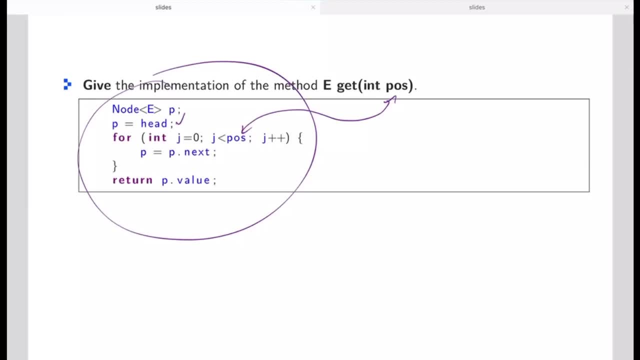 so if there is a call to get of 0 I don't go into the loop P was already pointing at head and returning P dot value if the call was for get of one P equals head we go inside the loop one time equals P dot next we return P dot value we visited two nodes if this is a call for get of get of one get of two 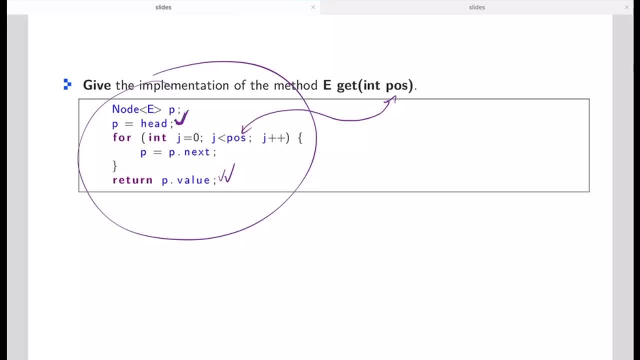 we position p on head we will go twice inside the loop and we return p.value we visited three nodes 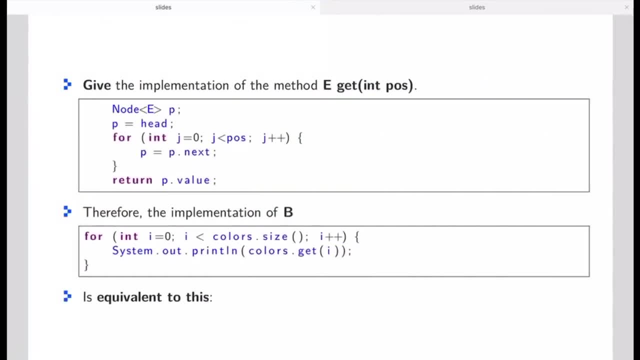 but here this get is called for every 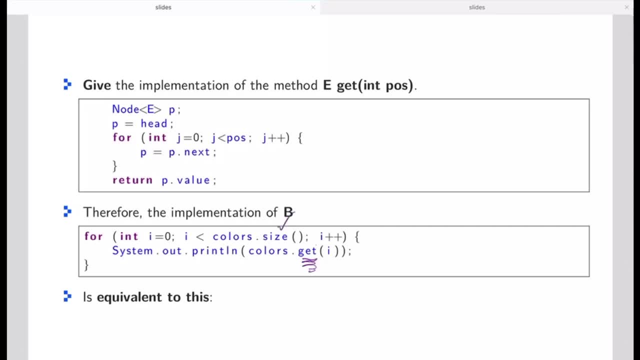 iteration of our for loop inside the method traverse inside the class test 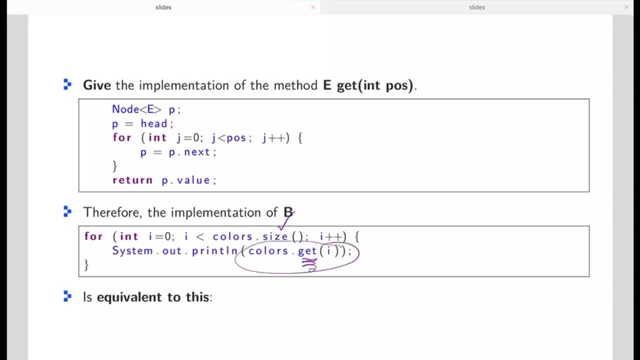 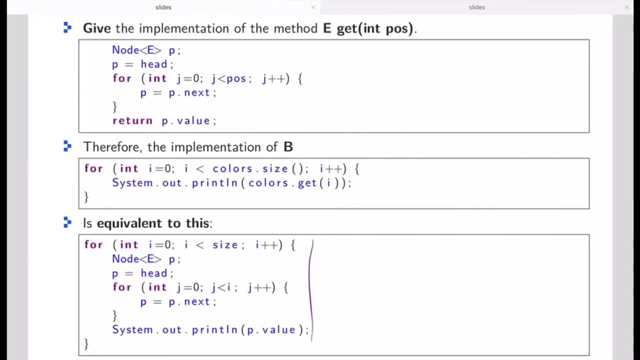 if we actually replace get by its implementation it means that the work that we're doing is equivalent to this for i equals 0 to size 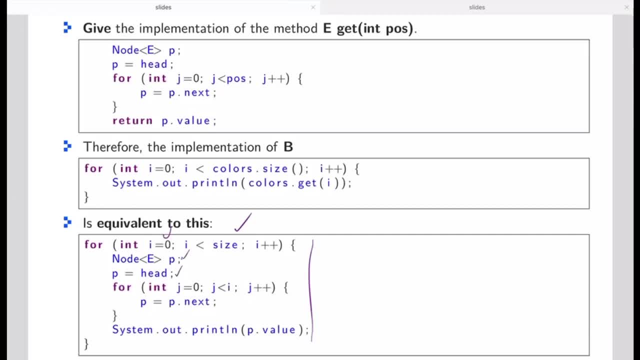 position p to head go inside the loop 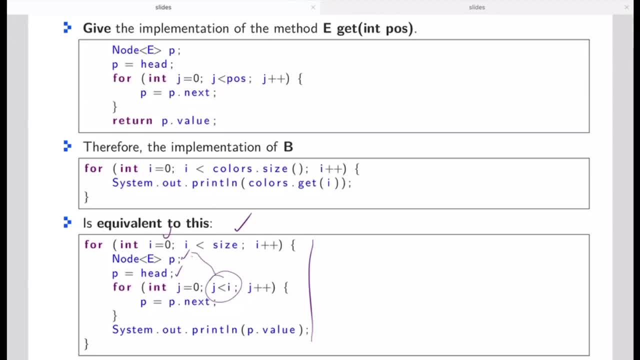 a number of iterations proportional to where we are right now, i and move 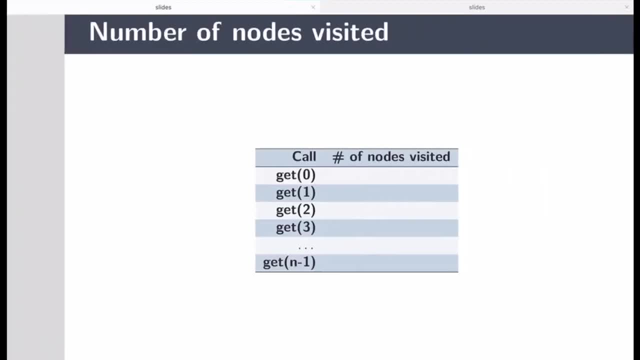 each time printing the value this means that a call to 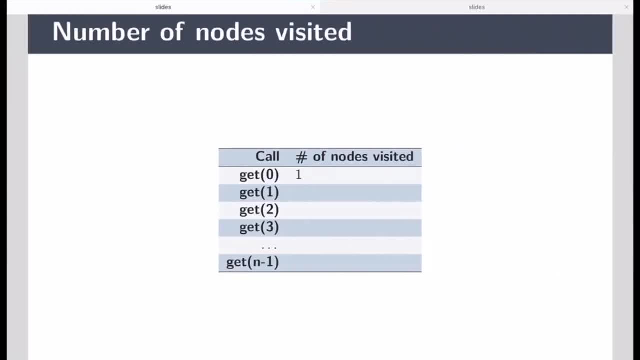 get of 0 requires visiting one node of the list 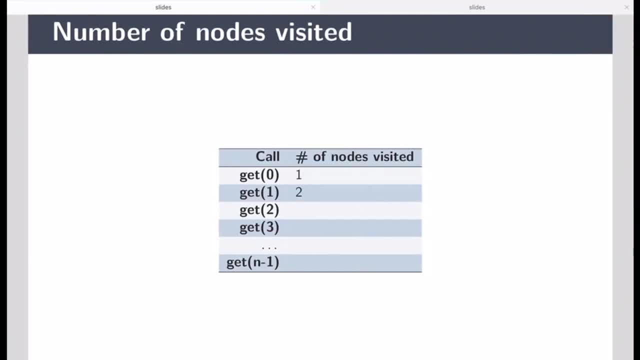 a call to get of 1 requires visiting two nodes of the list 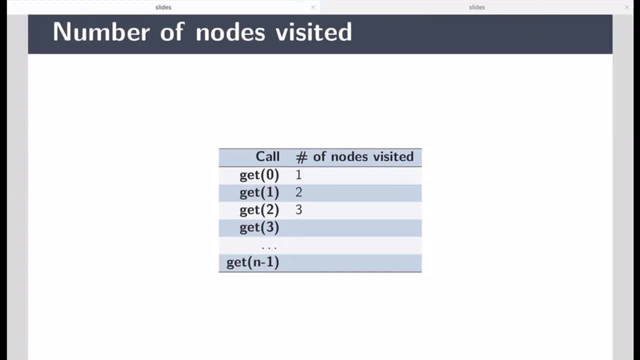 a call to get of 2 requires visiting three nodes 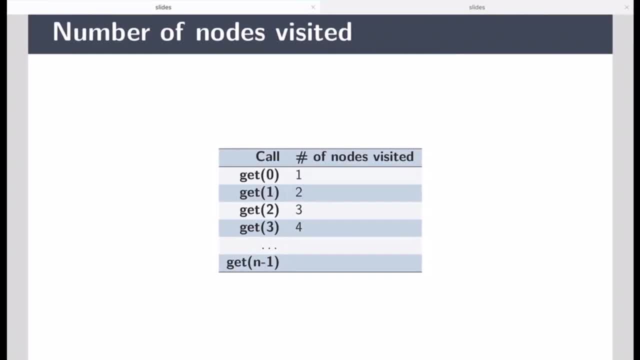 of the list a call to get of 3 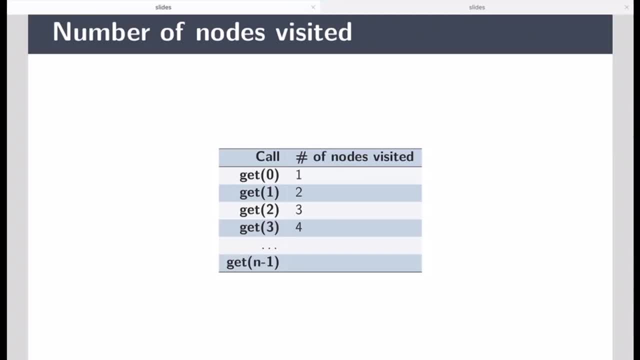 requires visiting four nodes in the general case a call to get of n-1 requires visiting n nodes 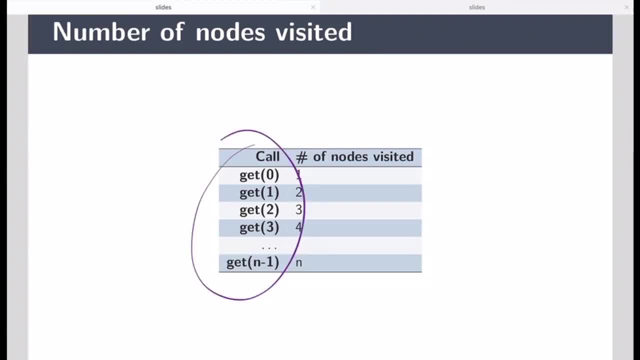 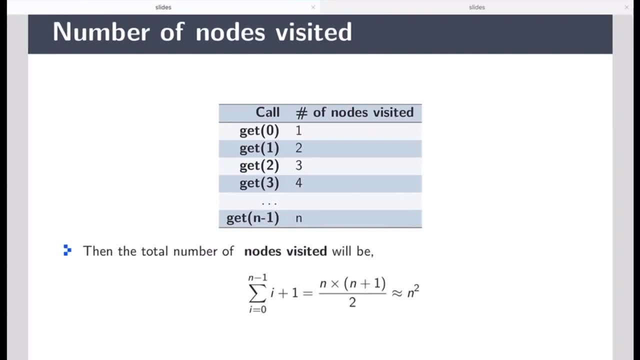 but we have made all these calls so the total number of nodes visited is the sum of all these numbers so therefore, it's n x n1 over 2 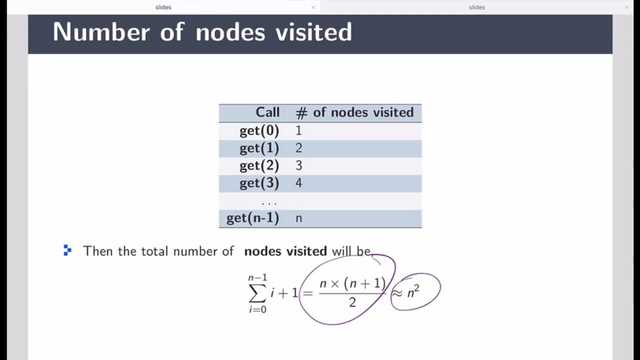 Nodes were visited. This is proportional to N square and it explains the behavior. Every time we multiply by 2 the value of N, the time that it takes is multiplied by 4. 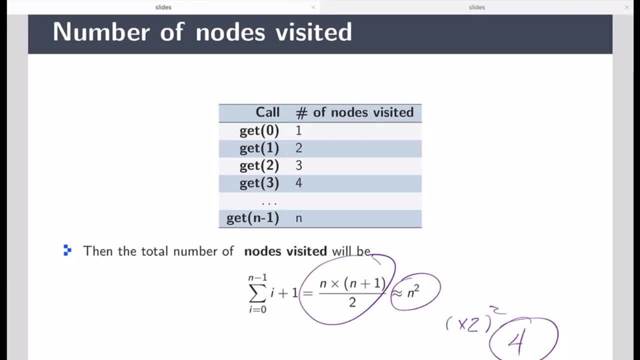 Okay, so that explains very well the observed behavior. 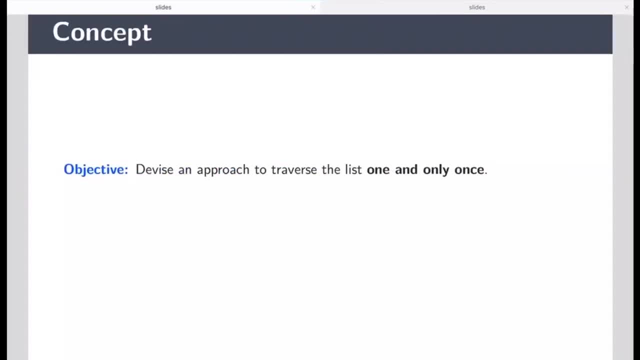 So we need a way out. We need a way to solve this problem. We want to be able to traverse the list from outside and we want to do it fast. 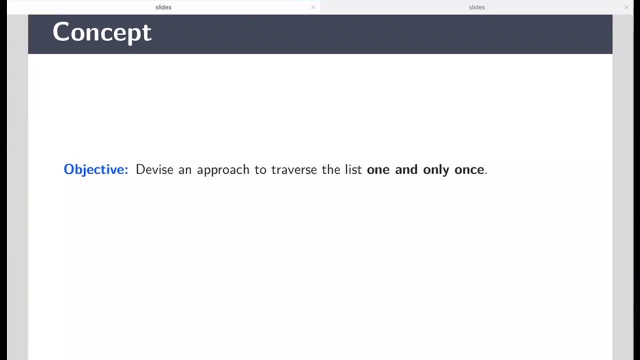 So the problem that we will be solving is as following. We want to create a method. Or a mechanism to traverse the list, meaning visiting each and every element one by one in order when we are outside of this list. Of course, the user does not have access to the nodes. We will not make any compromise on encapsulation. And it has to be clear that the mechanism that we will be providing is very specific. It's a mechanism that will allow us to visit all the nodes sequentially. This is by no means a general solution for speeding up get. It really is a way to traverse the list. So what is it? 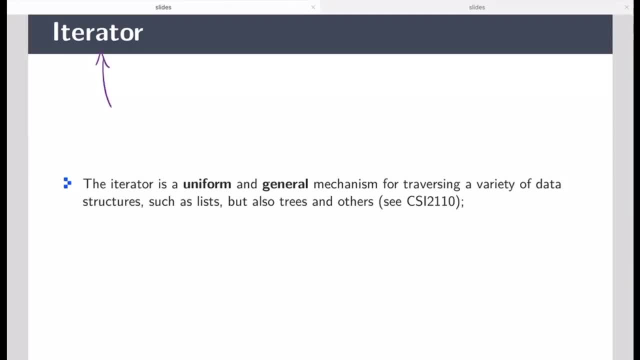 This concept will be called an iterative. This concept will be called an iterative. This concept will be called an iterative. 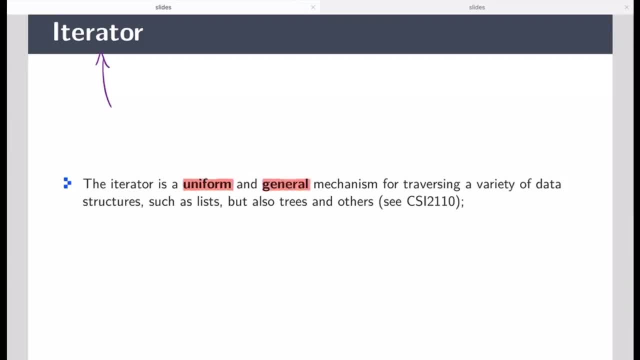 And it's uniform in general. Uniform. 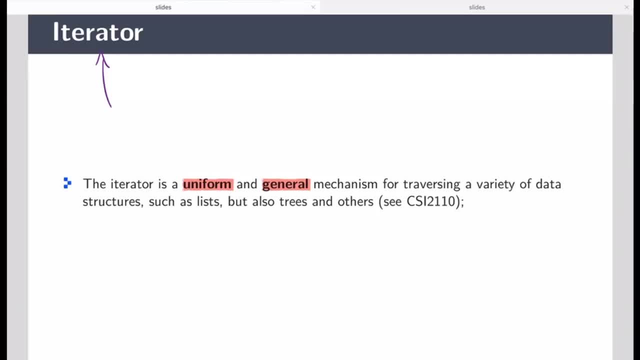 So it's the same mechanism will be applied for all the data structures that are present in the collection of Java. So this is true for the list, but also the trees and all these other data structure that you will see inside the in the data structure course. So this is true for the list, but also the trees and all these other data structure that you will see inside the in the data structure course. 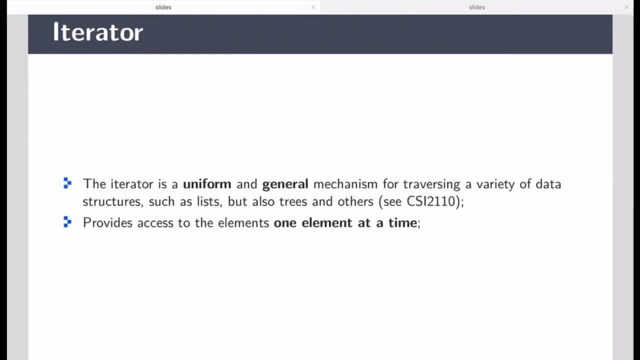 But it's a mechanism that visits the element one at a time. But it's a mechanism that visits the element one at a time. Very important. 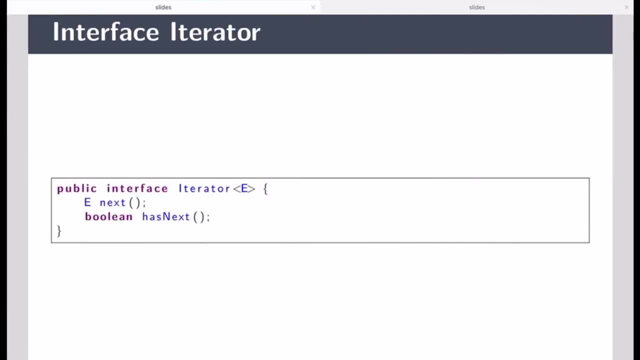 What's an iterative? An iterative 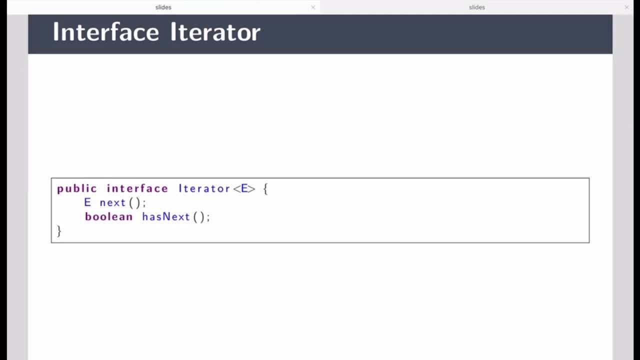 is an object that has a method next and as next 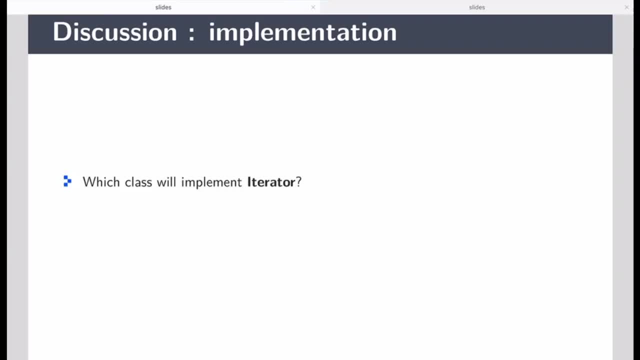 Now the important question is Who will be responsible for implementing the iterative? 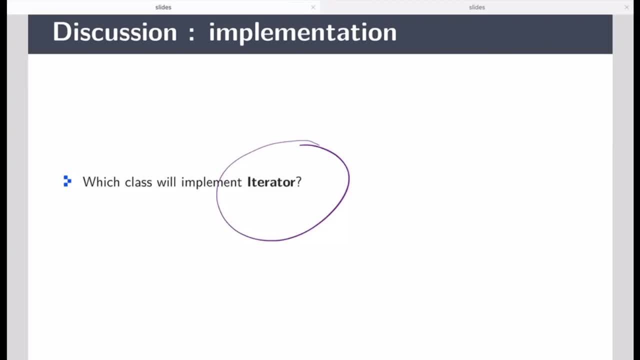 Who will be responsible for implementing the iterative? iterator that's the first question that we need to answer let me show you what i mean what i'm 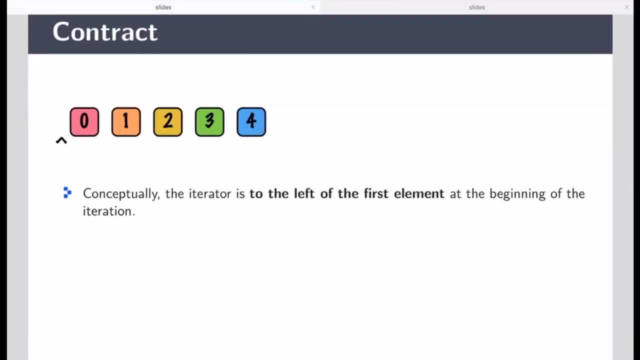 expecting what the behavior should be for this iterator if i have a list and it contains these five elements zero one two three four what we want is that conceptually the iterator is before 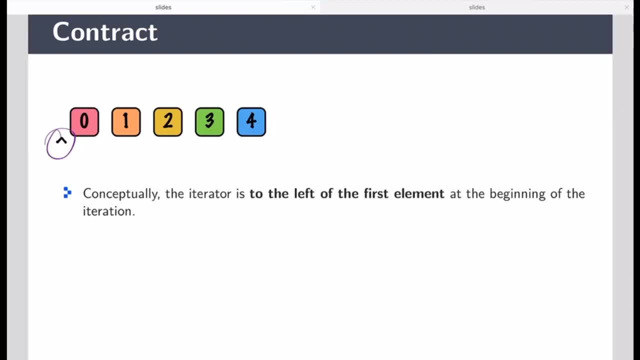 the first element we're at the start of an iteration we have not started an iteration yet and now there will be a call to the method next the iterator has moved over the first element and it has returned the value of the first element that's conceptually what we're going to do is we're going to call the method next and we're going to call the method 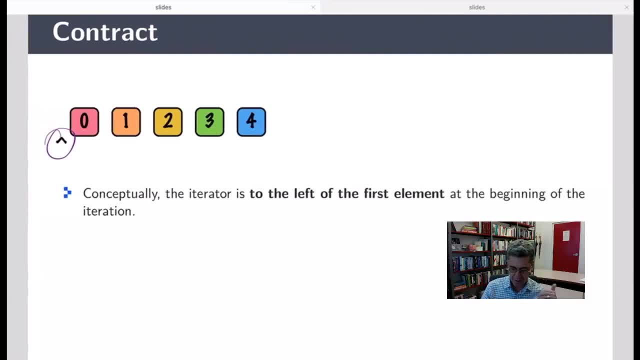 we're expecting before the iterator is at the start of the list we call next it returns one 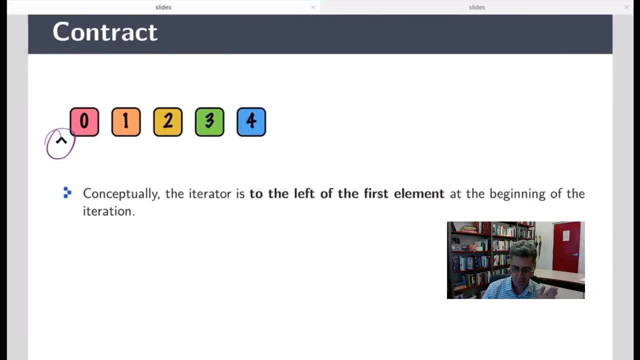 and it has moved past it returns zero sorry it returns zero and it has moved over the element if there's a new call to get to next 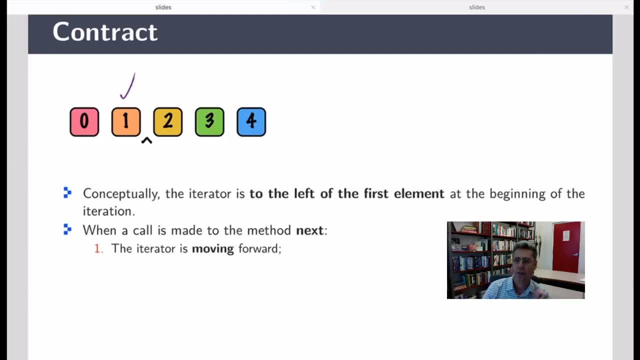 it returns one and it has moved over the first element it's positioned in between the next two call to next it returns two and the iterator is positioned after another call to next it returns three it's positioned before the last one if we call the method has next it should be returning us 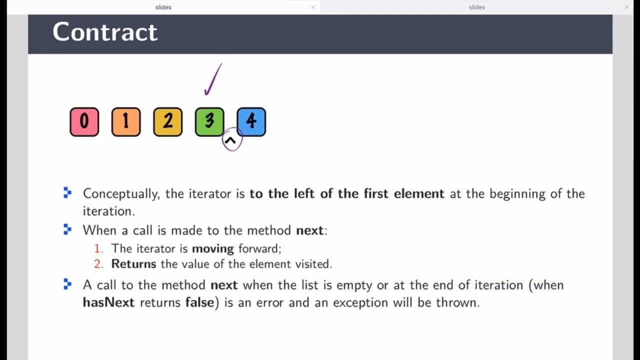 true because we're not done with the iteration the iterator can still be called we call the method next it returns the value four the iterator is now positioned after the list if we were to call the method has next it will return false because it would be an error to return a value we are done with this iteration 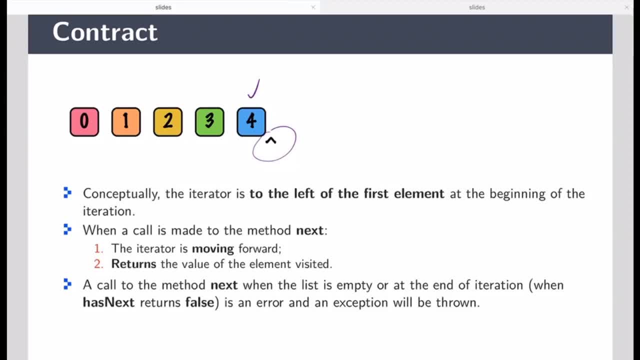 okay so that that's the expected behavior 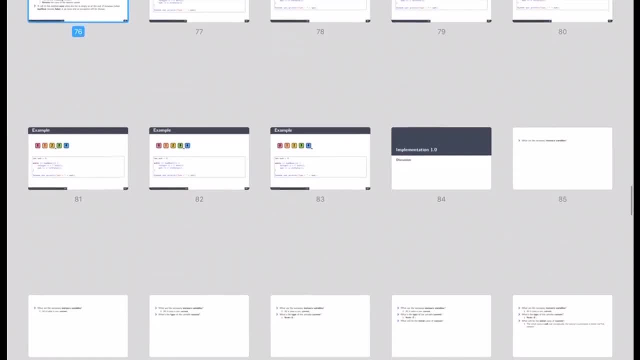 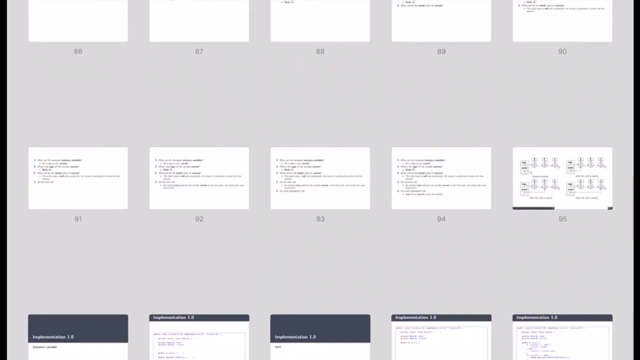 i'm going to propose you a first implementation that we will actually throw away very rapidly but still it's going to be a stepping stone it will allow us to understand the concept 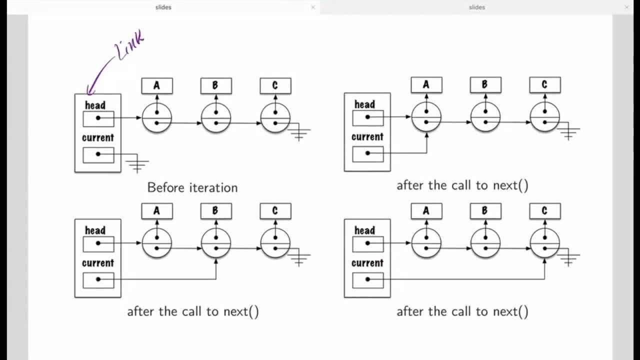 here this is the object of the class linked list has a variable head and i decided to give the responsibility of implementing the 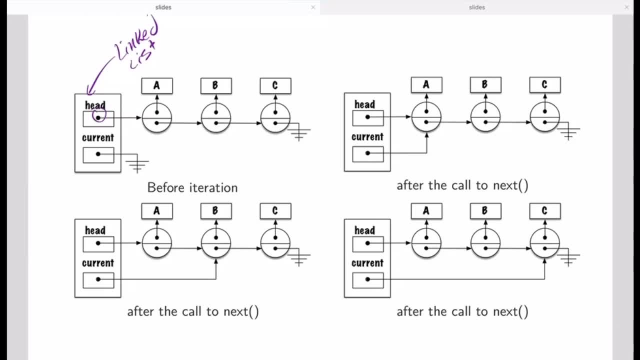 interface iterator to the list itself so i'm adding an instance variable to the linked list so its state now allows it to keep a bookmark on the list it's now able to 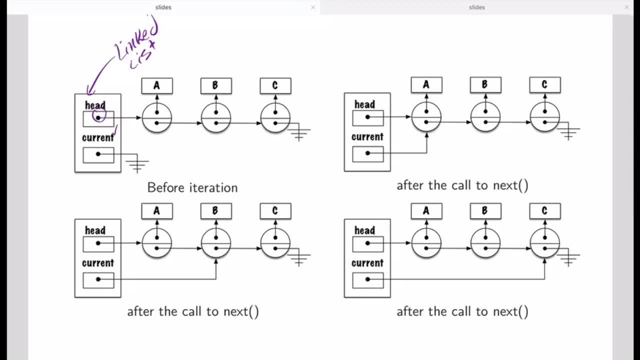 remember what was the last value that was returned by a call to next i really look at the iterator as some kind of bookmark you ask the iterator are there more elements in the iteration yes there are more element give me the next one 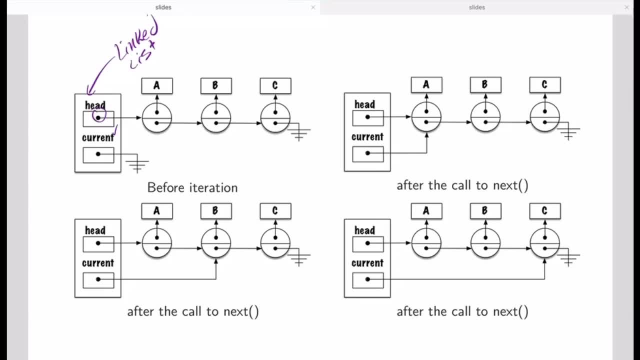 it's returning you the next element in the iteration and then it memorizes where it's at in the iteration so for the implementation in the slides 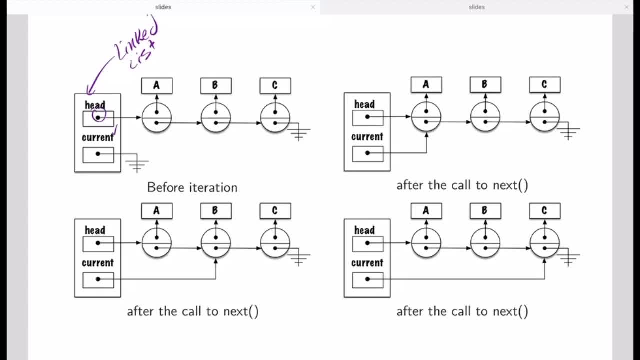 i have a singly linked list with only only a head pointer and my strategy is current equals null current equals null means i'm before the first element i have not started an iteration 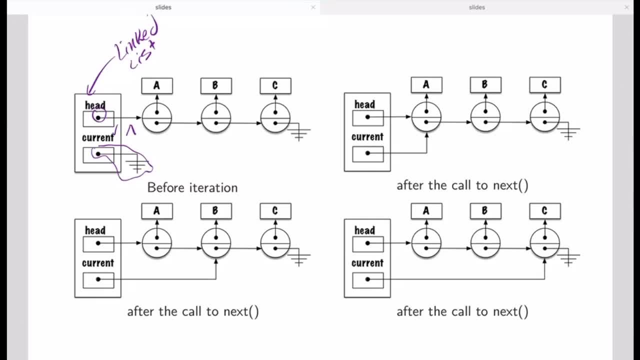 calling the method next the iterator will say okay i need to start this iteration i will copy the value of head in my instance variable current i will return current dot value so it returns a and conceptually the idea is that the iterator is now positioned after a conceptually 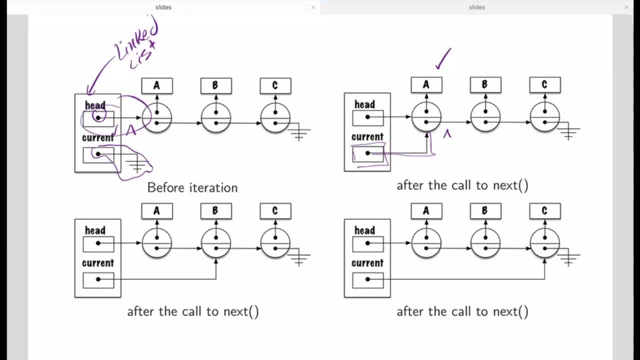 if we ask the method has next can i call the method next is would there be more elements in the iteration it will say yes here we call the method next here current is not null i'm already in an iteration let's copy current dot next in current as a result of that current is now pointing at the next element we return current dot value this is b the iterator is now positioned conceptually after the first element now 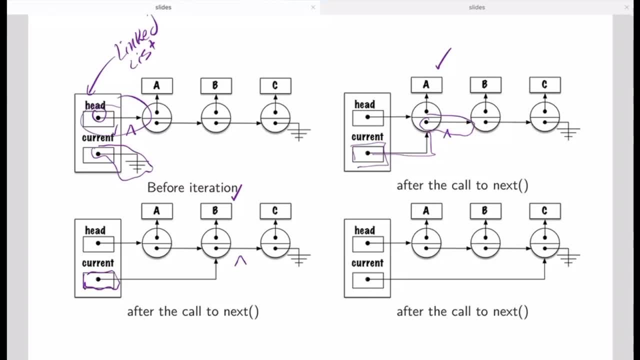 if we ask the method has next are there more elements inside this iteration it's going to say yes we call the method next again it copies current dot next into current as a result of that current points here we return curt dot value conceptually the iterator is after 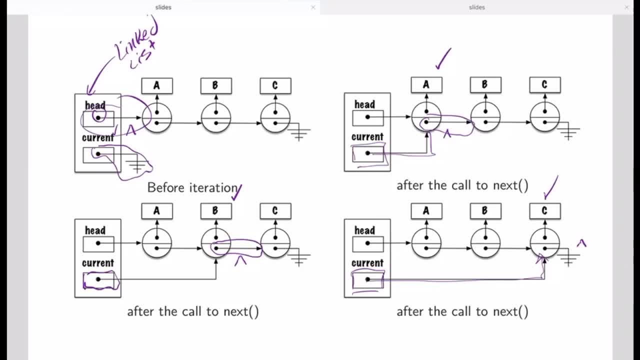 if we ask the method has next are there more elements it's going to say no this time it's going to return false 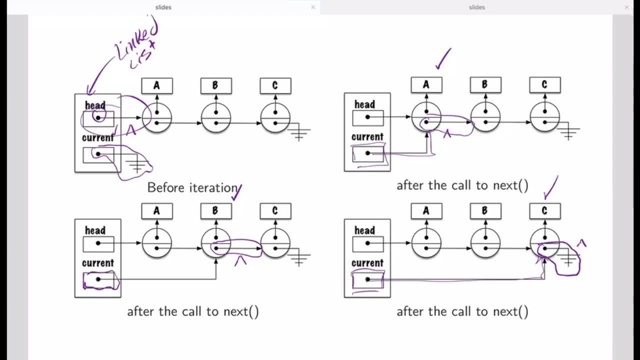 that's because current dot next is null and you clearly see that it would cause an error to call the method next again because what we would do is current equals current dot next as a result of that current would be null so we would return the method as null if we were to return current dot value we would get a null pointer exception okay so that's what i'm proposing as a solution 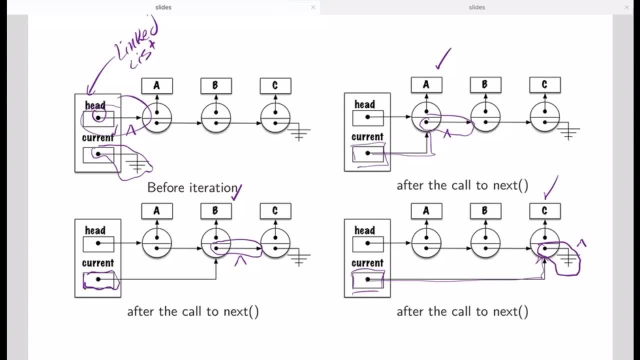 it's not going to be our final solution but it's going to work and it's going to be fast there will be some flaws but still it's going to work and it's going to be fast now 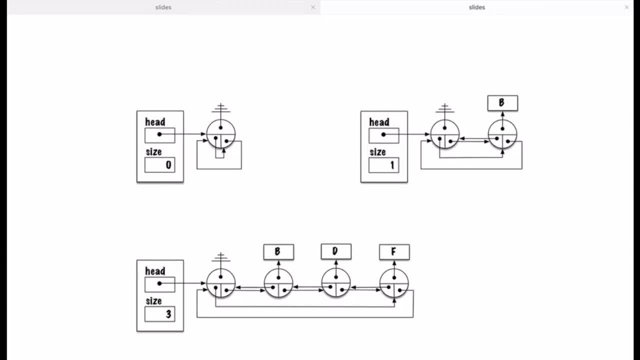 in in the implementation that we will be writing the code the list is doubly linked and circular 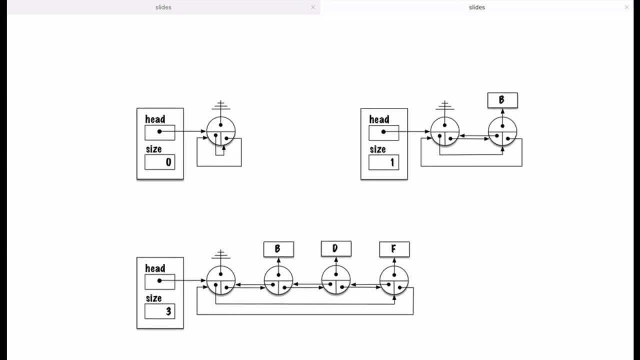 if we focus our attention at the bottom my implementation of the iterator will be very similar but with some small differences 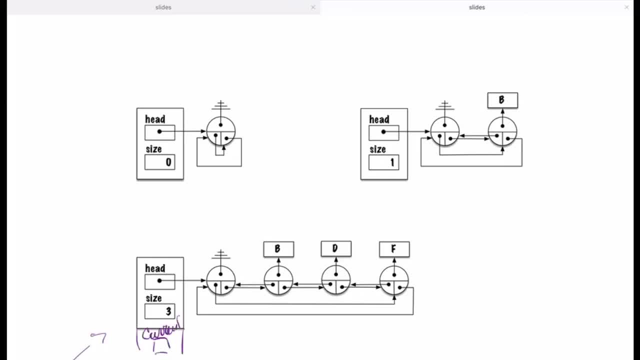 so i will still use a variable called current but because we have a dummy node i will initialize current to be pointing at the dummy node itself 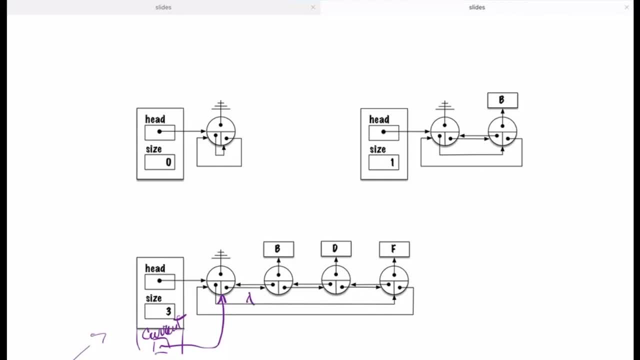 and here we will think about it as on before the first element if we call next it's going to copy current equals current equals current dot next so it's going to move the iterator here we will return current dot value so this b and the iterator is now conceptually in between these two elements there are there more elements in the iteration of course let's say current equals current dot next the iterator moves here we return current dot value if we ask the method has next are there more elements in the iteration of course so therefore we can call next it will copy current dot next in current and return current dot value if we ask the method has next are there more elements in the iteration here we want it to say no to return false because we are at the end we are at the end because because current.next is pointing at the same place as head. 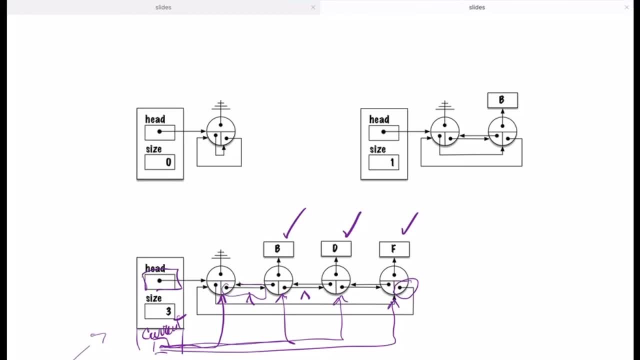 It's pointing at the dummy node. And this implementation of our iterator inside the circular list with a dummy node 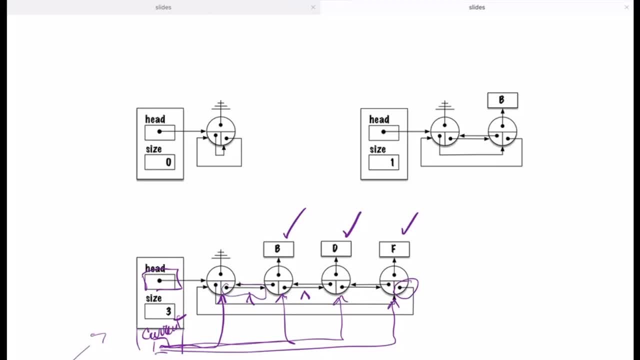 is actually easier to make than the other one. 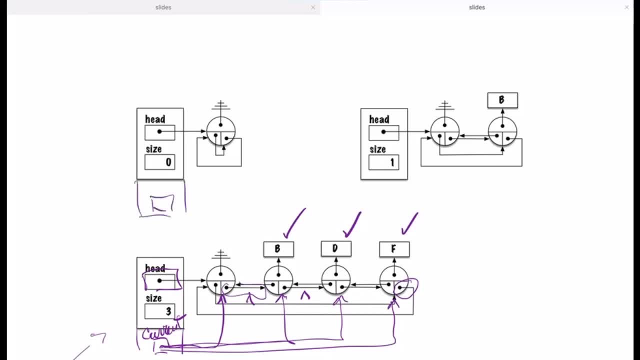 So here, and it will work all the time, in particular, when we have the empty list, current will be pointing at the dummy node. And here, if we ask the iterator, are there more elements inside the iteration? It's going to say no, because next is pointing at the dummy node, the variable next. Okay. Let's code. Let's code this thing. 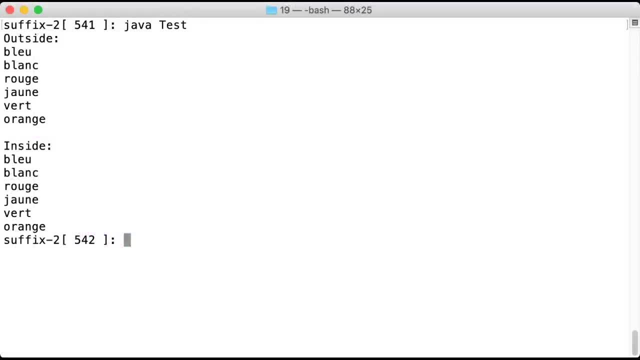 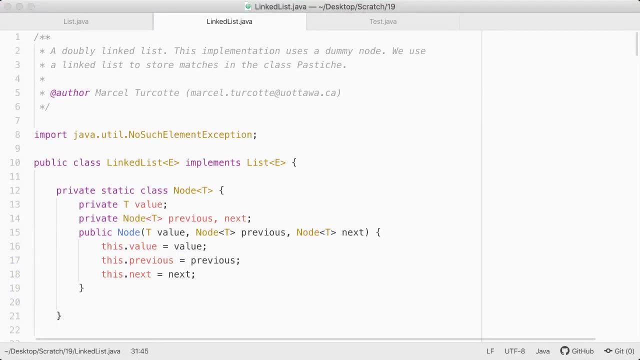 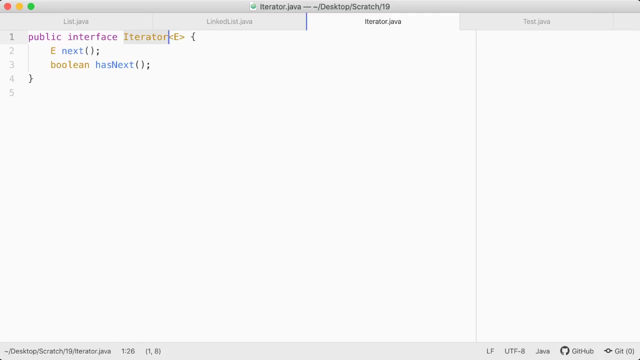 So, we actually need the interface iterator. Let's copy from 03 iterator.java here. Let me show you what iterator looks like. So, public interface iterator has a method next, returns something of type E, and has next a boolean. 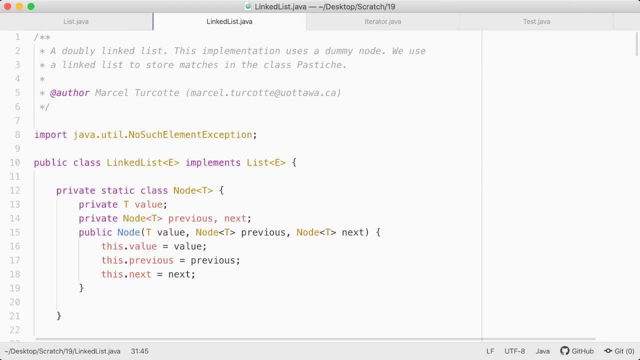 We said that for now, we're going to give the responsibility of implementing the iterator to the list itself. 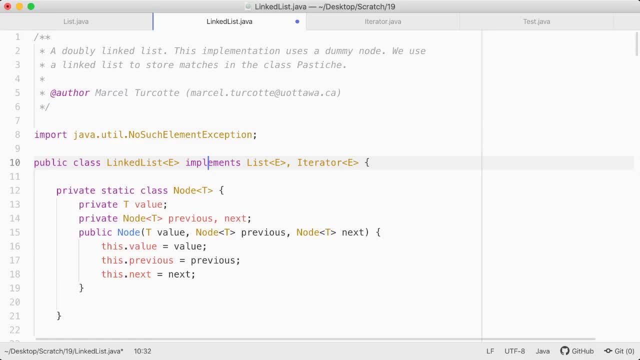 So, here, this is a good example that a class may implement, multiple iterators. Here, it says, a linked list can be seen as a list, having methods size, get, et cetera. Or, it can be seen as an iterator. It has next and has next. 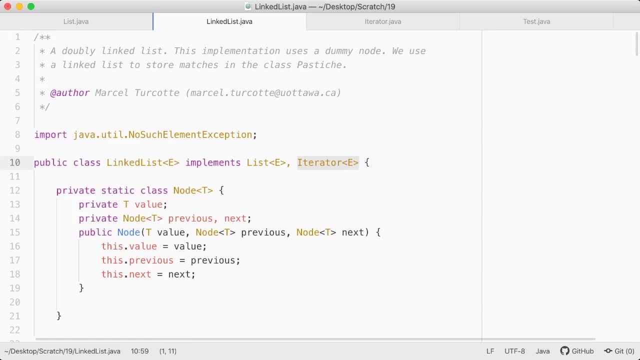 Okay. That's our first implementation. Our final implementation will be different. 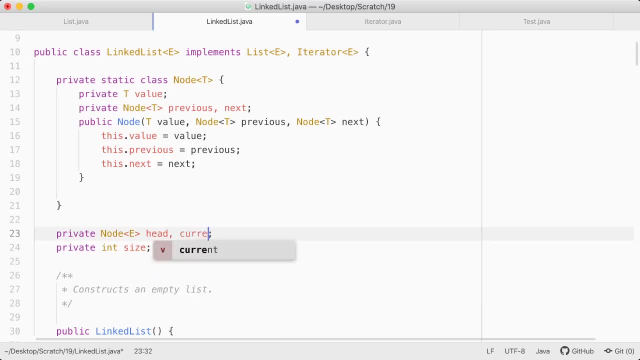 We said that, the list will have one additional instance variable 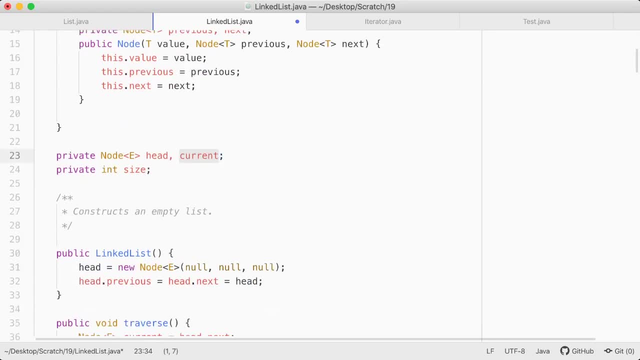 called current of type node. That's the iterator here. 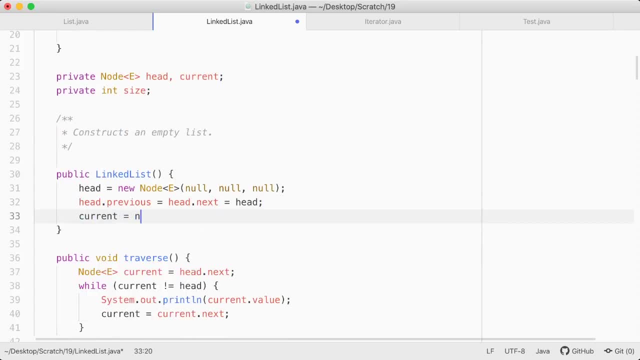 Current is initially equals to null. We are before the first node. 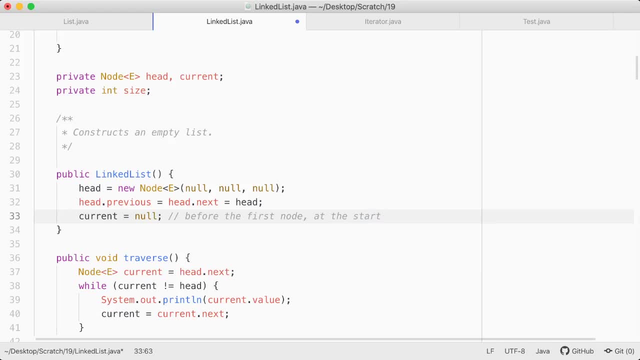 We're at the start. We're at the end of the iteration. 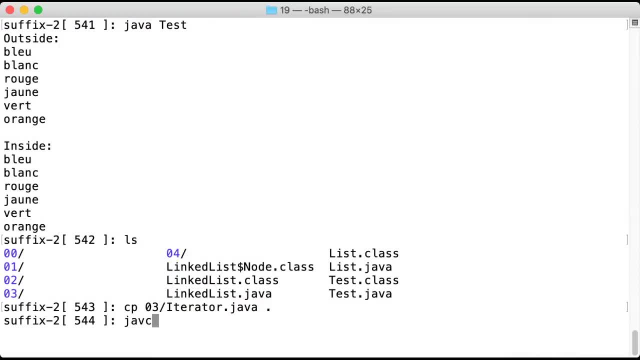 Right now, if I were to compile the list, it should tell me, no, no, no, you're not fulfilling our contract. 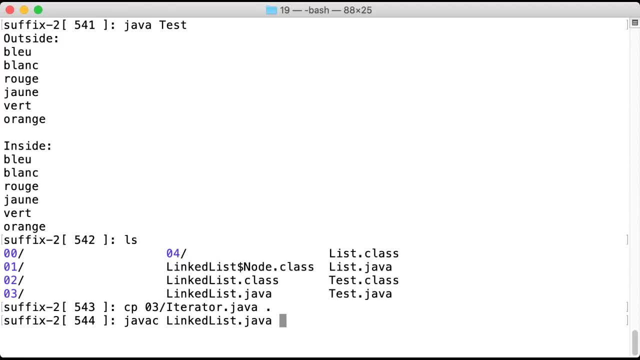 You told me that you can be seen as an iterator, and yet you're not providing an implementation for next and has next. Okay. 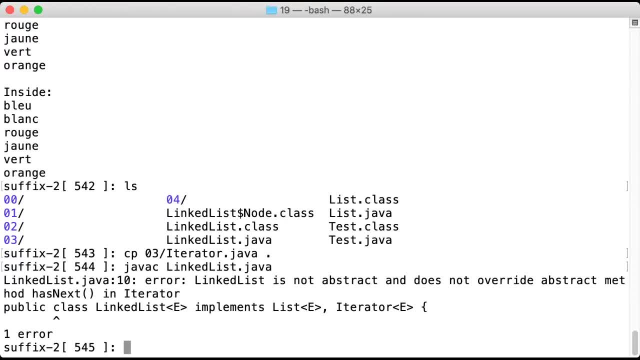 Linked list is not abstract and does not override the method has next. 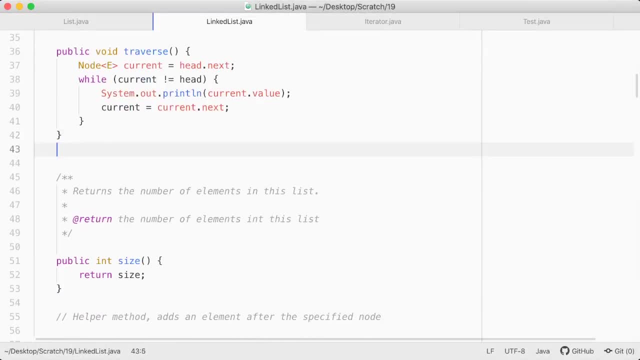 Okay. To have the list compiled, we need to make sure that we have an instance method has next, as well as a instance method private e next like this. 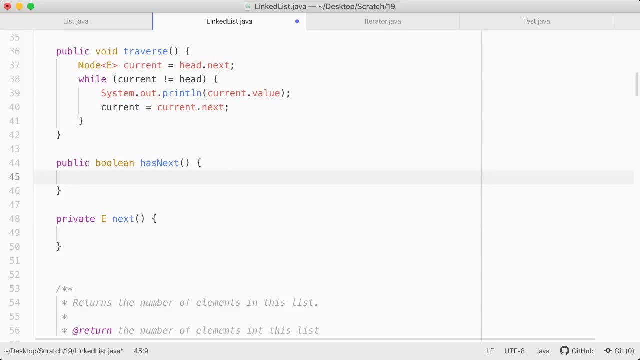 I always like to be able to compile an implementation as soon as possible. So I'm going to write throw new unsupported operation. Operation exception. Not implemented yet. I'm going to do the same thing here. Save. Compile. Error. 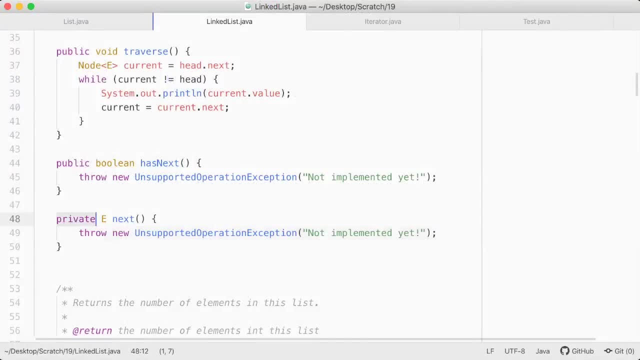 Next private. Oh, I made it private. 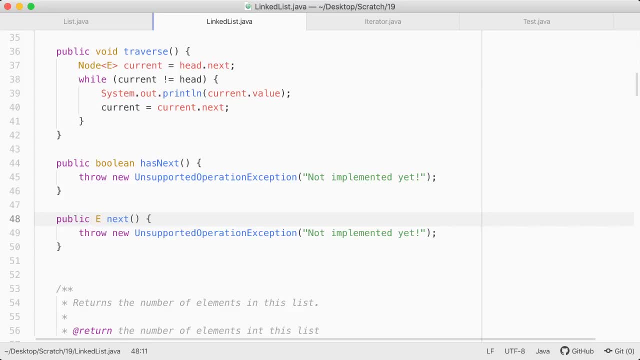 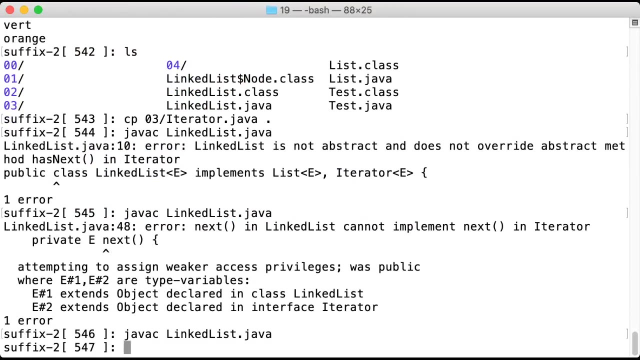 Cannot make the method less visible than what the interface says. So now it compiles. 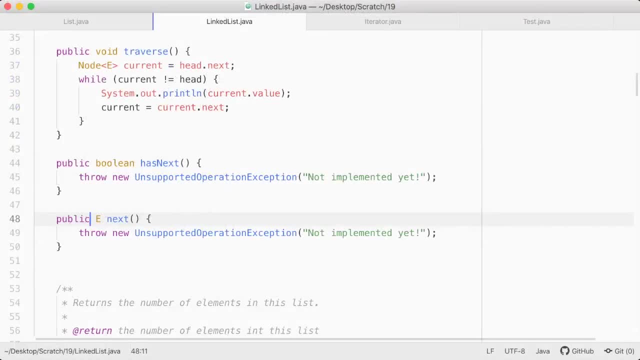 Why was it important to me that it compiles? Because I want to have the compiler on my side, helping me detecting errors as soon as possible. 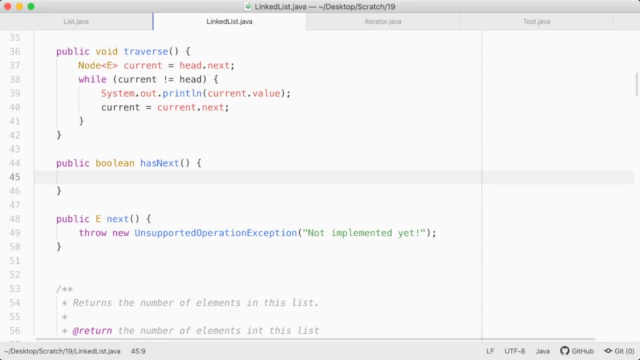 That's why I started my implementation like this. So now I know that everything that I've added to the list so far, at least from the point of view of the syntax and the types is sound. So what has next? 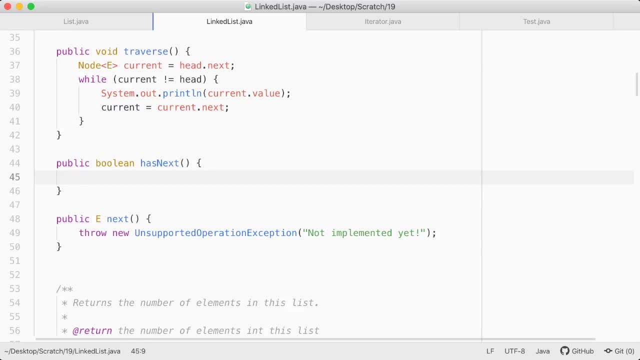 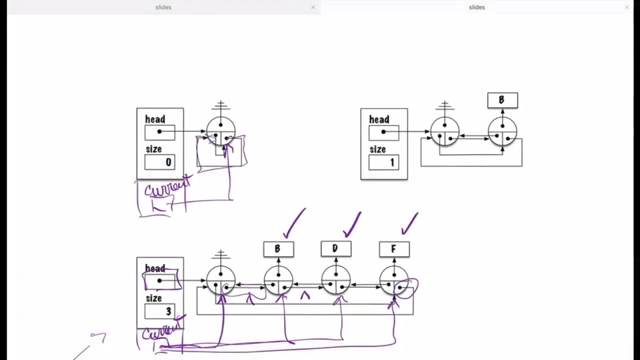 We are in the implementation where we have a dummy node. The implementation is quite simple, actually. If current.next is different than head, we can move forward. Remember, if the list was empty, then current.next would be .next. 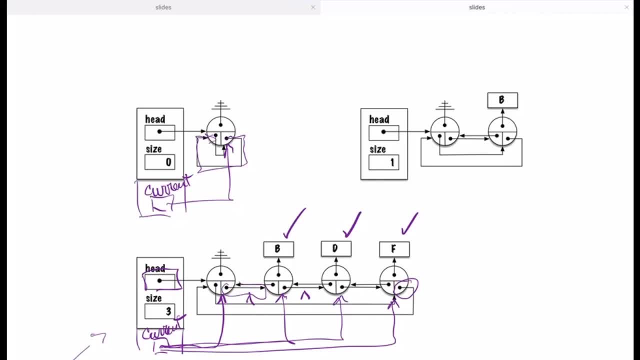 would be pointing at head. And here we would say, no, no, no, no. 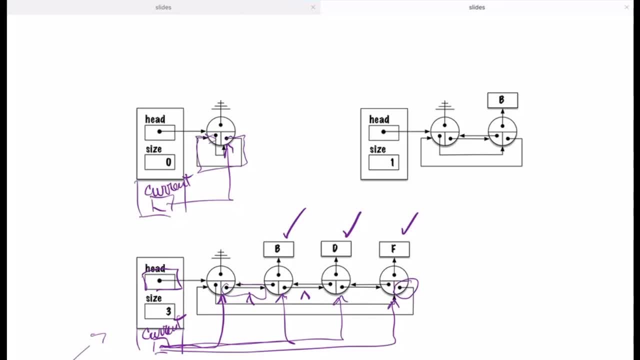 You cannot call the method next. There are no elements inside this list, so you cannot iterate. 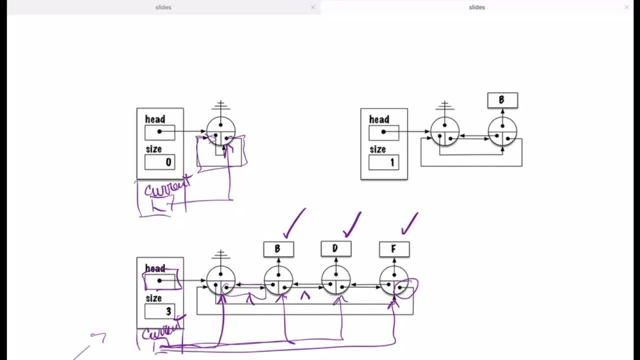 However, if there were elements, initially current is pointing at the dummy node. Current.next is not null. It's valid to move forward. 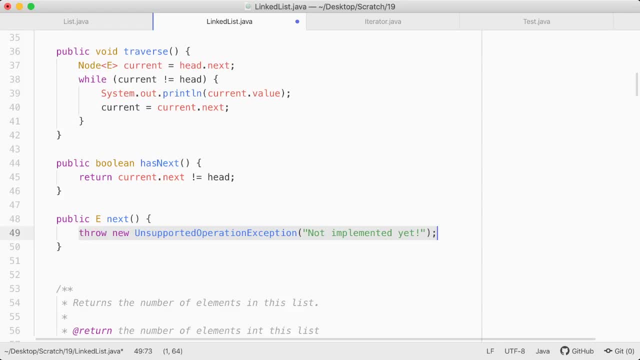 What's next? Well, we've said it. 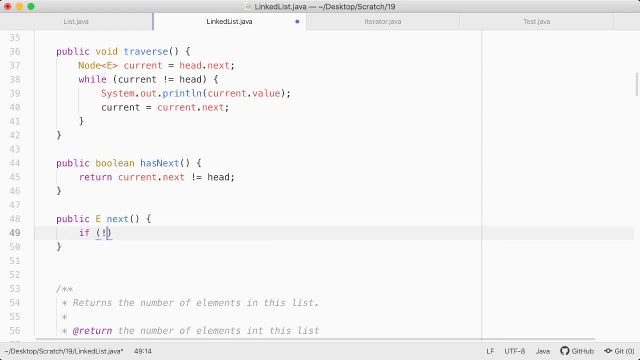 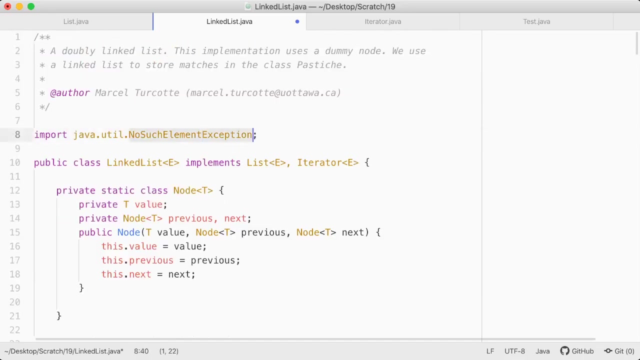 So first we have to see. If hasNext is false, if there are no next elements, throw new noSuchElementException. 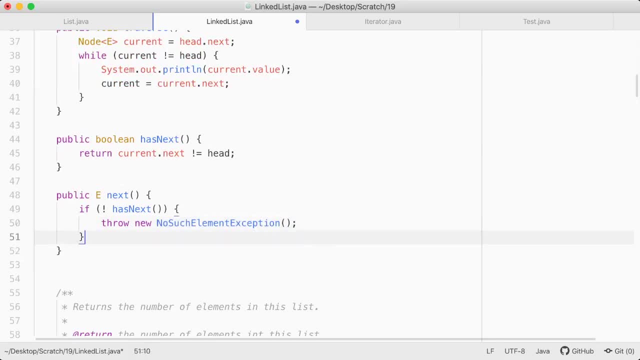 Should not call the method next if we're at the end of the iteration, if there are no elements in the list. 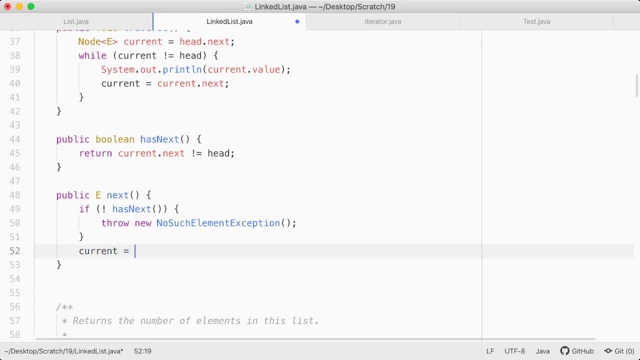 Otherwise, move forward. Current equals current.next. 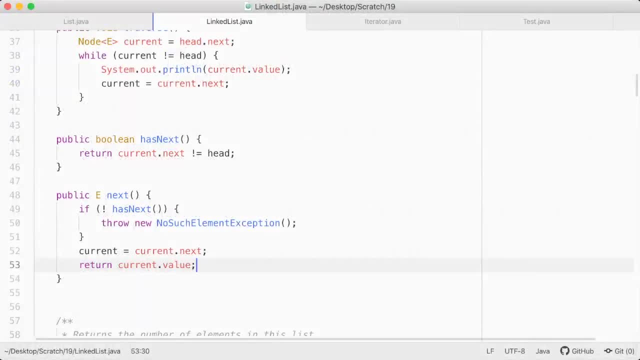 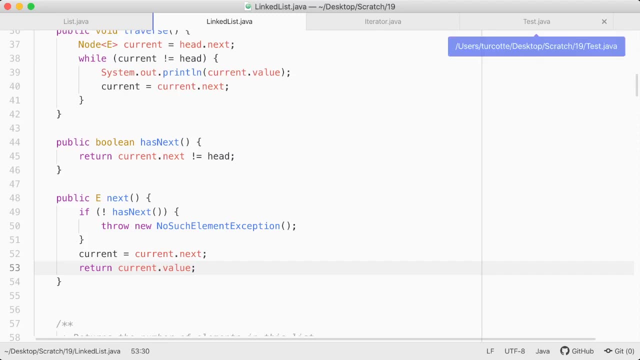 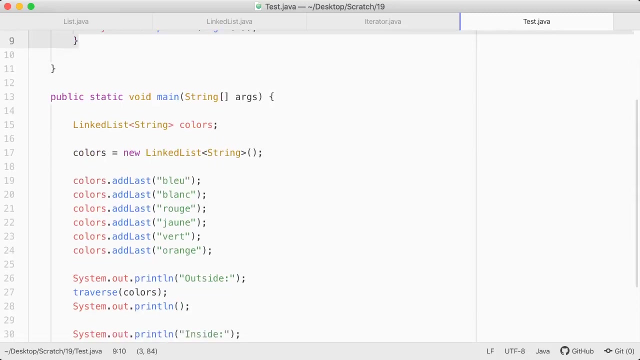 Let's see if we can use this mechanism. Let's see if we can use this mechanism. Let's see if we can use this mechanism. 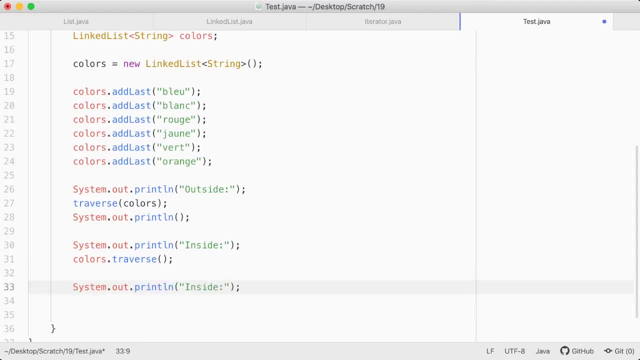 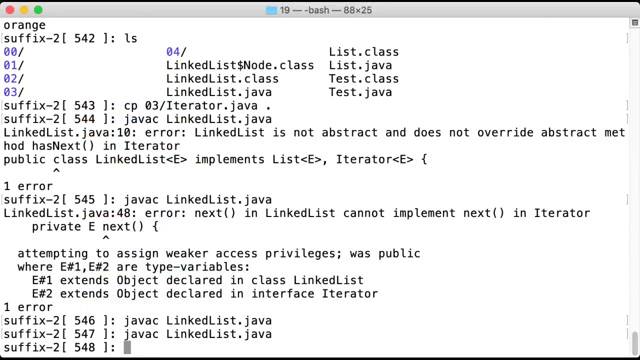 with an iterator we want this to be pretty we're gonna have a new line here here iterator for string i javac test.java 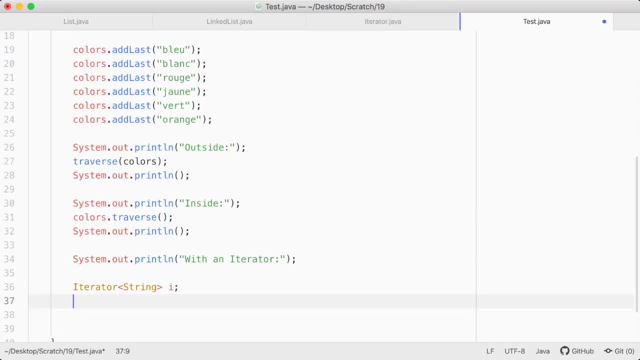 so far so good what can we store inside i the reference of an object that implements the interface iterator color does implement the interface that works while i as next 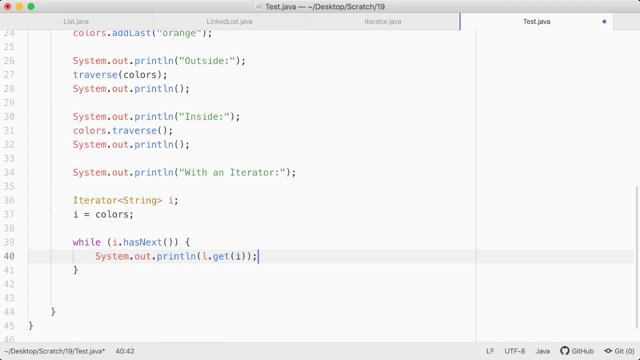 let's print i dot next 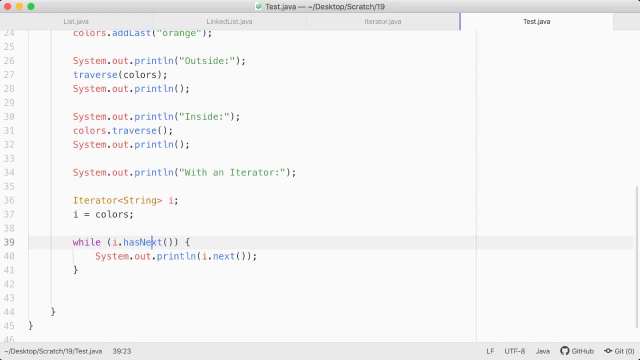 okay so i has a method as next and next 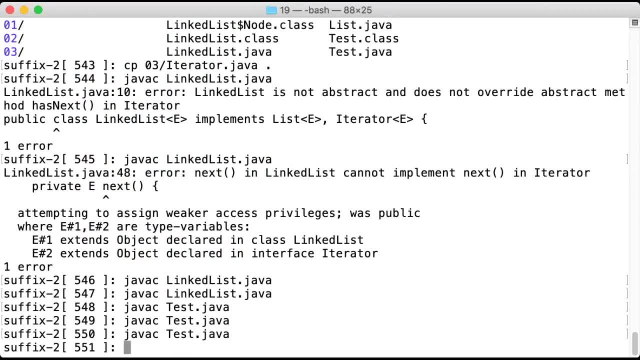 that should be okay java c and now let's run our test 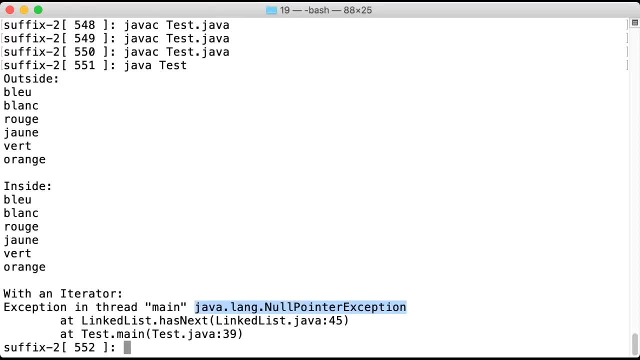 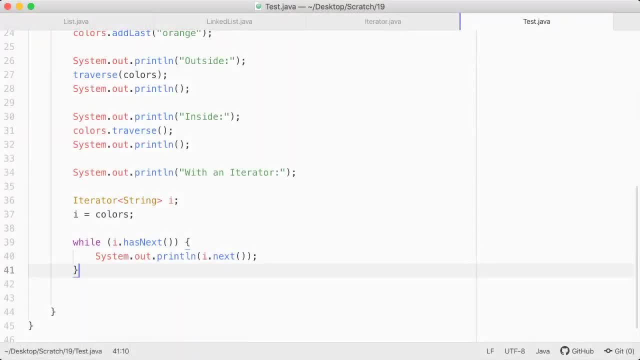 whoops null pointer exception on line 45 okay so we've done something wrong 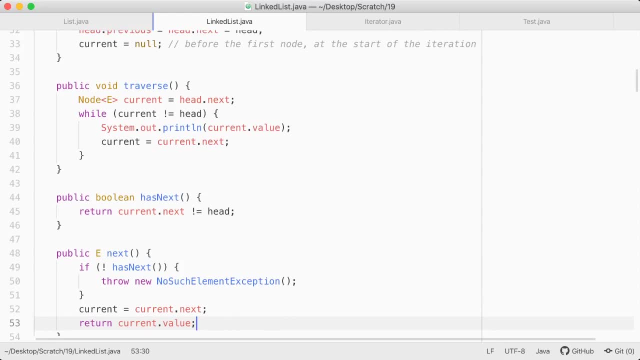 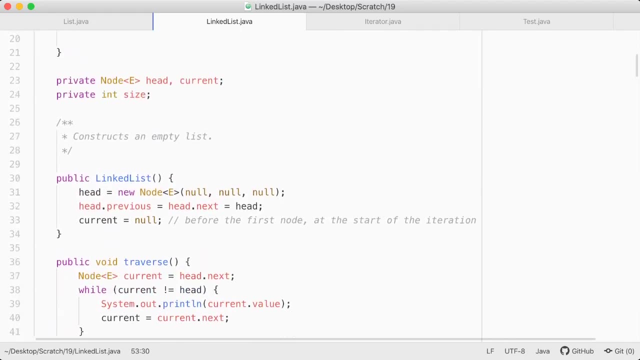 s oh oh yes oh yes i made this mistake 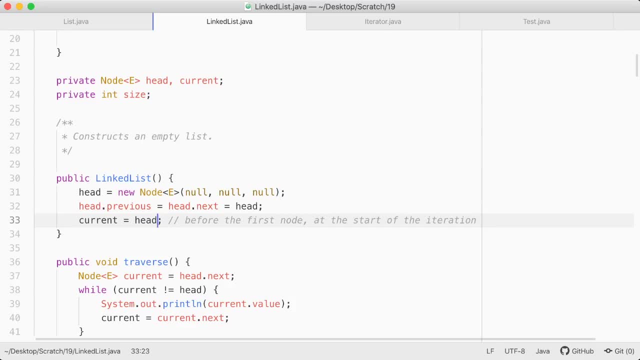 obviously it was not intended but it's a good example 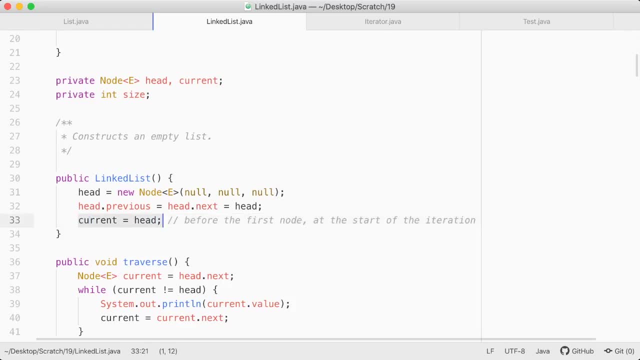 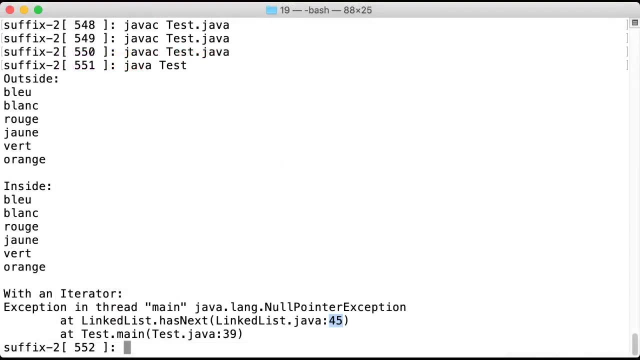 in the implementation where we have a dummy node the idea was that current would be pointing at the dummy node okay good good 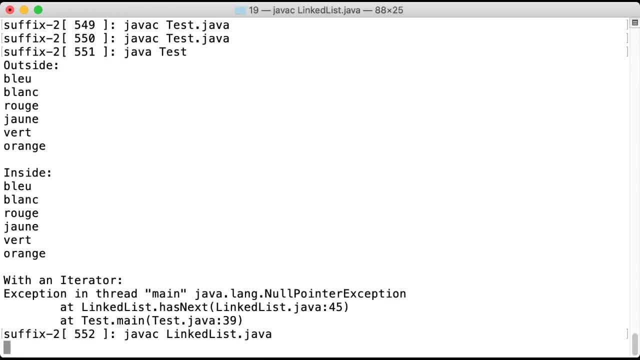 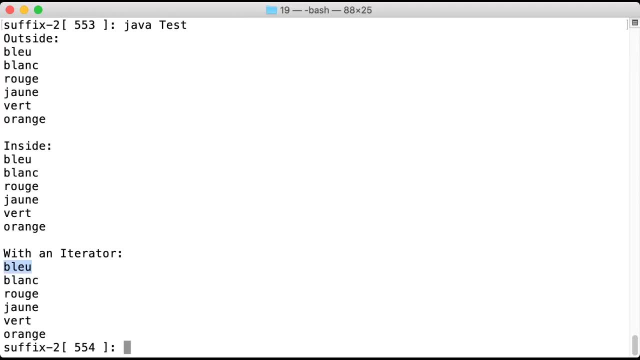 let's recompile our linked list let's recompile well no the test doesn't need with the iterator blur blonde rouge jaune vert orange this seems to be 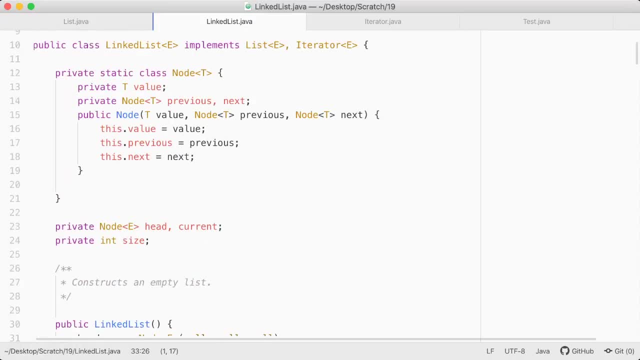 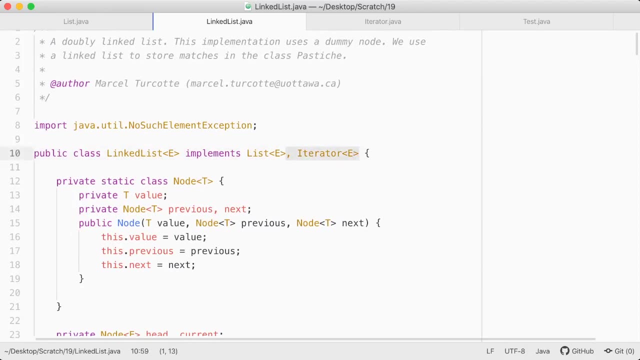 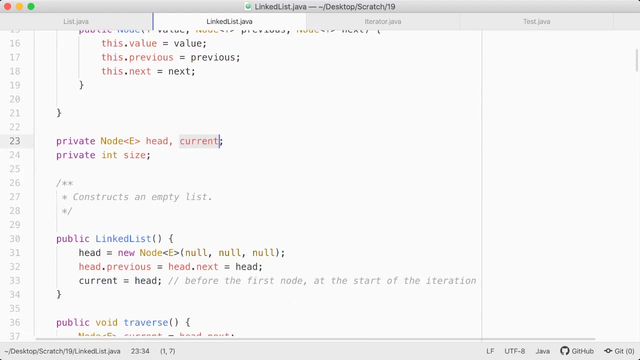 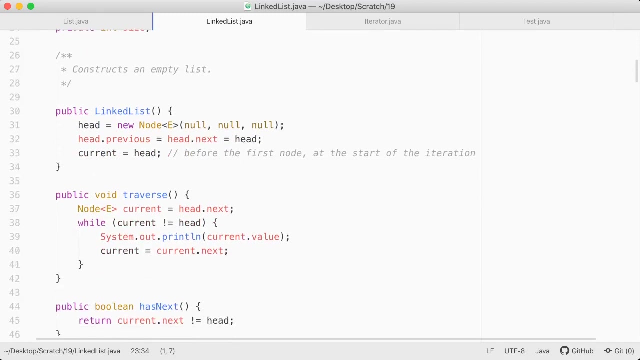 working okay so not too complicated what we said is let's give the responsibility of implementing an iterator to the list itself in order to do this the object of the class linked list has an instance variable current initially when the list is created we would 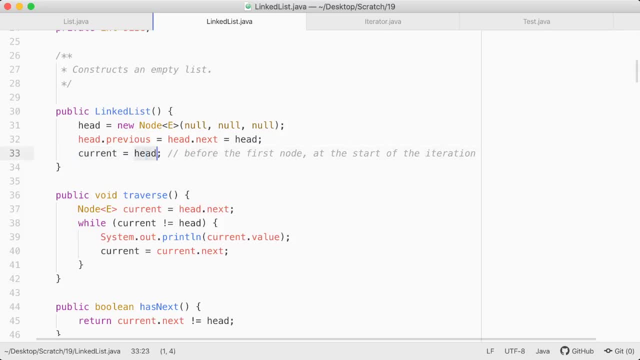 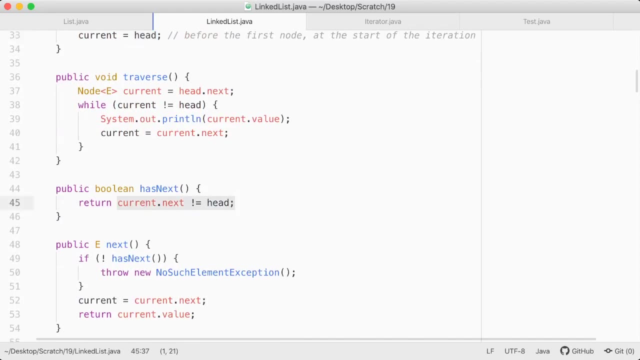 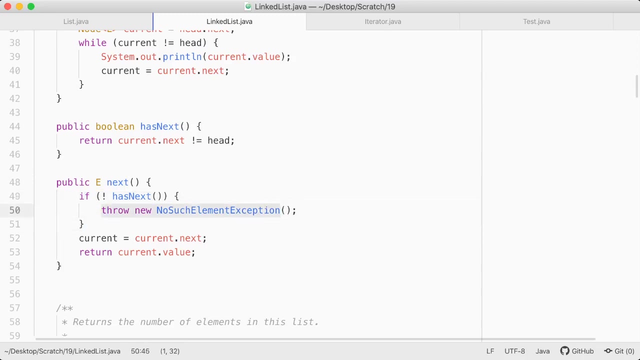 you set current to be pointing at the dummy node the method has next would return true if current dot next is different than head it's not we're not at the end of the list current dot next is different than the dummy node the method next if there's no next element throw an exception otherwise move forward return a value 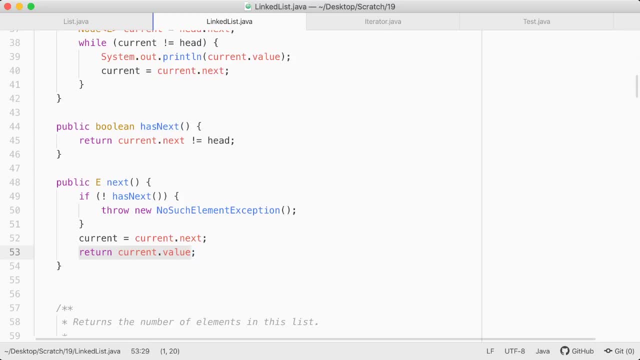 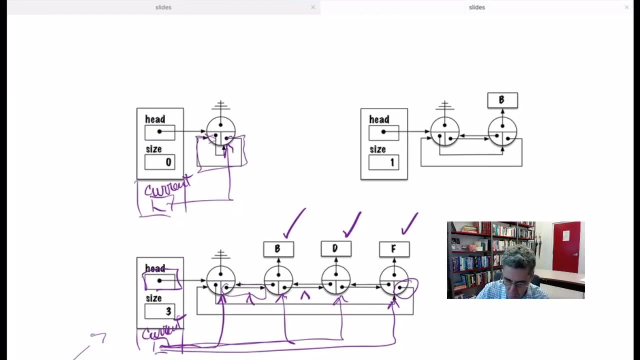 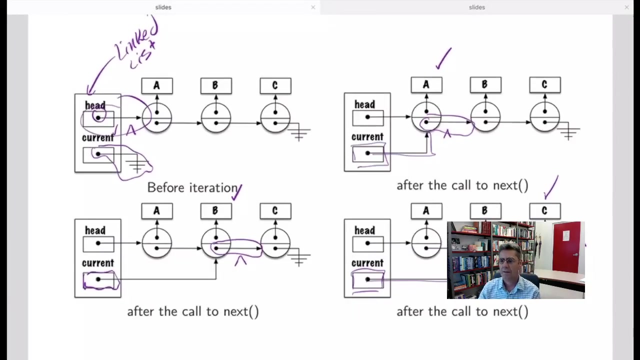 okay so i like this idea a lot it's um it it it's giving you a good intuition for what's the state of an op of a of an object okay so here on the implementation that we have inside 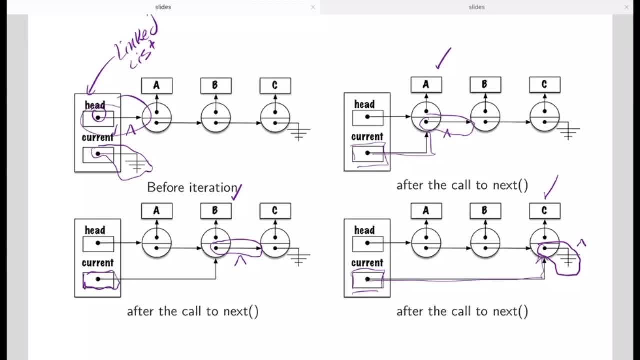 the slides the one where we using where where we are using singly linked nodes initially current is null and this means we're before the iteration when we start the iteration we say current equals to head after that for every call to next 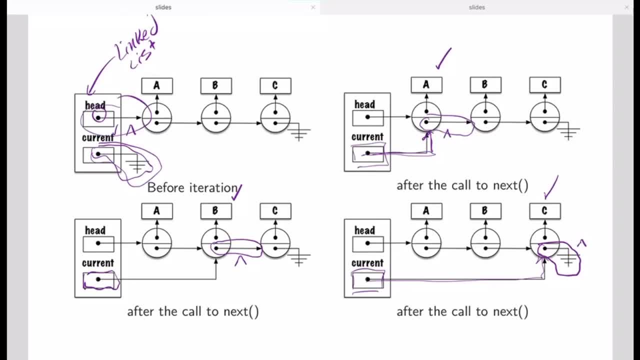 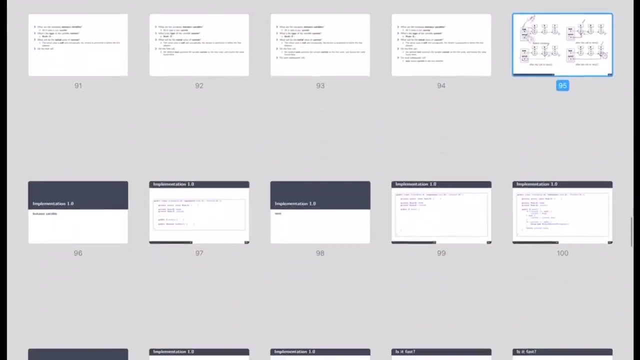 we say current equals current dot next and what I mean by state is the fact that the list now memorizes the last position that was visited by this iterator it's only a call to the method next that will move the iterator forward okay so question is now is it fast here's the result 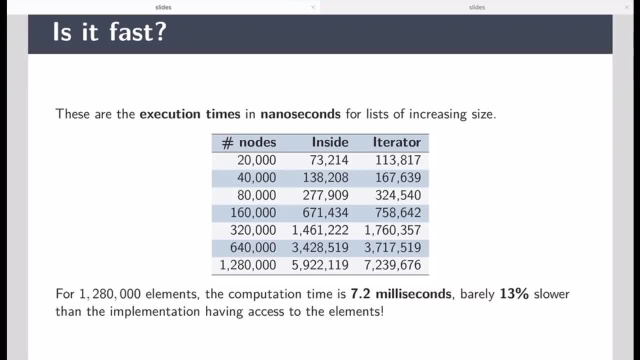 traversing a list when we are inside when we have 1,280,000 nodes 5.92 milliseconds when we use the iterator that we just created 7.2 milliseconds barely 13 percent slower 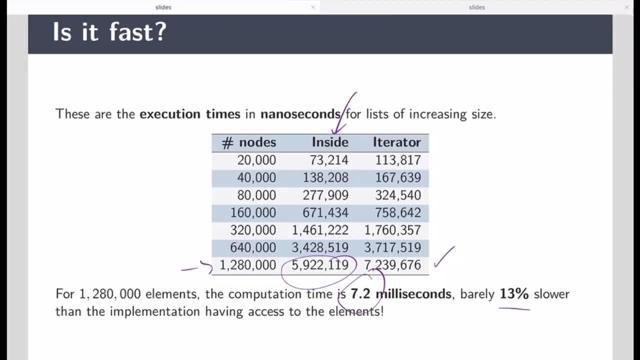 than the implementation where we are inside the implementation so this is a very very good results no compromise is made in terms of the encapsulation 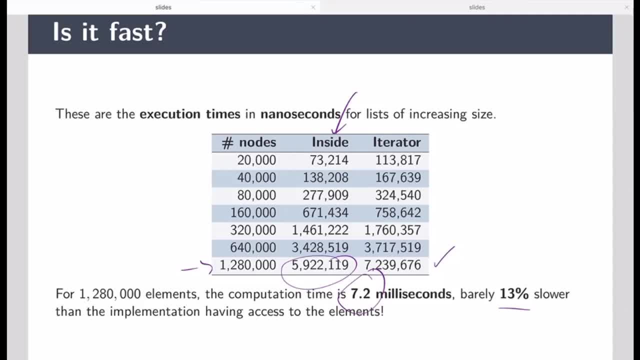 we've never made any variable public all all the variables are private we're providing a mechanism to visit every element of elements of this list and it's fast 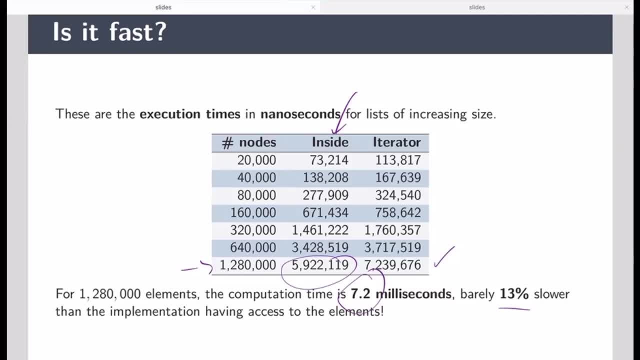 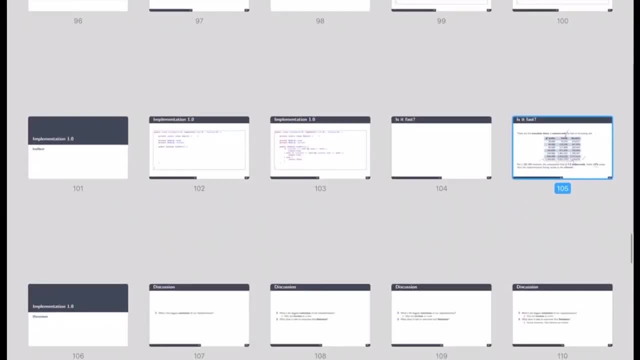 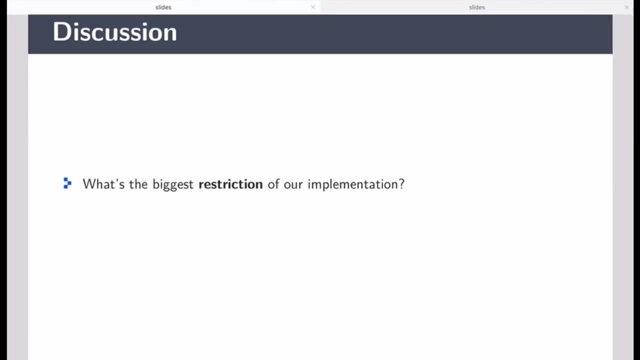 it's super fast so what's the problem then what's wrong what's the biggest restriction that we have for our implementation the biggest one is that there's only one iteration at a time this part is not indeed you don't find any 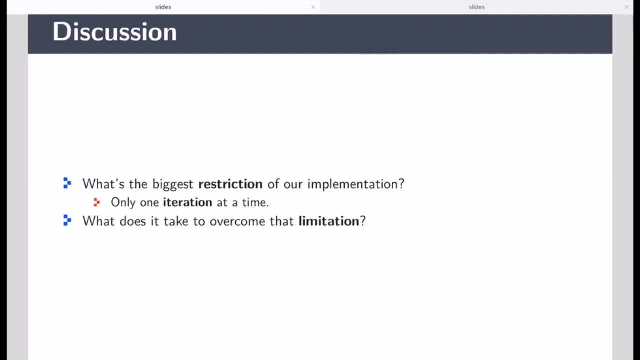 There is only one iteration at a time there is 90 in the application처 and maybe however many applications are right it can be like a is that there's only one iteration at a time if we wanted to have two three four as many iterators as we want on the list we cannot achieve this if you want you can pause this video and 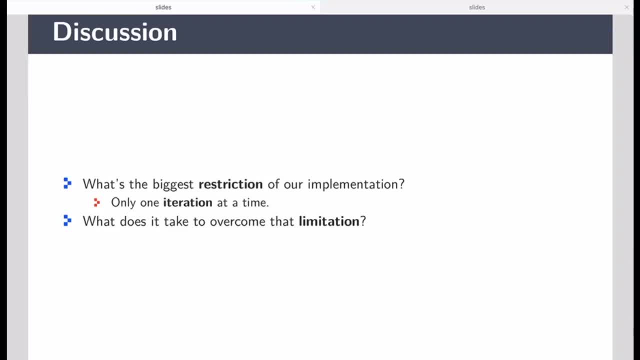 think how would you solve the problem with the knowledge that you have how would you solve it I can tell you we can solve this problem with the information that you have with the knowledge that 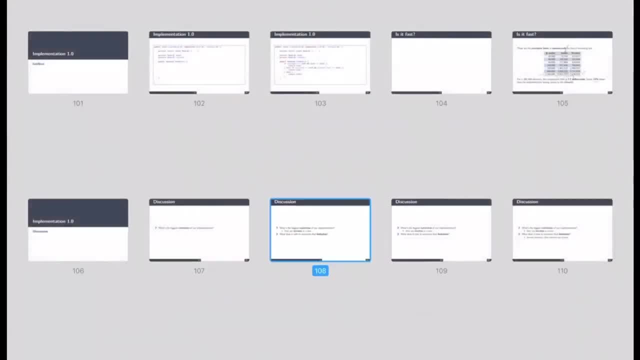 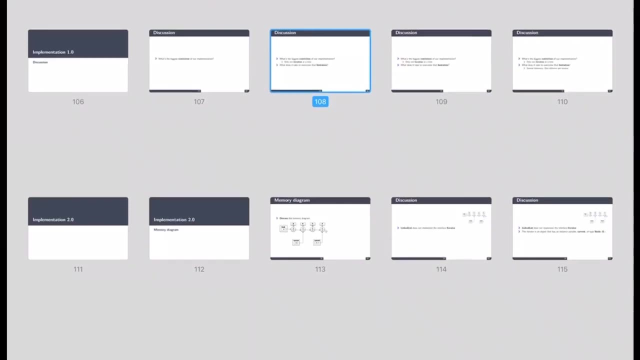 we have so far in ITI 1121 we can solve this ok if you made a pause and you're back I'm gonna show you some memory diagrams of my solution and I want you to reverse-engineer my solution 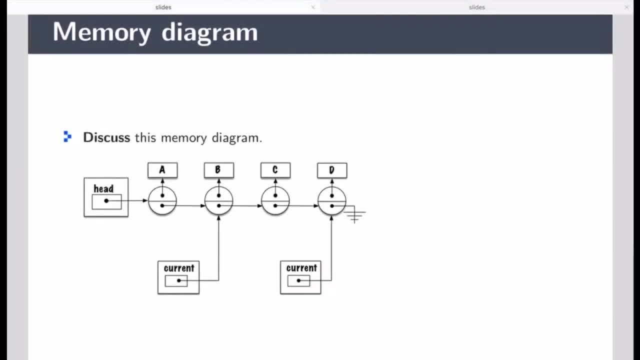 solution. If we want to have multiple iterators it means that there there will be multiple instances or multiple variables of type node each one of them pointing at a node they could be pointing at the same node obviously but pointing at a node of the list and they're like a bookmark on the list they're pointing at a node and they memorize where we are in the iteration and the idea will be like before so here you can imagine that I can have I is pointing at this iterator J is pointing at this iterator and I want if I call I dot next what I want is 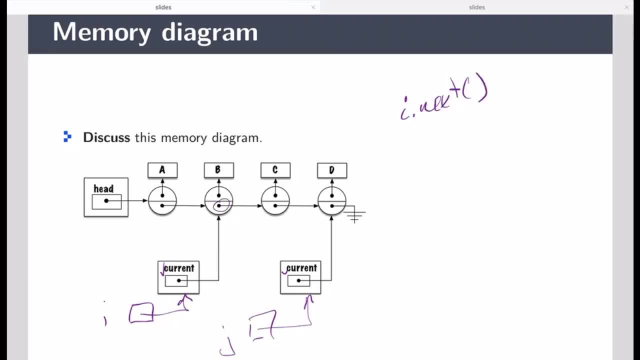 that we will copy current dot value into this particular variable current and return current dot value so we that's going to be the behavior of our iterator okay so now now we have a challenge how how do we do this okay so we cannot give to the users of the linked list 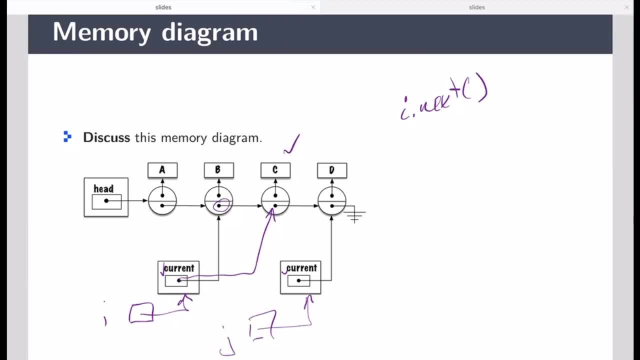 the possibility of declaring themselves variables of type node we can't because the nodes are private we want to keep this implementation private the instance variable next is private so we cannot allow programmers outside of the class 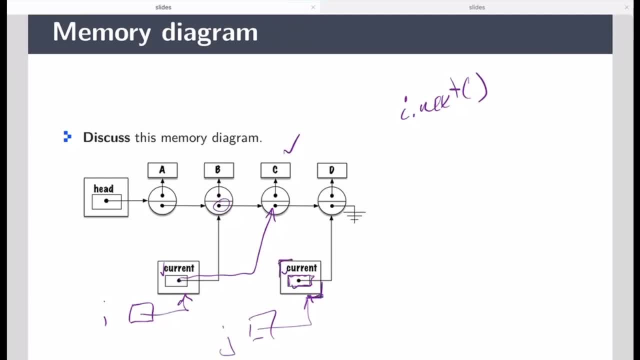 interface be generated by the iterator, correct? 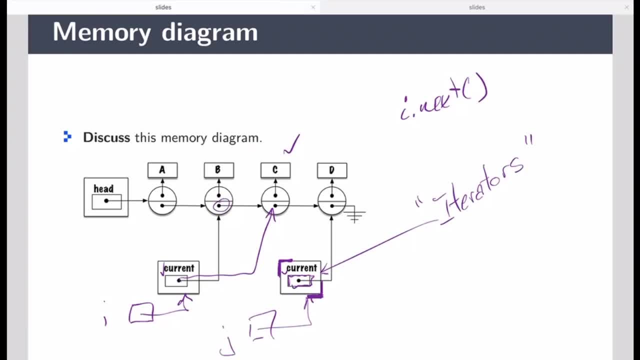 So this variable is a variable and in it's class it 703 layers I talk to it is and it's class is ten components it's an iterator that violates short Obviously how do you look like? What it means is that this object has a method next and a method has next. 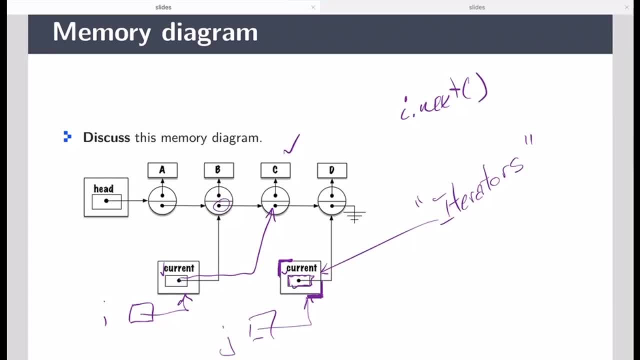 So for this next implementation, what we're going to do is we will be declaring a new static nested class that we will call myListIterator. 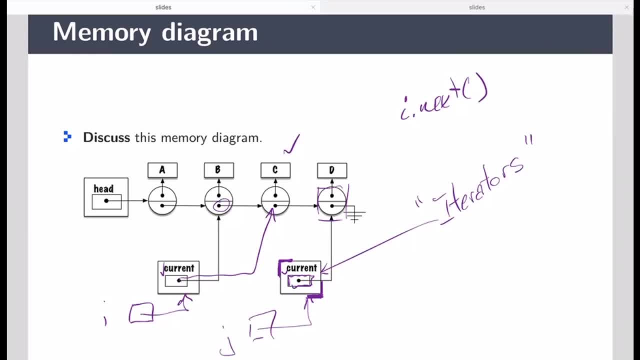 And it's that particular class that will be implementing the interface iterator. We're now giving the responsibility of implementing the interface iterator to another class. 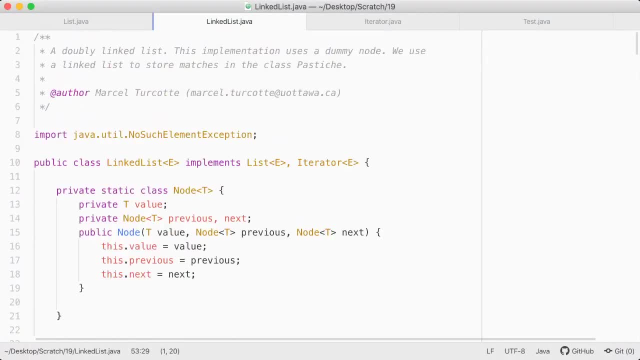 Okay, let's work on this. 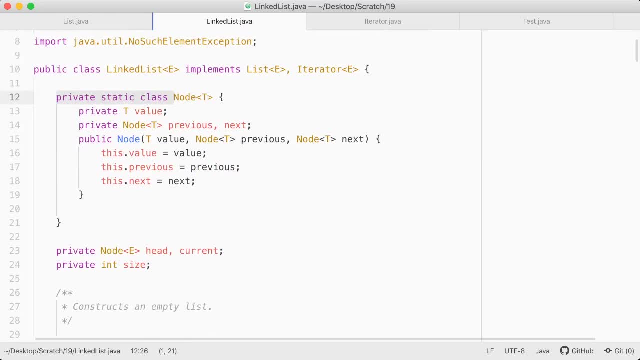 So... We're going to use another static nested class. Let's call it myIterator. It has its own type. If we want to avoid confusion, let's say that the type is you. MyListIteration implements iterator for these things of type you. 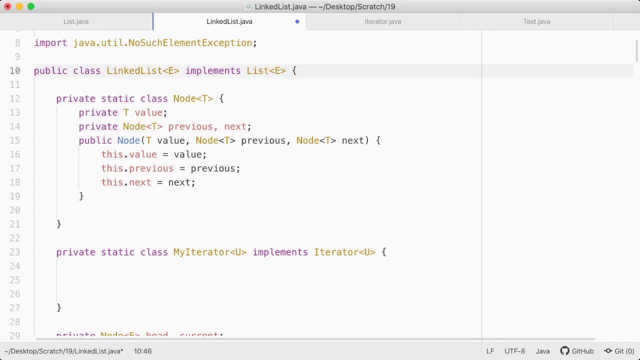 So it's no longer the case that the list is responsible for implementing the iterator. Its objects... 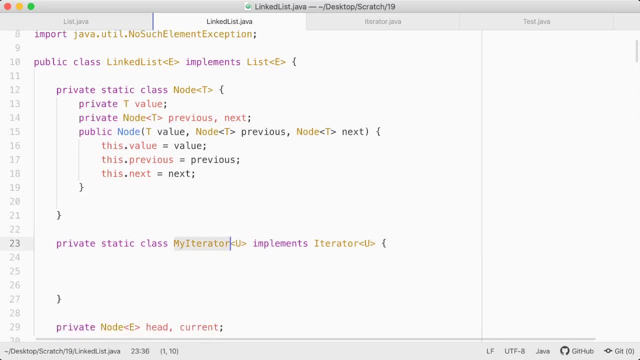 Of the class myIterator that will be doing the job. 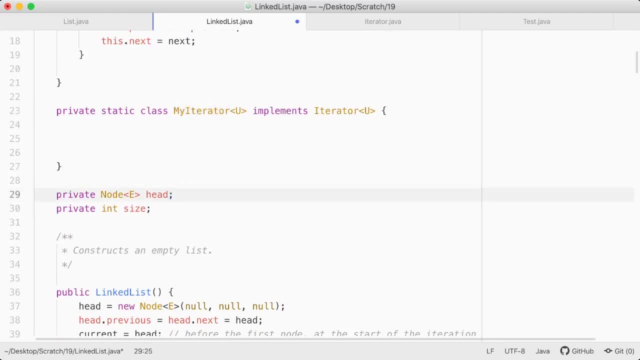 The list no longer needs an instance variable current. 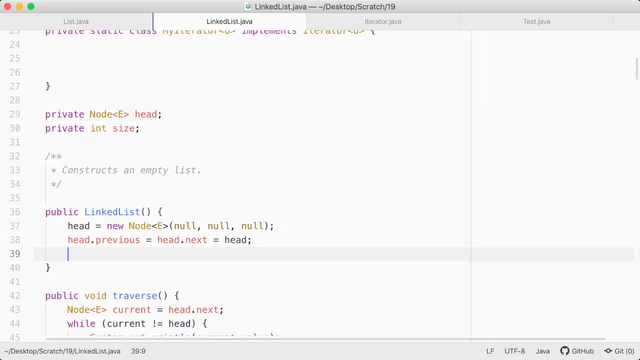 I have now to change this. The method has next and next. 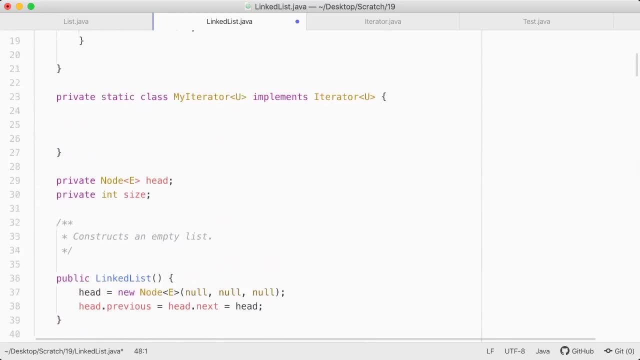 So, in the literal world. As before. 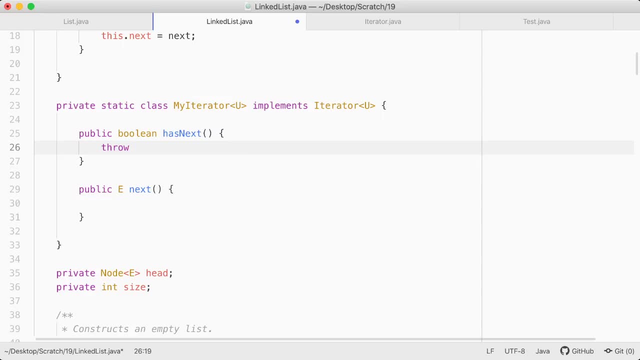 I really like to have a strong starting point where... 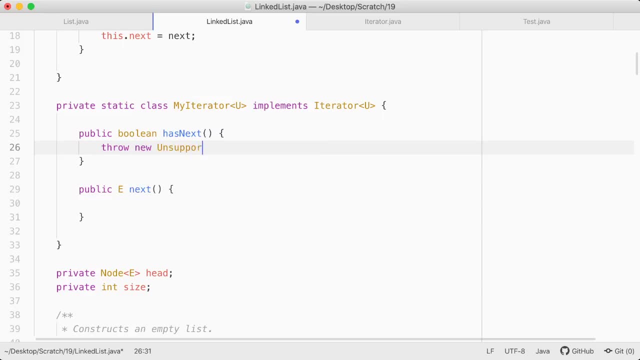 I know that everything is safe in terms of syntax and types. So, throw new... operationException not implemented yet 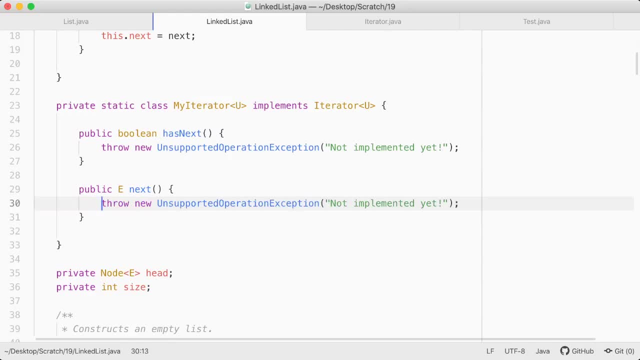 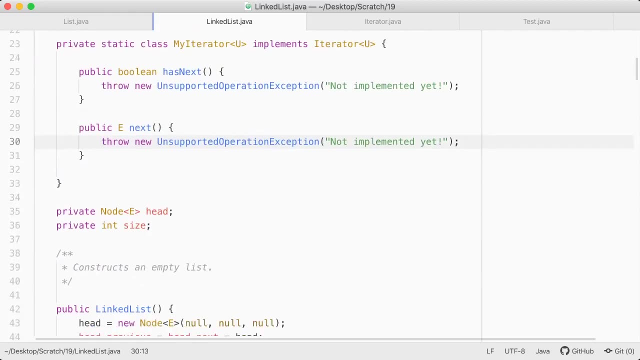 okay so normally in class i would ask you if this would compile or not and with your help we would make sure that we don't have any compile error okay let's now javac linkedlist.java 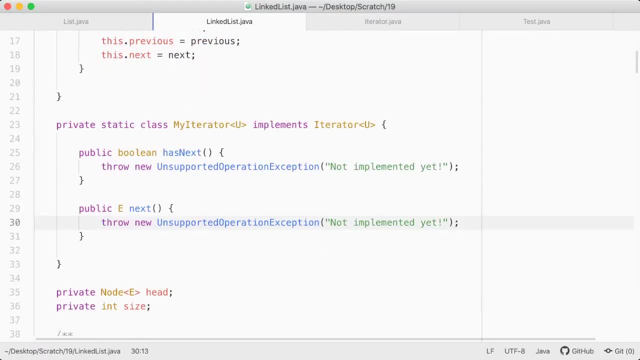 okay so made a typo obviously because i decided that the type here would be you oops okay 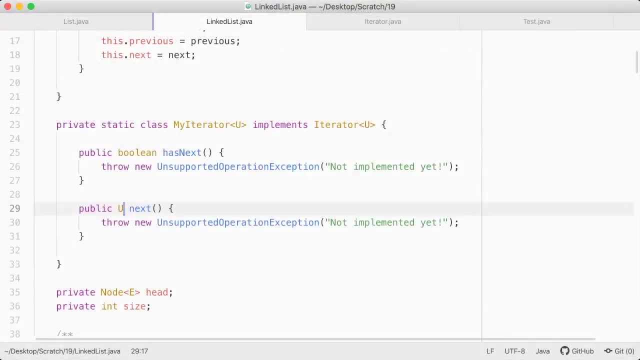 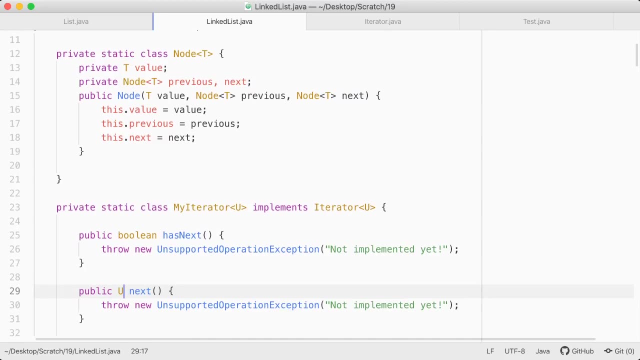 it complies okay so what this means is simply that there are no syntax error and from the point of view of the types so far so good this seems to work 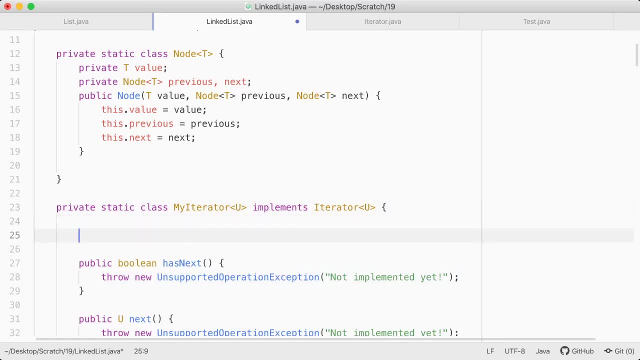 what are the instance values so private node and here you is our type current here what we said is 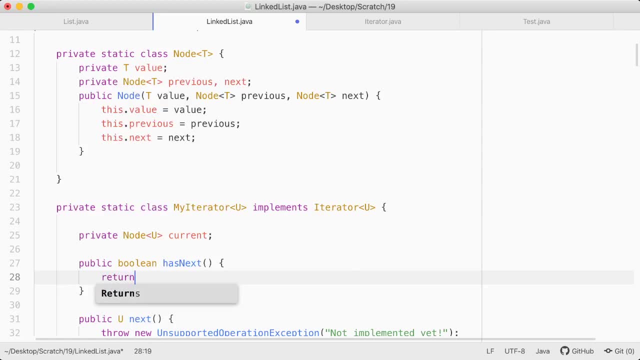 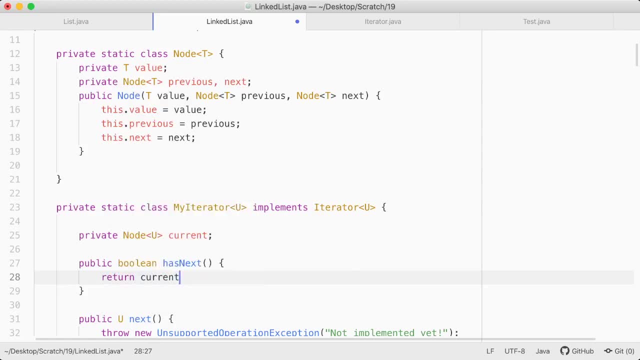 here what we said is the click here 05.285.89T0000003 it's this cioè if the instance variable is pointing at the head node then we're at the end so there's a next one and then this is therefore a next step below evidentially when the iterator is created current will be pointing at the domino if the instance variable is pointing at the head node the dummy node then this means that we're at the end time then this means that we're at the end so there's an next step behind us that's tocher…? 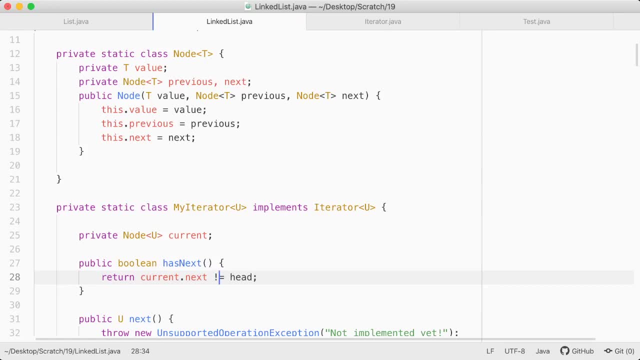 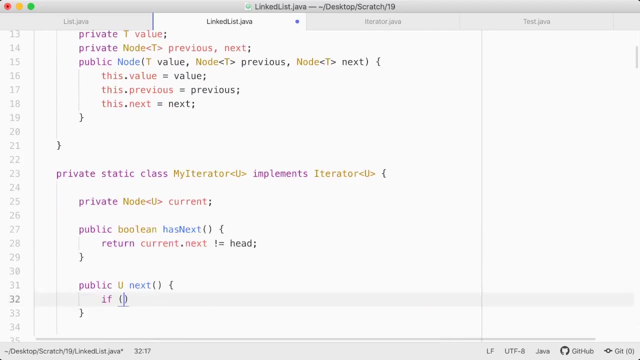 if it's not pointing at head here if hasNext is not true so not hasNext throw 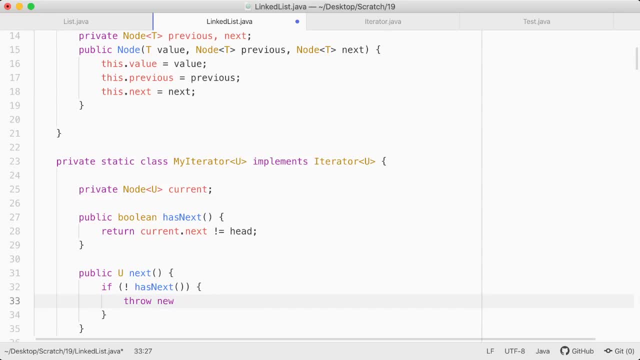 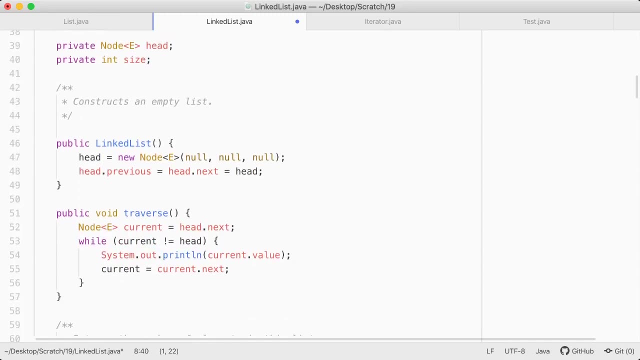 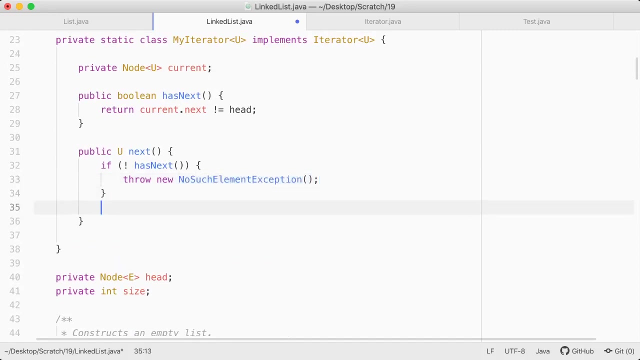 new noSuchElementException like this otherwise move forward current equals current.next and return 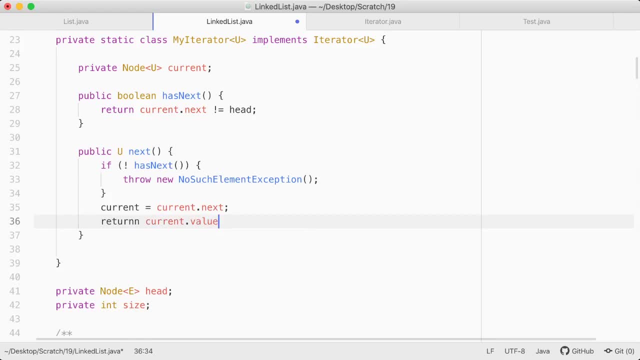 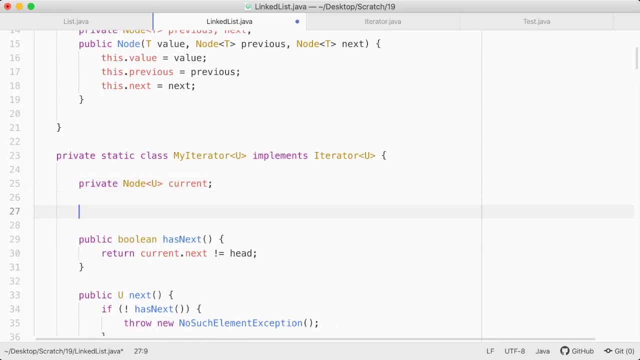 current.value now we said that the work of making current pointing at the dummy node would be done when we create a new iterator so let's do let's implement a constructor private myIterator and here we want to say current equals someHead and here look at this will this work will this compile the reason why I'm making this very long 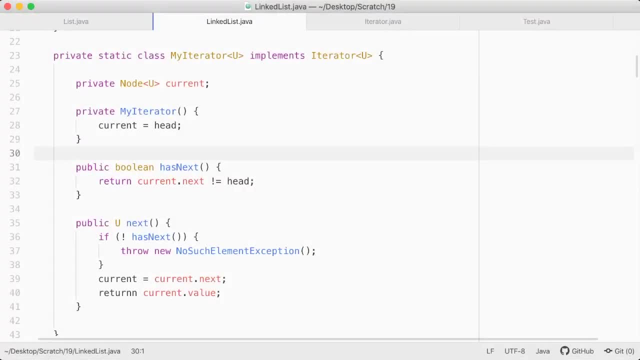 on pause is because i know that it will not be compiling i know that there is an error 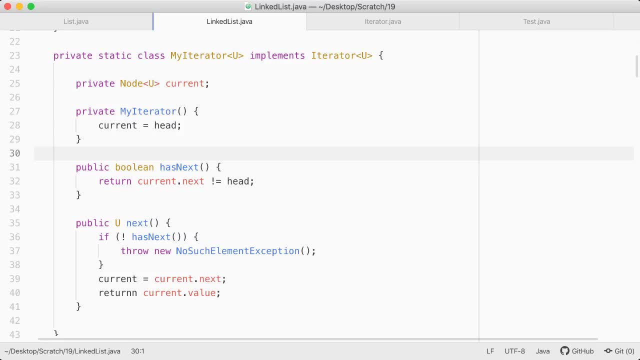 if you need if you want pause this video and think where will this error be reported what is the problem 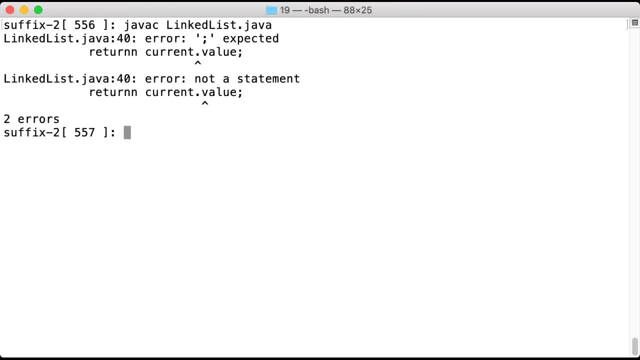 let's compile okay there was a syntax error that was not expected where is it return here with 2n that was silly let's compile again 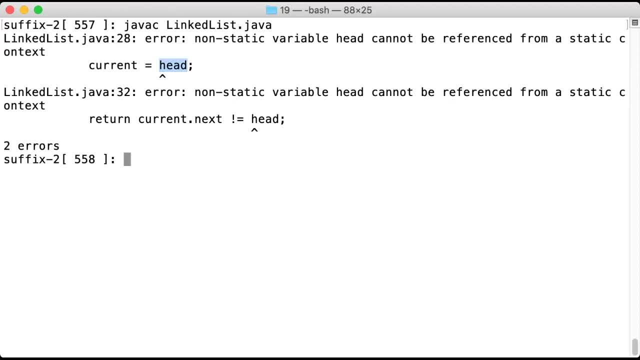 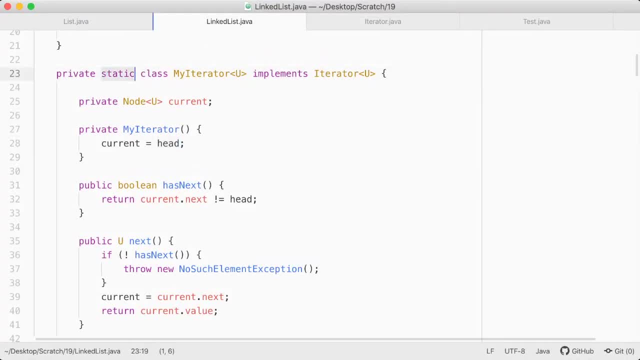 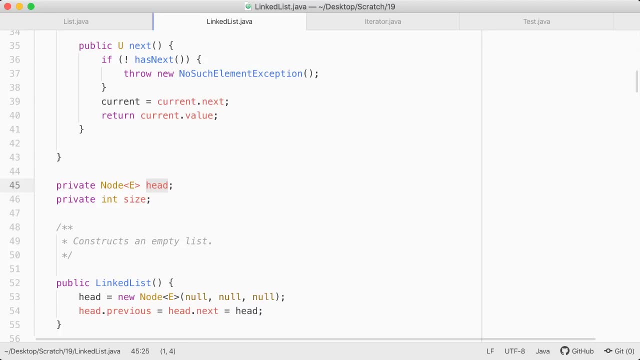 so here do you see what's wrong we're trying to access some variable head from a static context and head is a non-static variable that's not going to work so the iterator has to know to which list it belongs 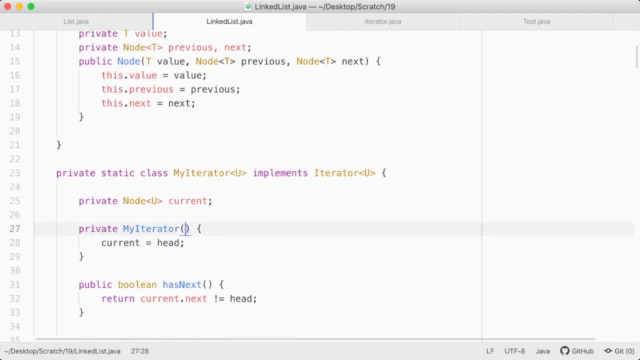 so what i'm going to do i'm going to propose to tell the iterator what it lists what list it belongs to so here that would be linked list of type U myList and we would make the iterator know 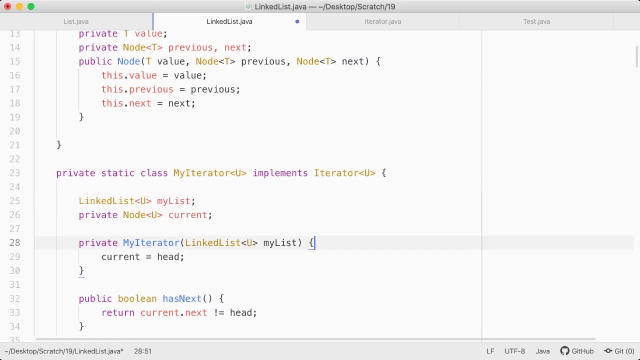 remember what list it belongs to this 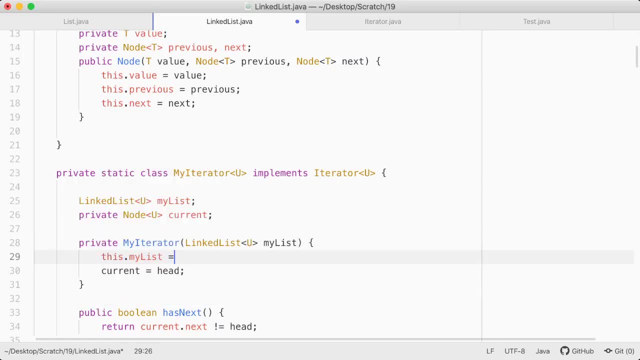 myList equals list equals myList 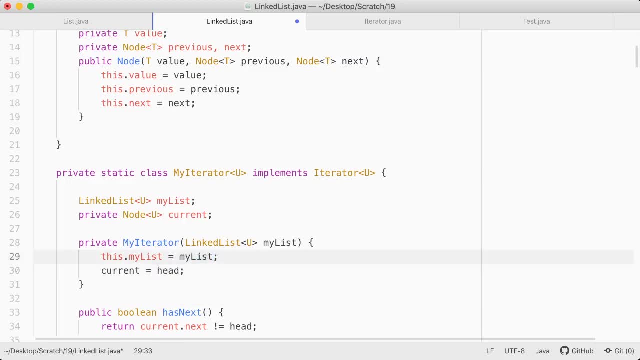 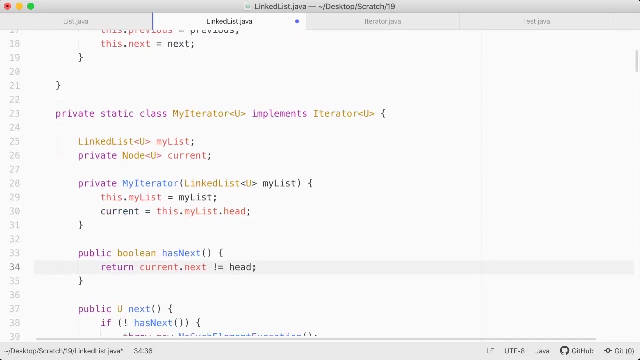 here it's going to be myList.head here as next it's going to be and now it compiles 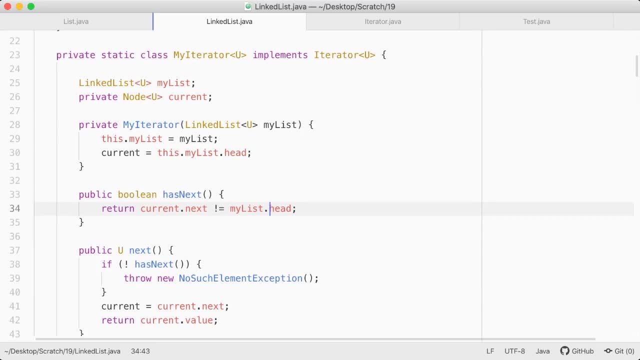 ok so an object of the class myIterator is told you belong to this list 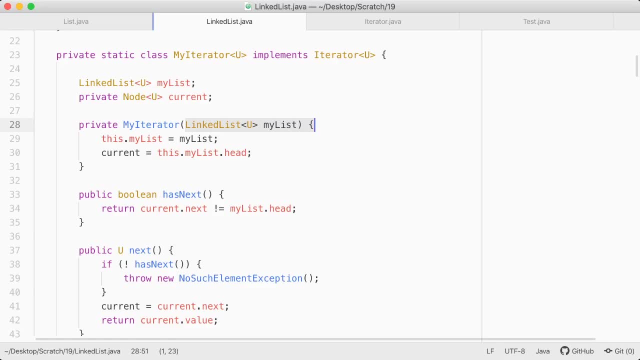 or that list it's when constructing an object of the class myIterator 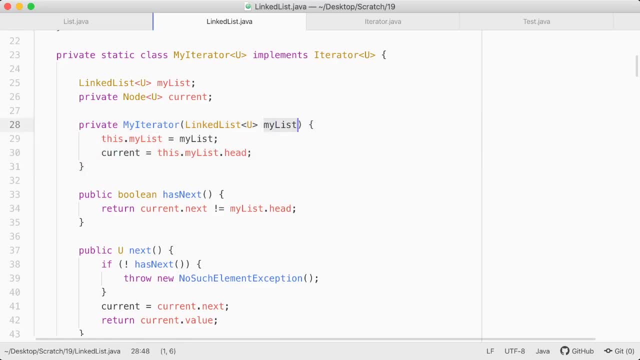 that you belong to that we would provide the list that the Iterator belongs to 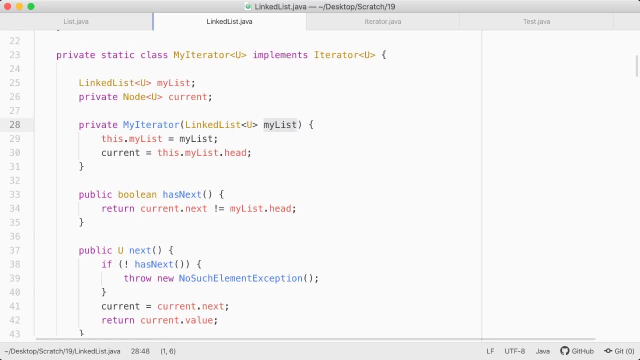 and then knowing that the Iterator 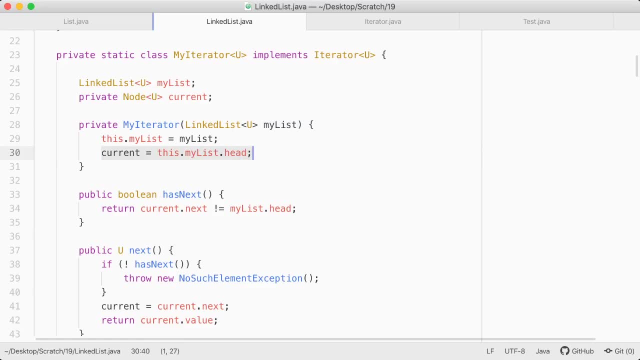 will now have access to the variable head of the list 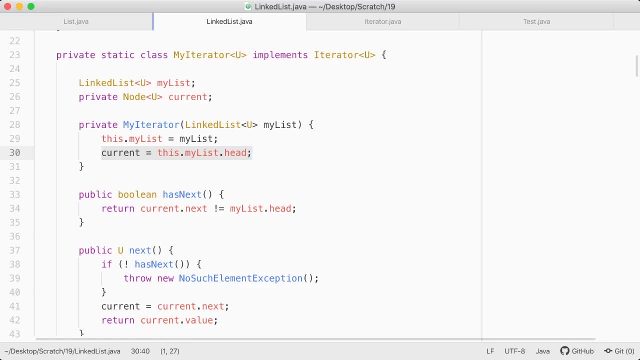 that it belongs to can actually show you some memory diagram for that 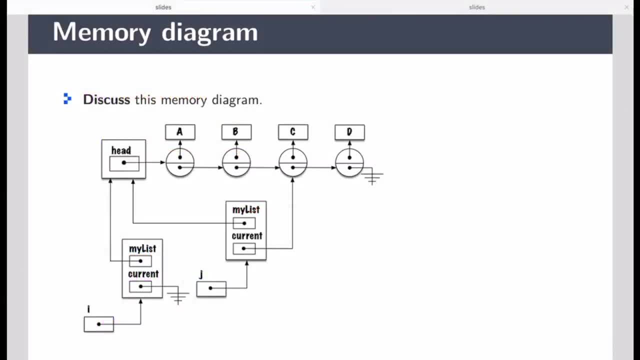 the Iterator belongs to ok so so here this is an object of the class my iterator it has an instance 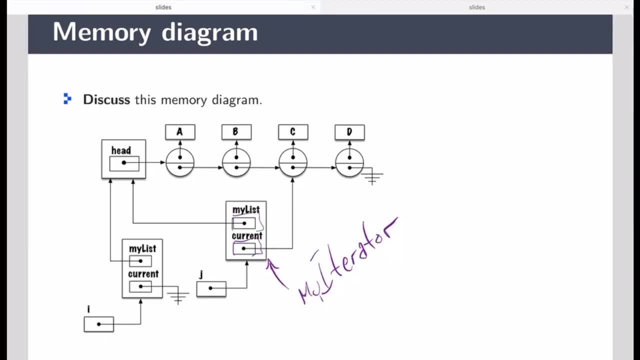 variable current and it has an instance variable my list this is an other object of the class my iterator its instance variable current is null in the singly linked implementation 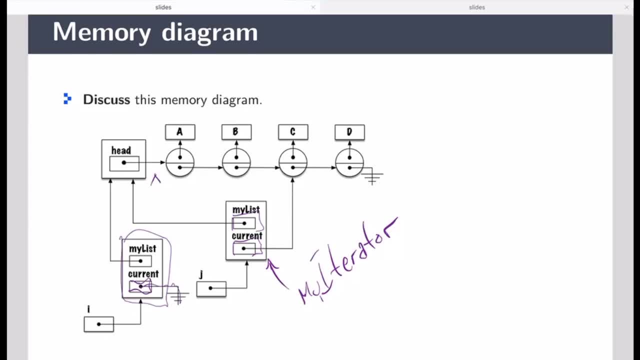 this is this means on before the start of the iteration it has an instance variable of type my list this is my list and if we are to call i dot next it's going to say hmm my 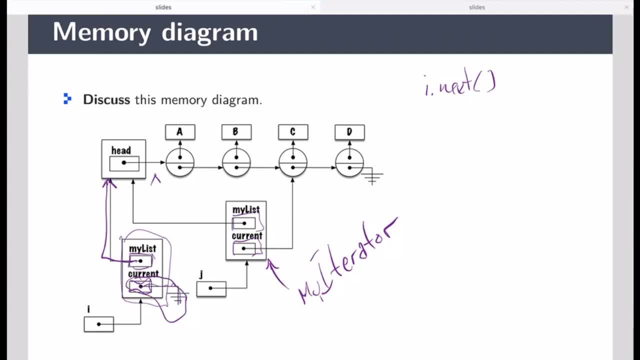 instance variable current is null i am before the start of the iteration let's start let's copy 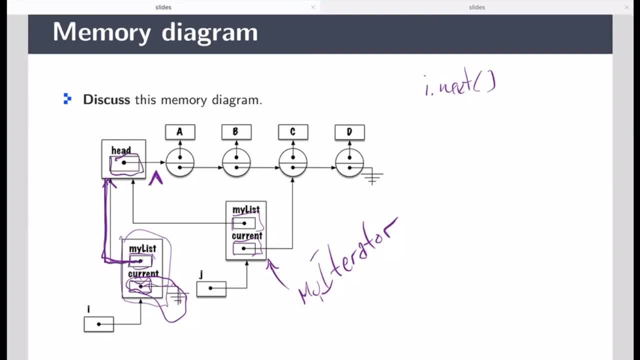 my list dot head inside current return current dot value so we're starting this iteration if we call j dot next next the variable current of the object designated by j is not null so therefore it's already 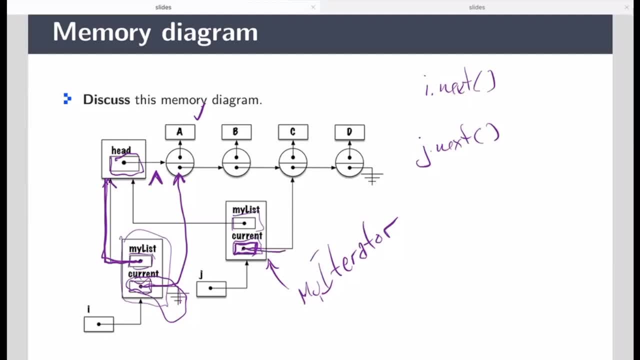 inside an iteration it's going to say current equals current dot next it will move forward and return d 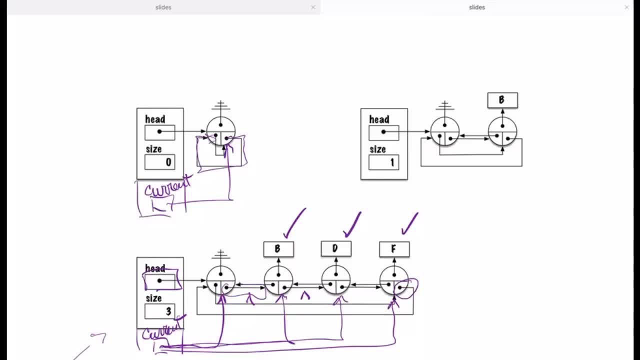 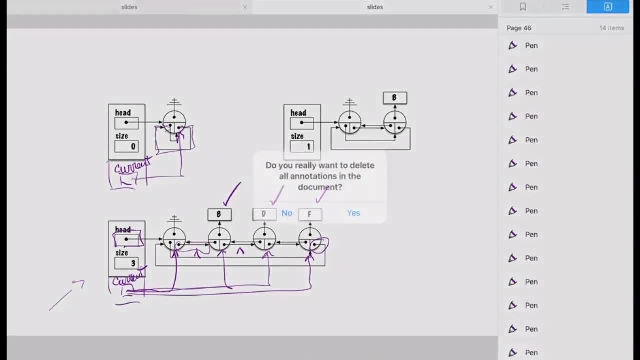 here on our implementation let me remove all these annotations okay 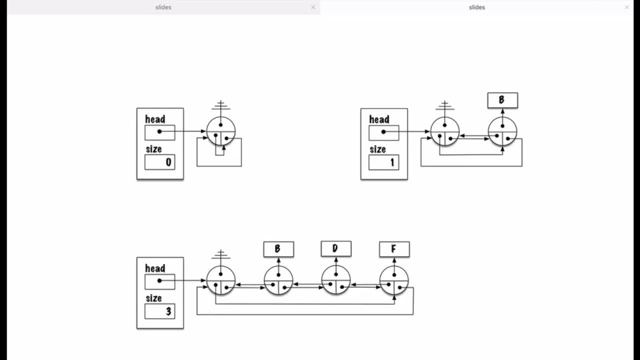 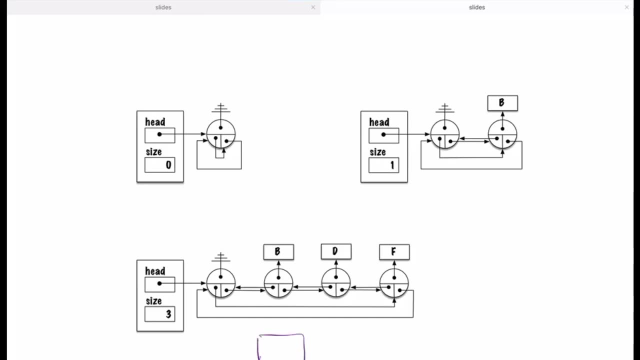 so an iterator is an object that has a variable called my list and 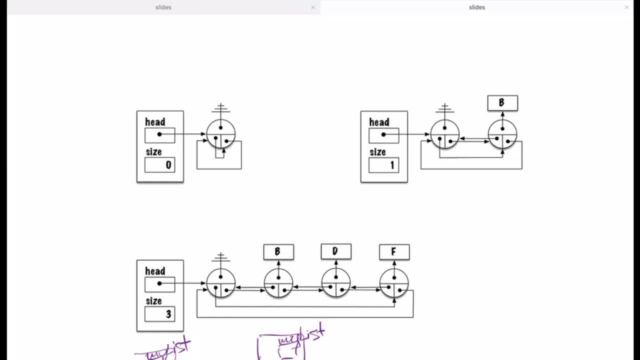 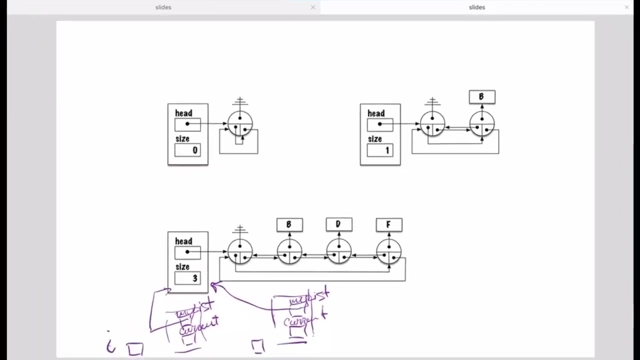 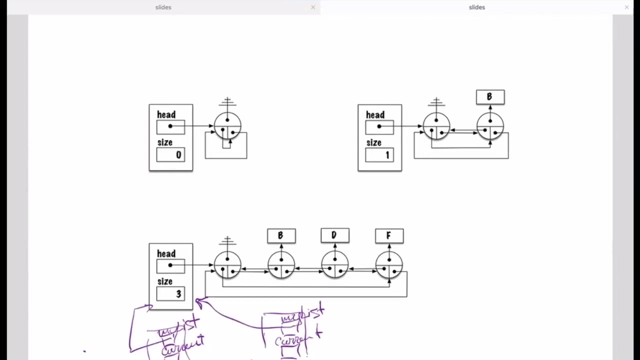 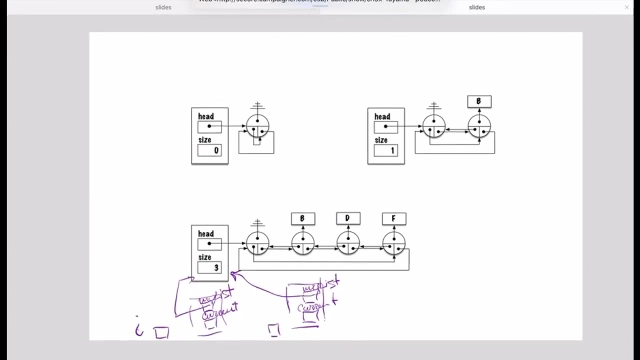 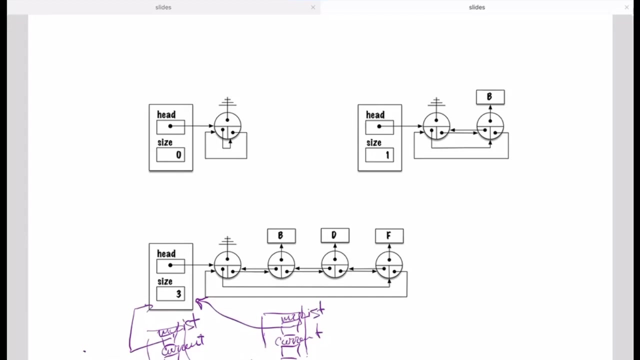 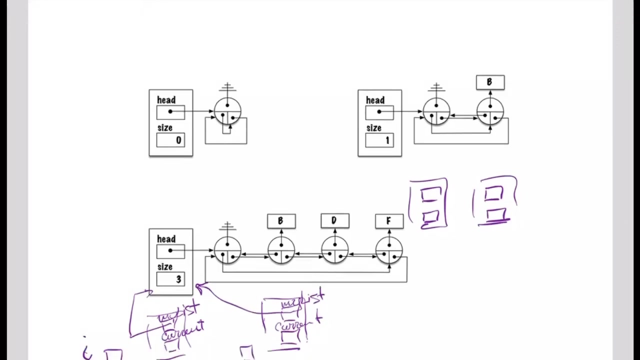 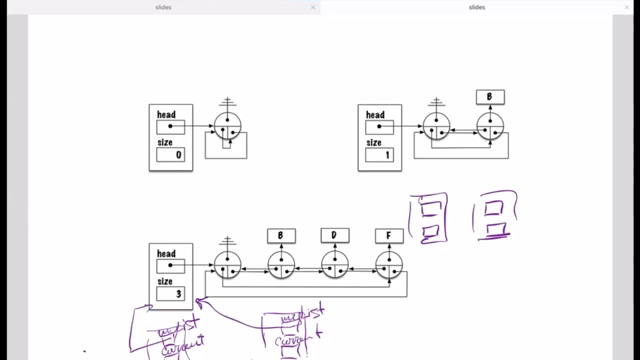 a called current so the iterator is for this list and this one as well somewhere in some program we possibly have I oh I see that it's you cannot see okay so I'm gonna make try to make this hmm fortunately having a hard time making this smaller okay let me if I do this you can barely see okay so let's start over okay let's go here where you can see my drawing okay so we have my list and current my list is at the top current is at the bottom okay we just do a little thing here okay so and the top is my list my list at the bottom current current current let's have I pointing here J pointing there they're both iterators for this list and I is pointing at the dummy node and in j current is pointing here if we call i dot has next it will say yes there are more elements inside this iteration because current dot next is not pointing at the dummy node current dot next is different than head if we call i dot next it will copy current dot next to current as a result of that 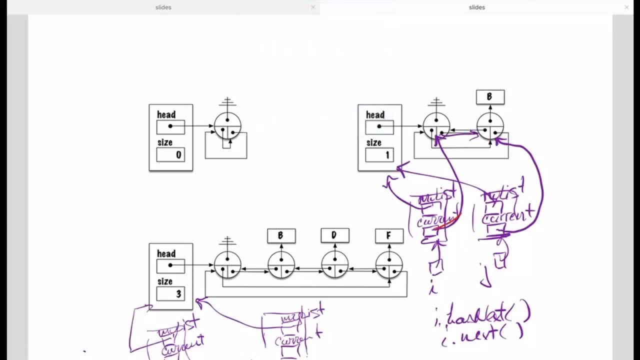 current will now be pointing at the last element of the list for both iterators if we ask i dot as next or j dot as next they will both return false because 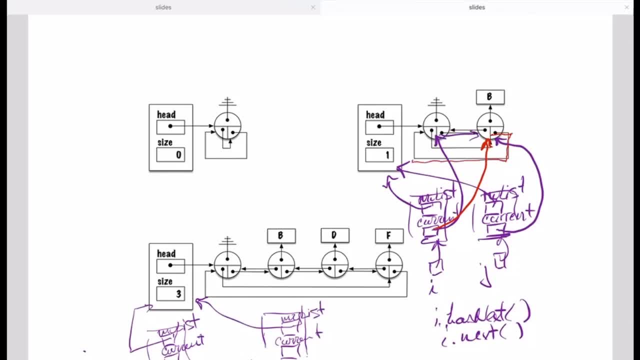 current dot next is equals to head 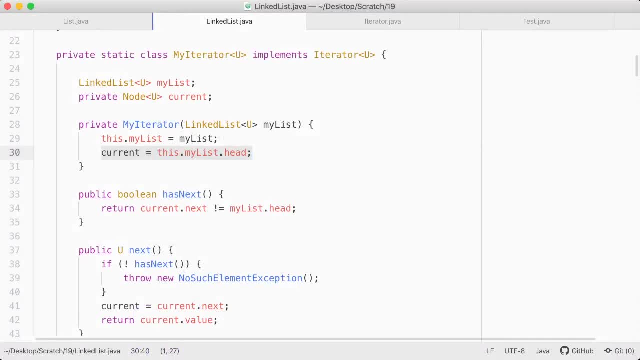 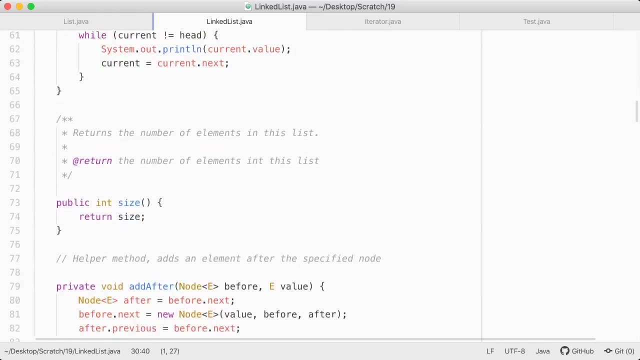 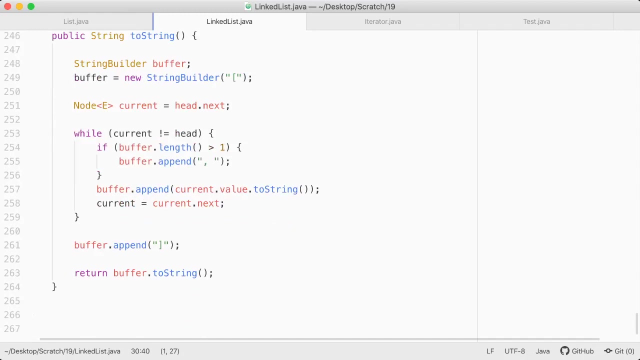 okay back to our implementation here i can show you here artificially how i would be creating these objects okay 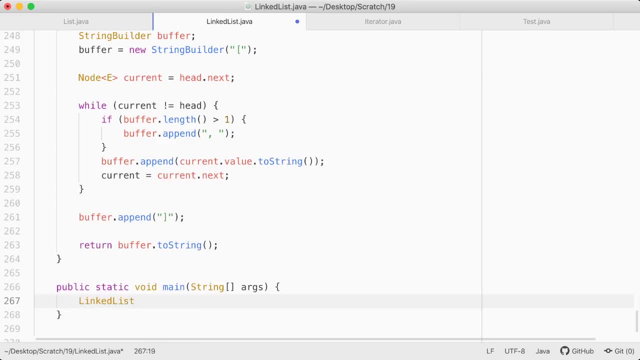 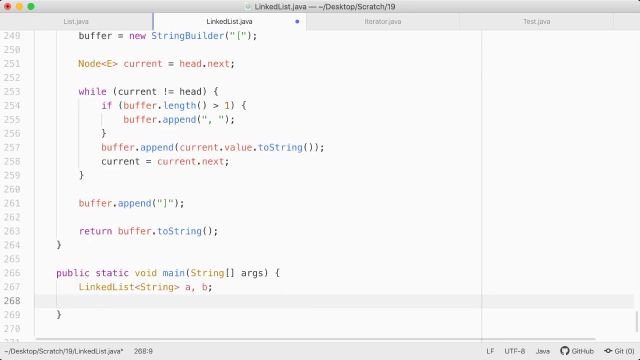 here let's have a linked list for some string here let's have a linked list for some string here let's have a linked list for some string for some string for some string here let's have a linked list for some string a and b let's say a equals to new linked list let's say a equals to new linked list let's say a equals to new linked list for some string for some string for some string like this 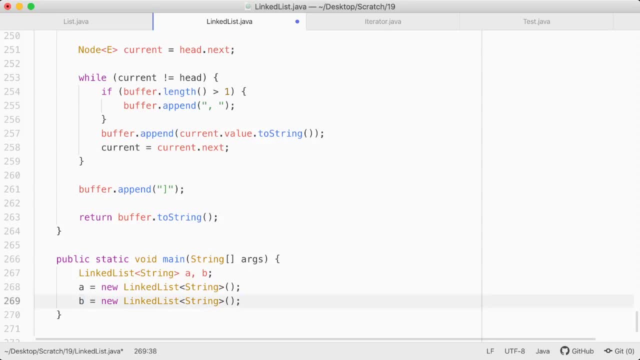 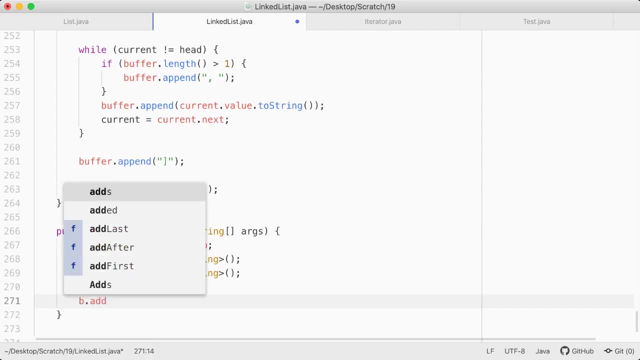 let's have b here let's have b here let's have b here say b dot add say b dot add say b dot add 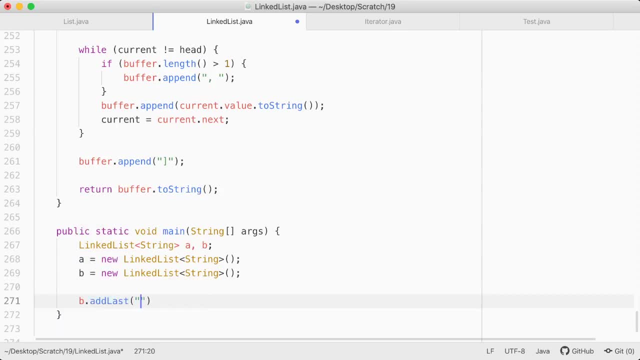 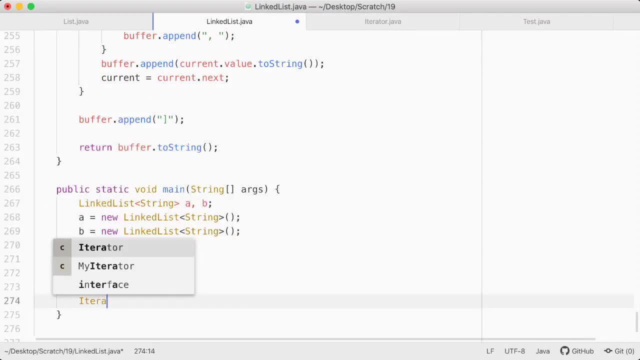 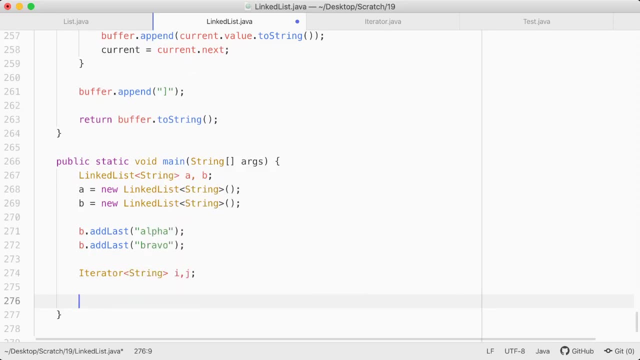 so far so good this compiles so far so good this compiles you can declare an iterator you can declare an iterator you can declare an iterator or string or string or string i and j i and j i and j i equals to new i equals to new i equals to new iterator for string for string 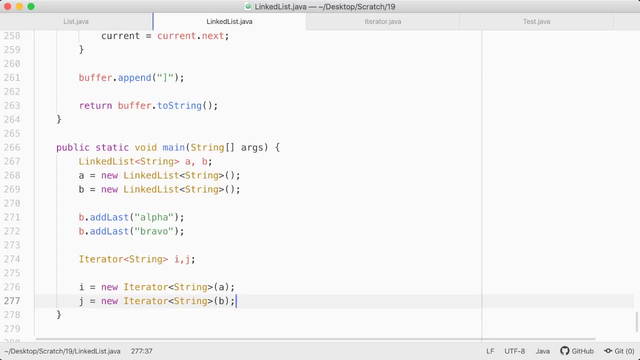 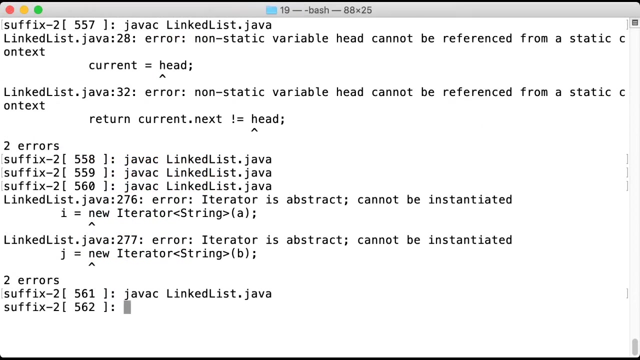 I was not paying attention we called it my iterator and the compiler very I was not paying attention we called it my iterator and the compiler very friendly reminded us of this friendly reminded us of this 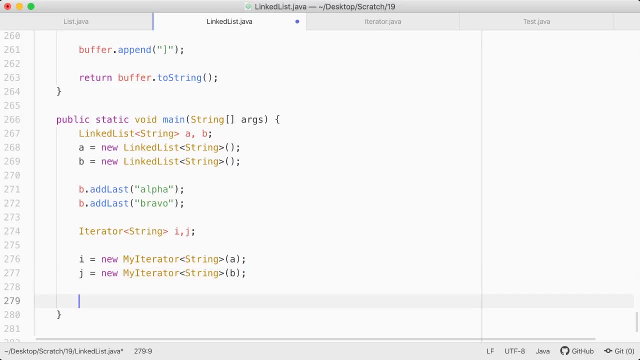 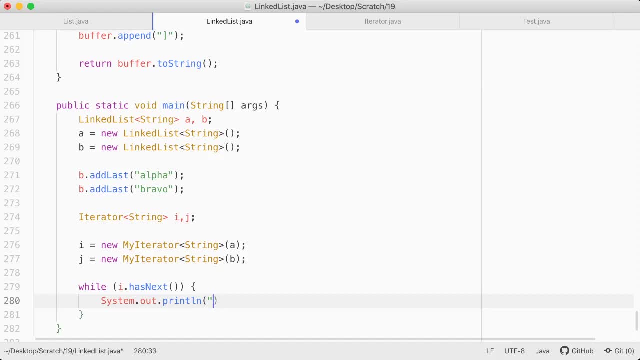 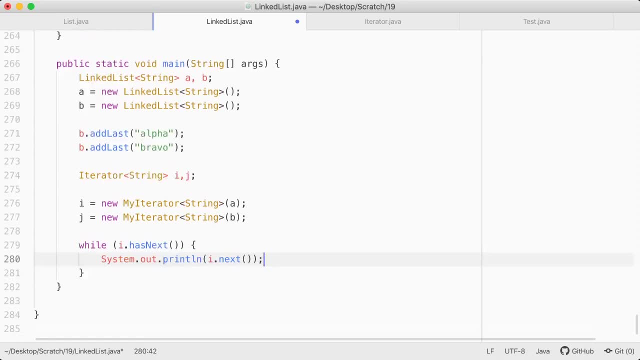 we expect that this is an empty list I've we expect that this is an empty list I've we expect that this is an empty list I've added nothing inside a and while j has 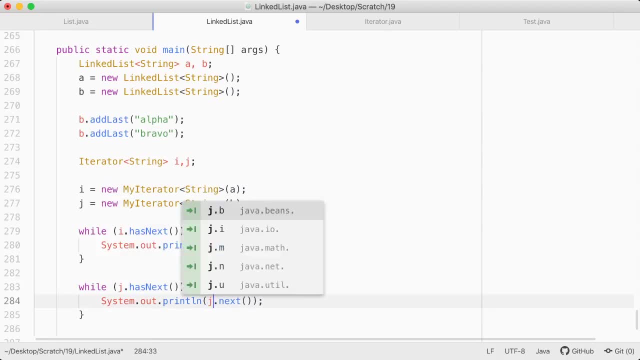 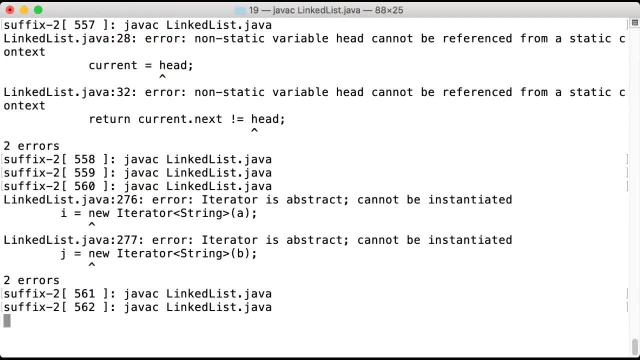 let's print j dot next next let's print j dot next now linked list as a main method I'm 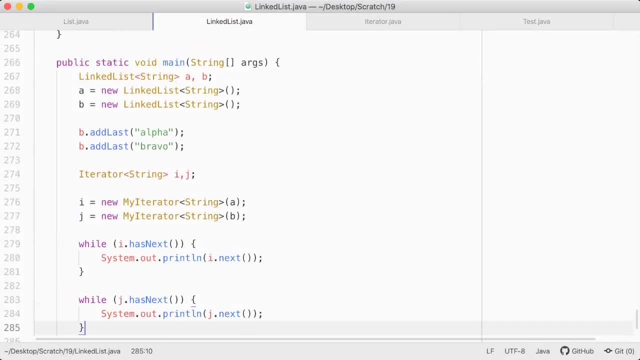 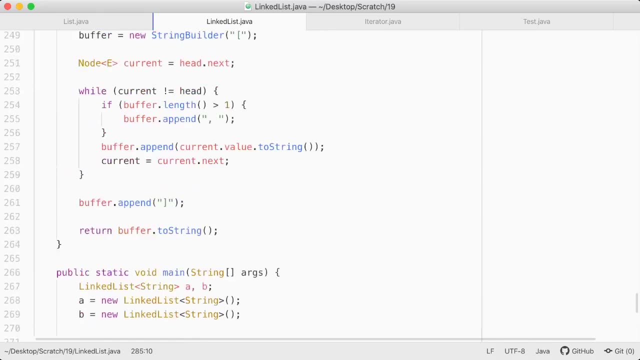 now linked list as a main method I'm now linked list as a main method I'm executing it it works but now that that executing it it works but now that that executing it it works but now that that doesn't seem so useful I'm inside the doesn't seem so useful I'm inside the 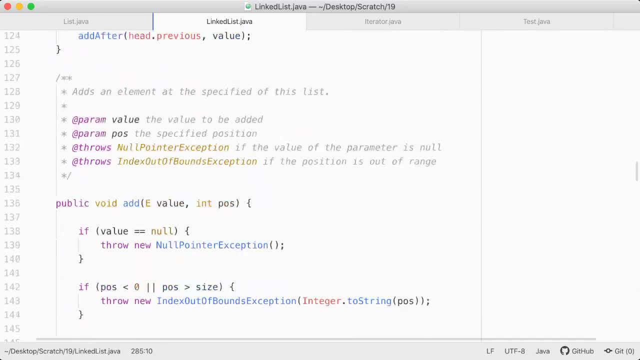 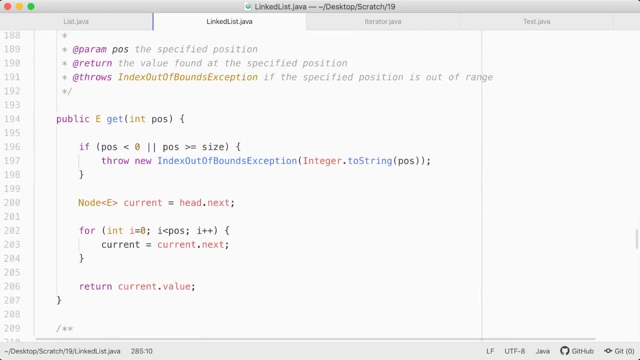 doesn't seem so useful I'm inside the implementation of the class linkless how implementation of the class linkless how implementation of the class linkless how will will will someone from outside of this someone from outside of this 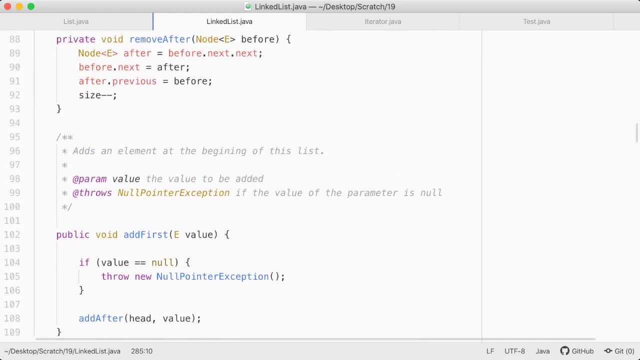 someone from outside of this implementation actually be able to create 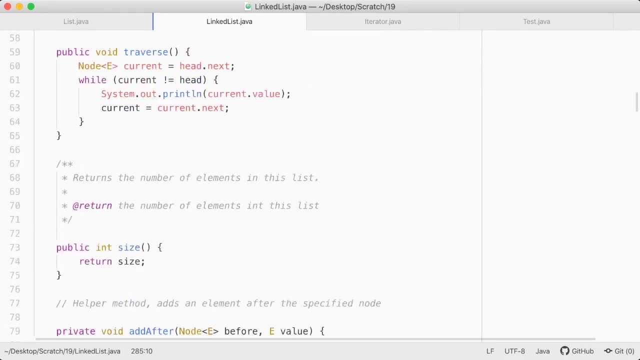 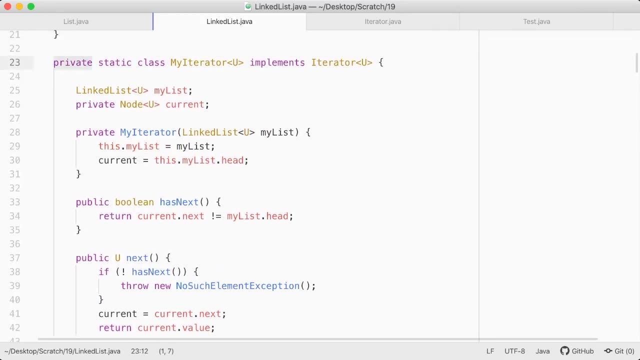 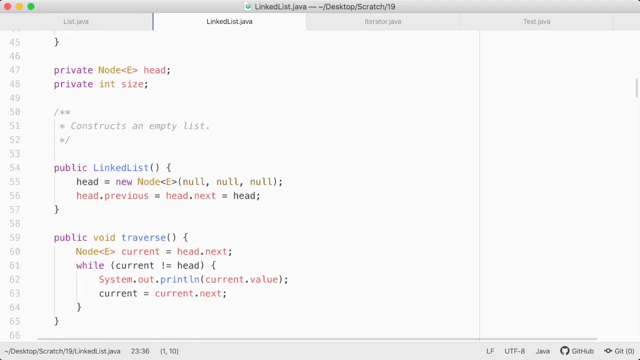 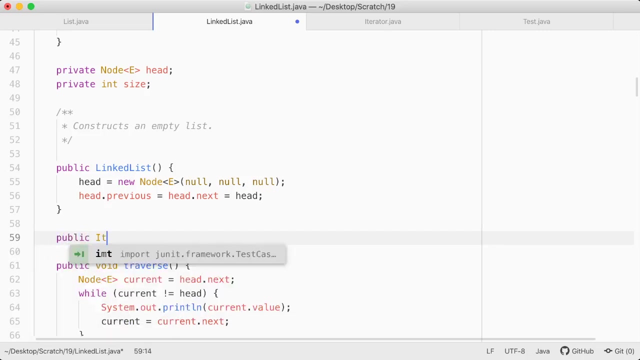 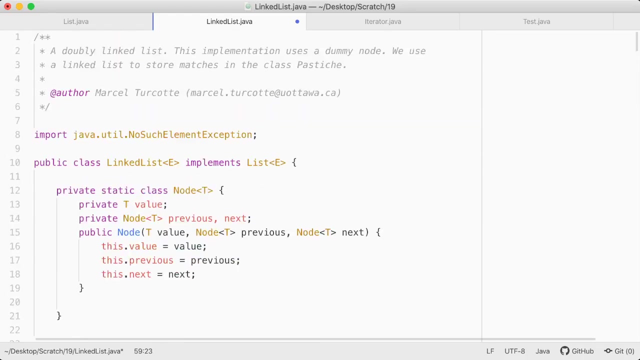 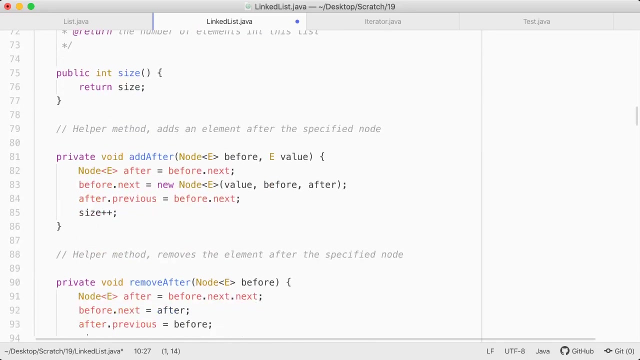 implementation actually be able to create these whoops these objects I'm looking these whoops these objects I'm looking these whoops these objects I'm looking for my class here how would someone from for my class here how would someone from for my class here how would someone from outside be able to create these objects outside be able to create these objects outside be able to create these objects of the class my iterator and of the class my iterator and of the class my iterator and the the answer will be let's provide a the the answer will be let's provide a the the answer will be let's provide a method public method it's an instance method public method it's an instance method public method it's an instance method iterator II so here objects of method iterator II so here objects of method iterator II so here objects of the class linked list are using the 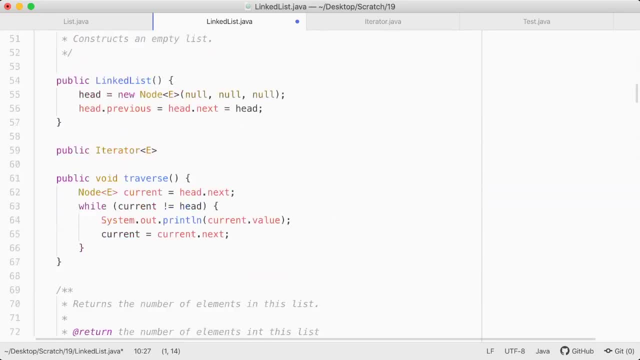 the class linked list are using the the class linked list are using the generic type II just lost the method 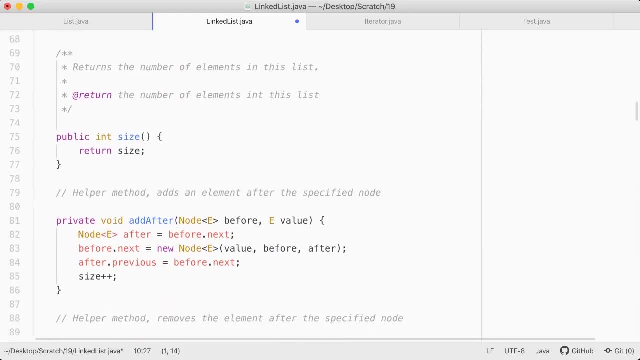 generic type II just lost the method generic type II just lost the method that I want to create where is it 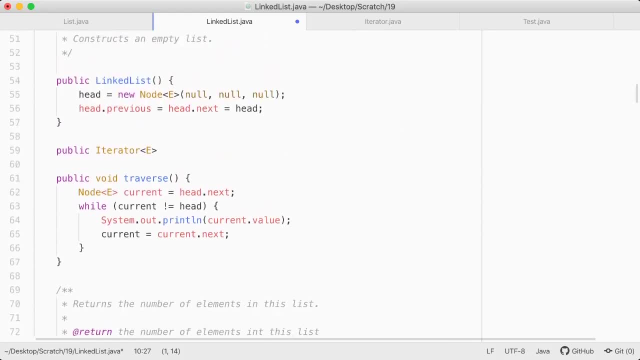 that I want to create where is it that I want to create where is it oh it's right here okay so public oh it's right here okay so public 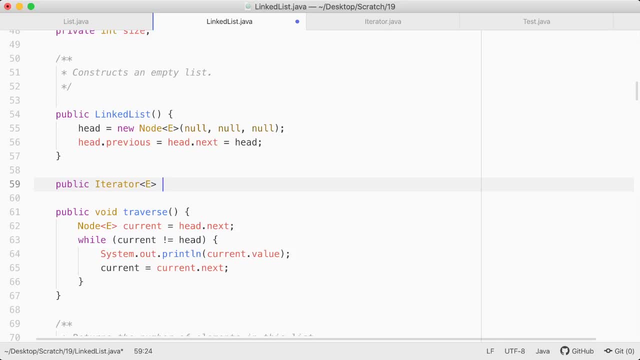 oh it's right here okay so public iterator for some e and if I follow the iterator for some e and if I follow the iterator for some e and if I follow the nomenclature of Java they're calling 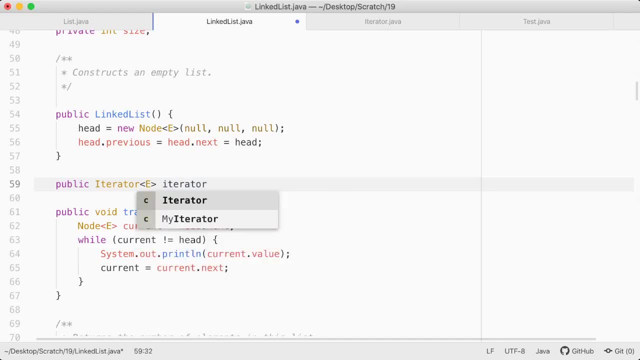 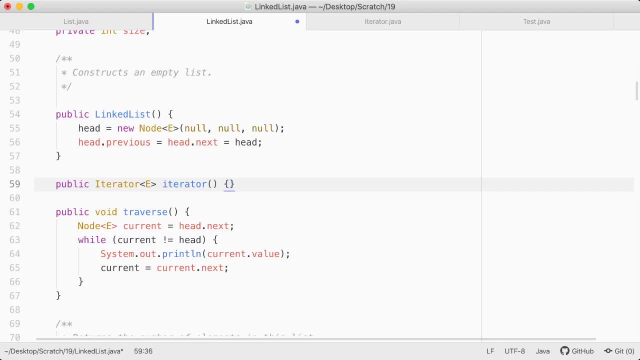 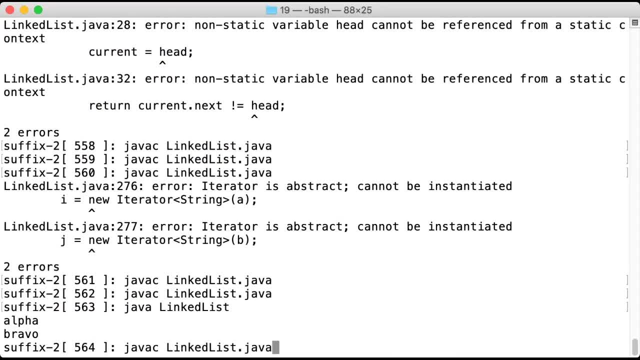 let's see if this compiles let's see if this compiles 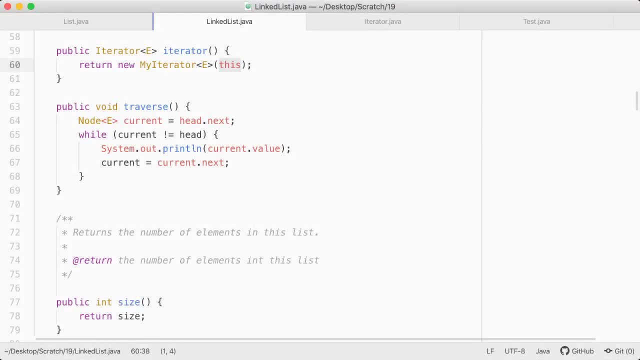 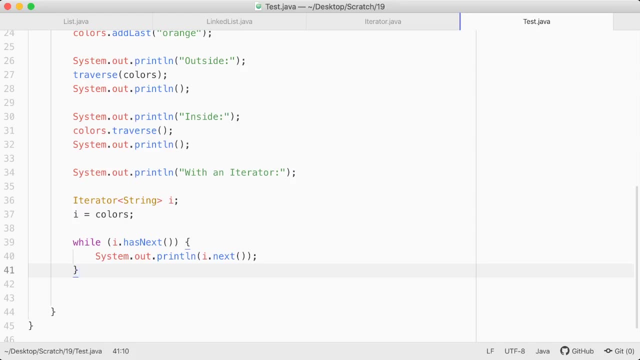 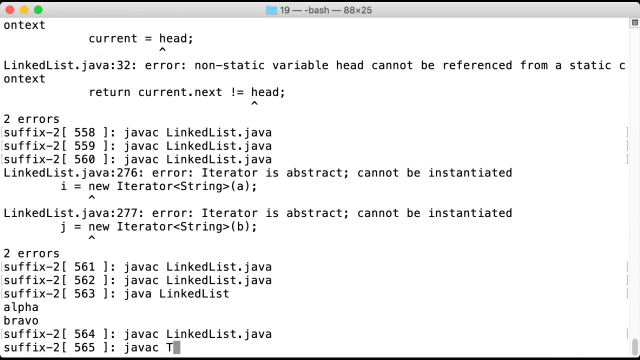 let's see if this compiles compiles let's see how we would use this compiles let's see how we would use this compiles let's see how we would use this from outside so here I is an iterator from outside so here I is an iterator from outside so here I is an iterator but it's no longer true that linked list but it's no longer true that linked list but it's no longer true that linked list implements implements implements the iterator and the iterator implements the iterator and the iterator rather linked list provides a the iterator rather linked list provides a the iterator rather linked list provides a method called iterator that returns on method called iterator that returns on method called iterator that returns on it an iterator on this list 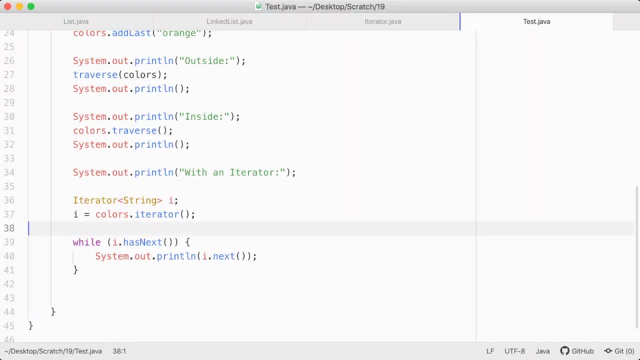 see it works we've created an iterator 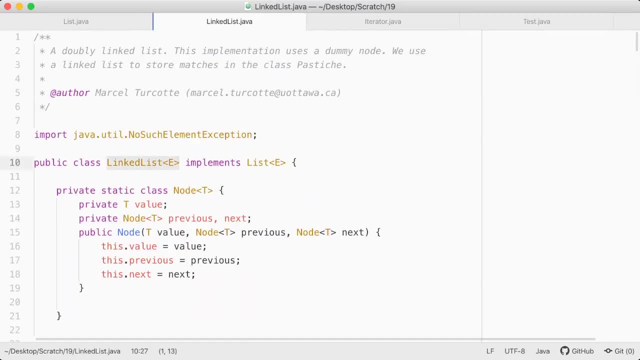 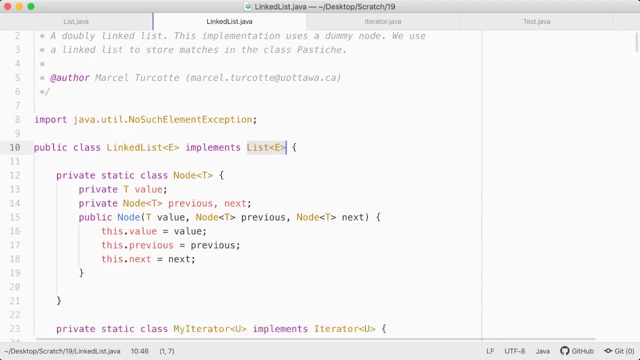 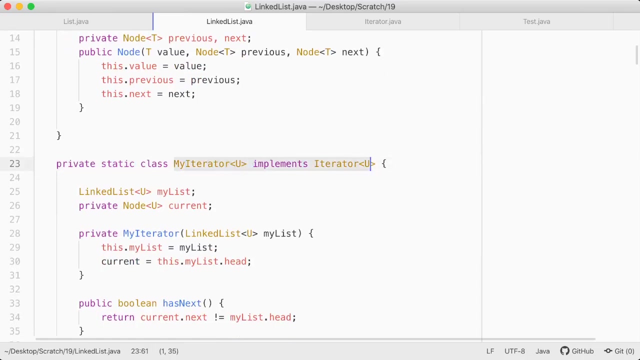 see it works we've created an iterator so what's an iterator so it's no longer so what's an iterator so it's no longer so what's an iterator so it's no longer true that the list implements the true that the list implements the true that the list implements the iterator the list implements the iterator the list implements the iterator the list implements the interface list only we now created a new interface list only we now created a new interface list only we now created a new static nested class called my iterator static nested class called my iterator static nested class called my iterator and it's this one that's implementing the and it's this one that's implementing the and it's this one that's implementing the iterator but because it's a static iterator but because it's a static iterator but because it's a static nested class it needs to be told to nested class it needs to be told to nested class it needs to be told to which list it belongs which what is the 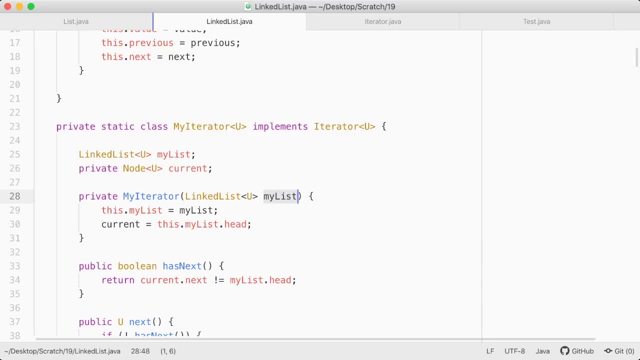 which list it belongs which what is the which list it belongs which what is the list that this iterator will be list that this iterator will be list that this iterator will be iterating when it's created where does 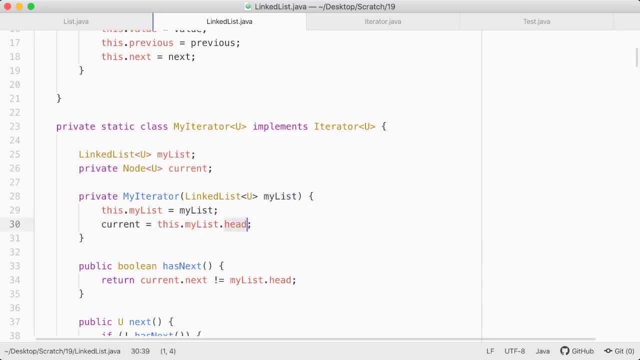 iterating when it's created where does iterating when it's created where does it find the header of the list where it find the header of the list where it find the header of the list where does it find the variable head it's by 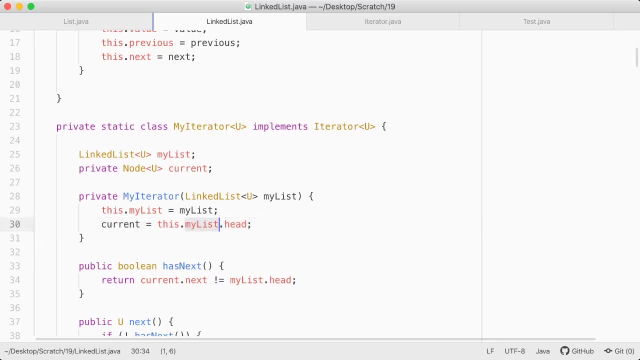 does it find the variable head it's by does it find the variable head it's by using its variable my list here using its variable my list here using its variable my list here 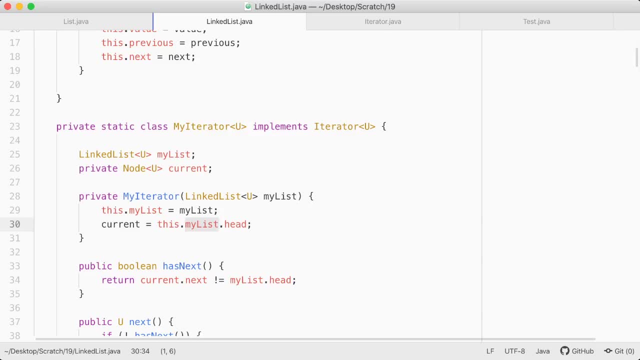 okay so that could be the end of the 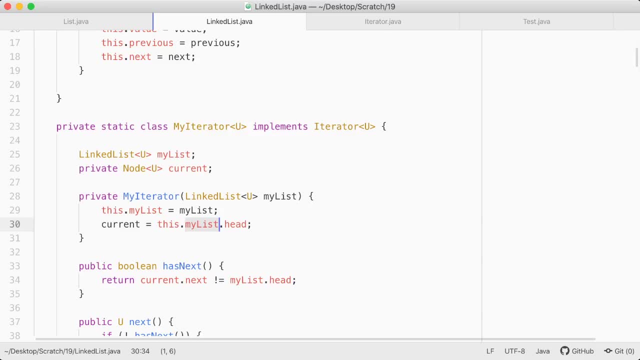 okay so that could be the end of the okay so that could be the end of the story that could be it that could be our story that could be it that could be our story that could be it that could be our iterator it could be just that it would iterator it could be just that it would iterator it could be just that it would be perfect now we've solved the problem be perfect now we've solved the problem 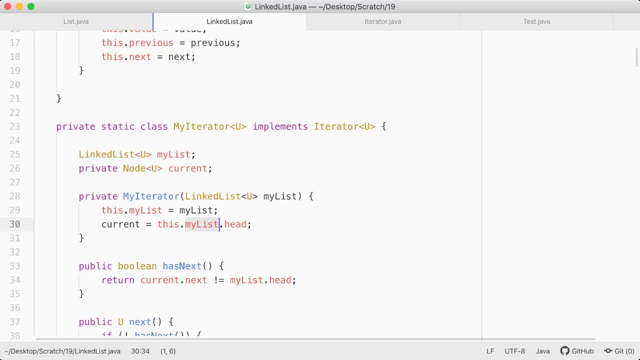 be perfect now we've solved the problem what I mean by that we now have an what I mean by that we now have an what I mean by that we now have an iterator a mechanism that we can create iterator a mechanism that we can create iterator a mechanism that we can create as many iterators as we want for a list as many iterators as we want for a list as many iterators as we want for a list one two three four five ten iterators one two three four five ten iterators one two three four five ten iterators that works we just need to call the that works we just need to call the 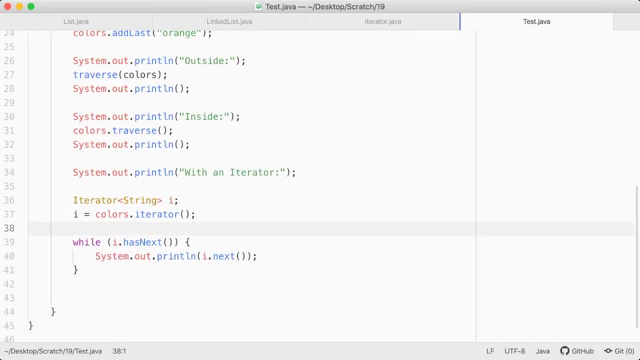 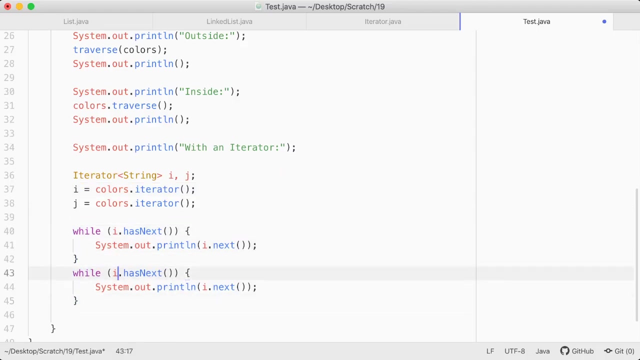 that works we just need to call the method iterator so here if I wanted two method iterator so here if I wanted two method iterator so here if I wanted two iterators so I and J I just need two iterators so I and J I just need two iterators so I and J I just need two calls I and J and we could traverse the calls I and J and we could traverse the calls I and J and we could traverse the list twice here or even we could list twice here or even we could list twice here or even we could intertwine these two lists these two intertwine these two lists these two intertwine these two lists these two while loop if we wanted to we could do while loop if we wanted to we could do while loop if we wanted to we could do what what we want let's see if this 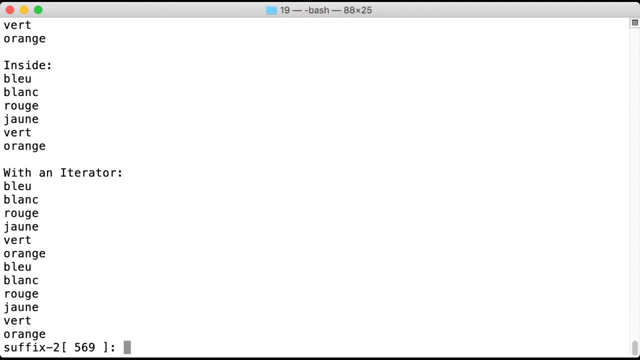 what what we want let's see if this what what we want let's see if this works you have a seat test Java test you 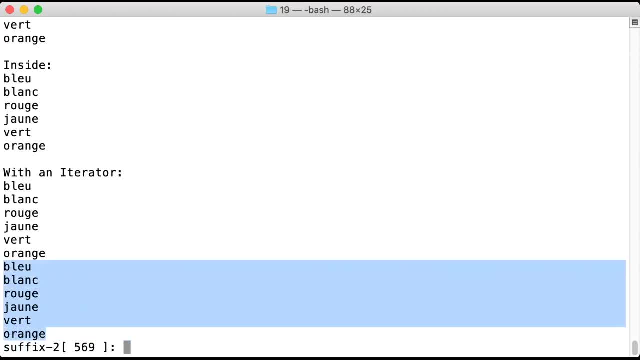 works you have a seat test Java test you works you have a seat test Java test you see with the iterator we printed the see with the iterator we printed the see with the iterator we printed the list twice because we had two iterators list twice because we had two iterators 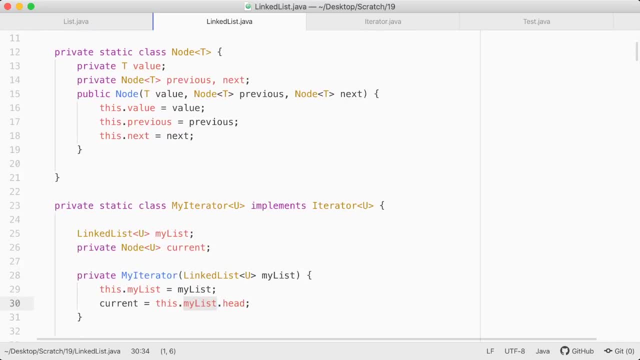 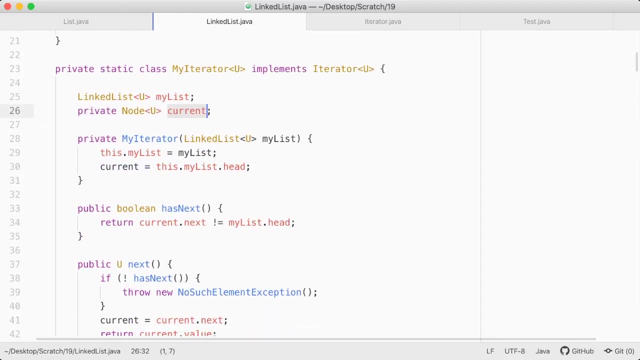 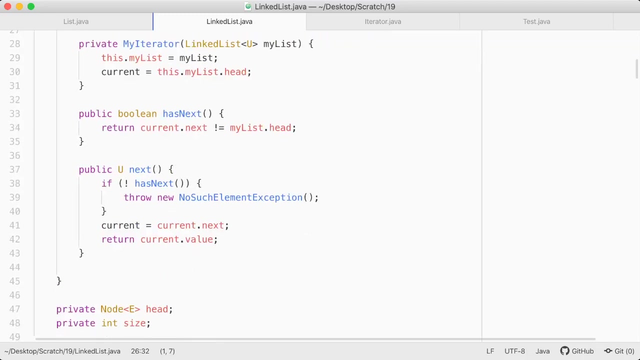 list twice because we had two iterators okay so we have a static nested class my okay so we have a static nested class my okay so we have a static nested class my iterator each iterator memorizes a iterator each iterator memorizes a iterator each iterator memorizes a position inside the list and it's as position inside the list and it's as position inside the list and it's as simple as that I'm not done with the simple as that I'm not done with the 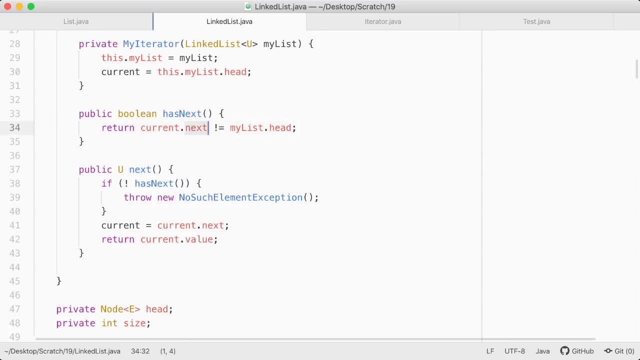 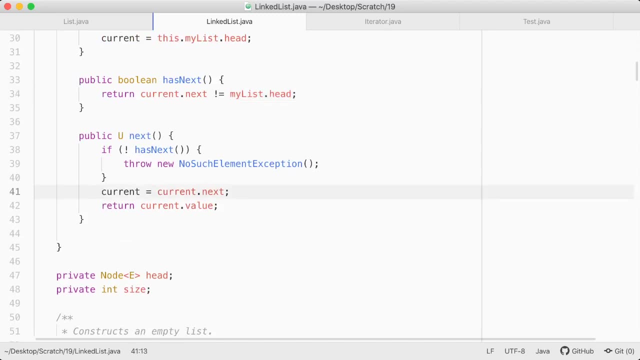 simple as that I'm not done with the iteration if current dot next is iteration if current dot next is iteration if current dot next is different than the dummy node and next different than the dummy node and next different than the dummy node and next simply simply simply simply and next simply and next simply simply simply and next simply moves forward and returns current value moves forward and returns current value moves forward and returns current value okay so as I said that could be enough okay so as I said that could be enough okay so as I said that could be enough we would have solved the problem it's we would have solved the problem it's 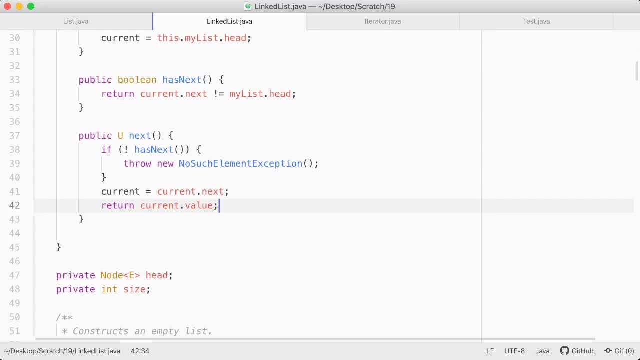 we would have solved the problem it's very fast multiple iterators it works very fast multiple iterators it works 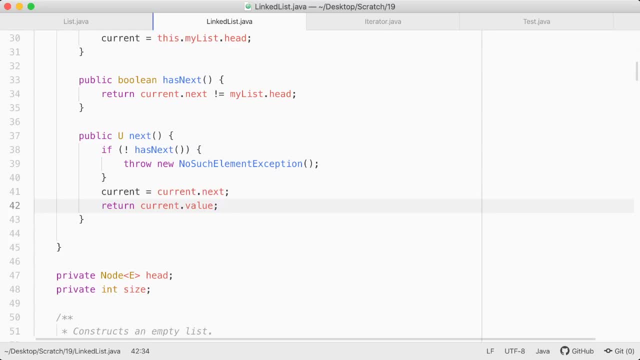 very fast multiple iterators it works but we could do something more elegant but we could do something more elegant but we could do something more elegant the problem that we faced here 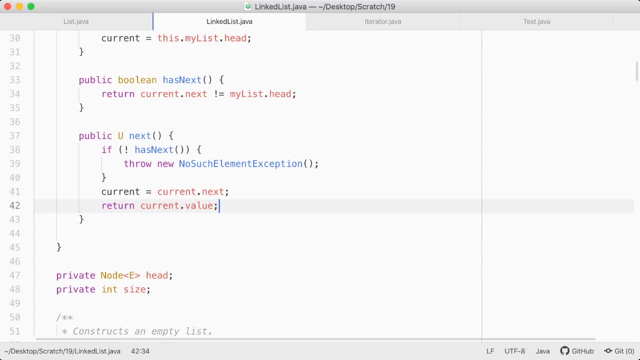 the problem that we faced here the problem that we faced here where the iterator needed to be associated 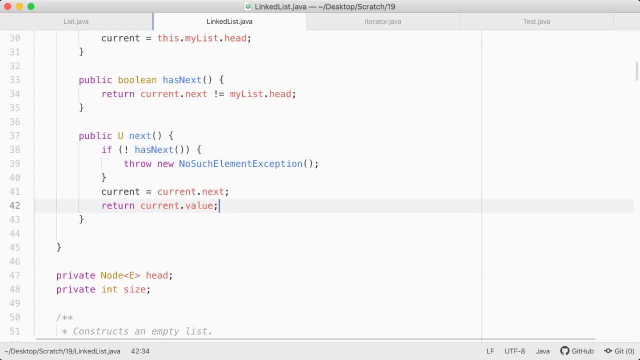 where the iterator needed to be associated where the iterator needed to be associated with one list one object of the outer 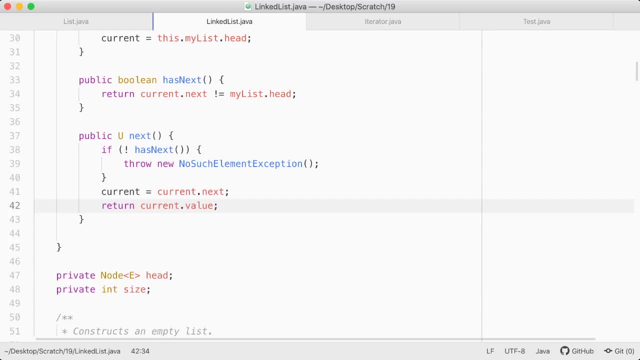 with one list one object of the outer with one list one object of the outer class is a very frequent problem in Java 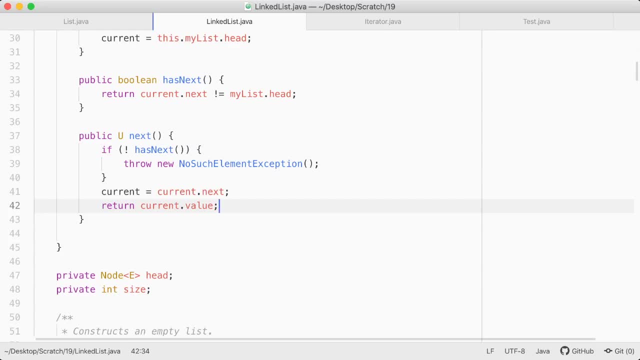 class is a very frequent problem in Java class is a very frequent problem in Java in particular when we are implementing 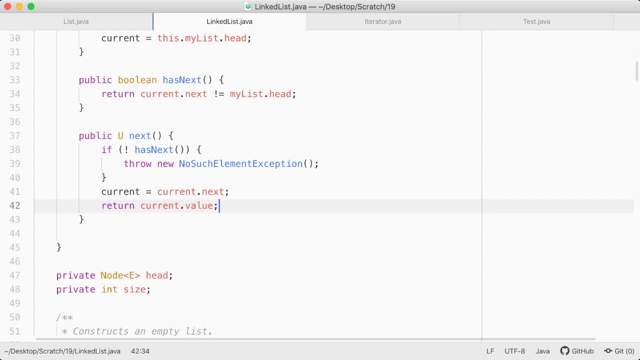 in particular when we are implementing in particular when we are implementing linked structures when we are 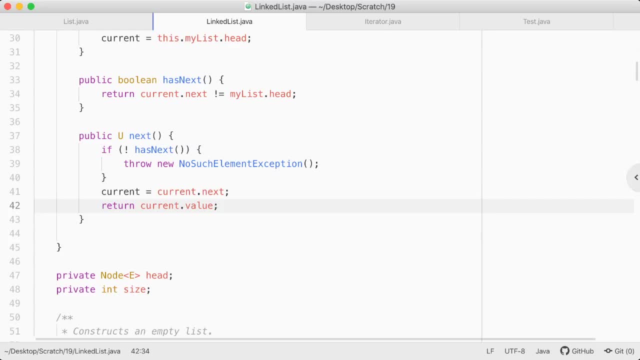 linked structures when we are linked structures when we are implementing GUI sorry graphical user implementing GUI sorry graphical user implementing GUI sorry graphical user interfaces we're facing the interfaces we're facing the 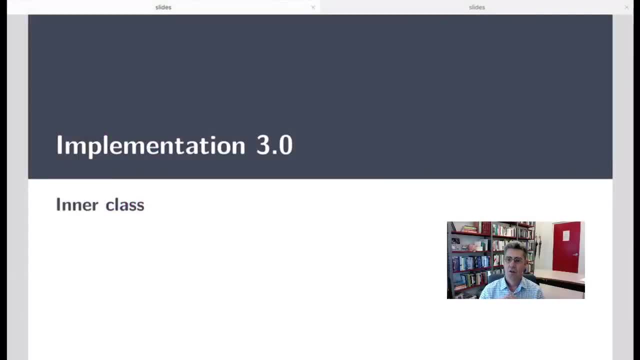 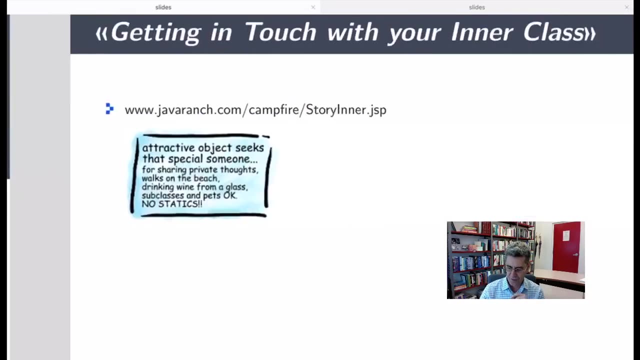 interfaces we're facing the problem often so therefore we're going to problem often so therefore we're going to problem often so therefore we're going to look at the new Java concept that look at the new Java concept that look at the new Java concept that solves this problem in an even better solves this problem in an even better solves this problem in an even better way I don't know if you had a chance to way I don't know if you had a chance to way I don't know if you had a chance to see this but on the internet there is a 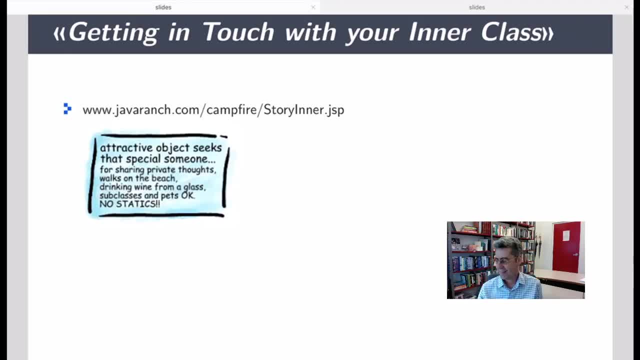 see this but on the internet there is a see this but on the internet there is a website called Java wrench and it has website called Java wrench and it has website called Java wrench and it has very funny stories and one of them is very funny stories and one of them is very funny stories and one of them is called getting in touch with a called getting in touch with a called getting in touch with a touch with your inner class and you have the touch with your inner class and you have the touch with your inner class and you have the URL there and it goes like this URL there and it goes like this URL there and it goes like this attractive object seeks that special attractive object seeks that special attractive object seeks that special someone for sharing private thoughts someone for sharing private thoughts 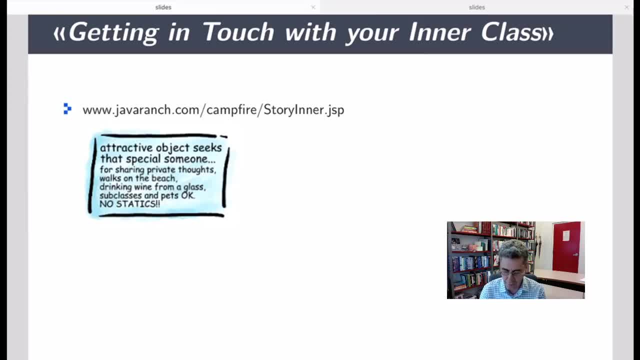 someone for sharing private thoughts walks on the beach drinking wine from a walks on the beach drinking wine from a walks on the beach drinking wine from a glass subclasses and pets are okay no 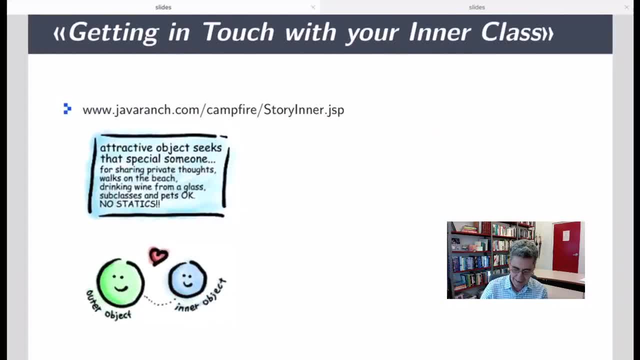 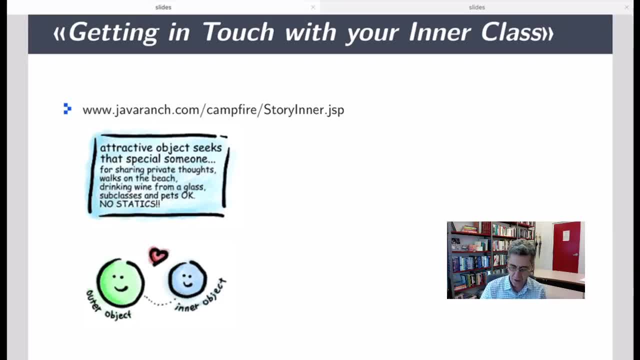 an object of an inner class will be automatically connected to an object of automatically connected to an object of automatically connected to an object of the outer class and there can be as 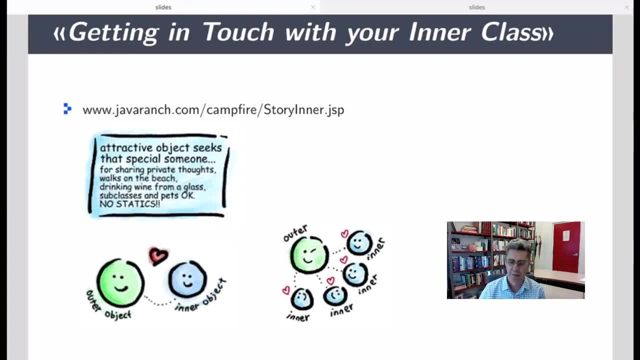 the outer class and there can be as the outer class and there can be as many objects of these inner classes as 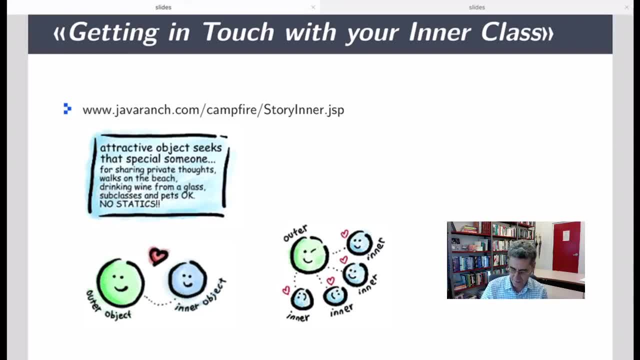 many objects of these inner classes as many objects of these inner classes as we want what's an inner class simply we want what's an inner class simply 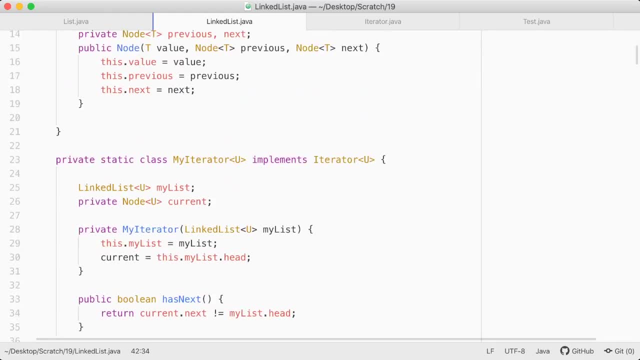 we want what's an inner class simply this we this we this we move the keyword static move the keyword static 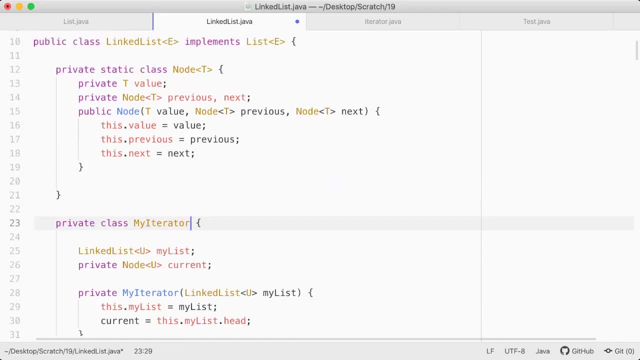 move the keyword static now this iterator now this iterator now this iterator has access to the type parameter has access to the type parameter has access to the type parameter of the class this of the class this 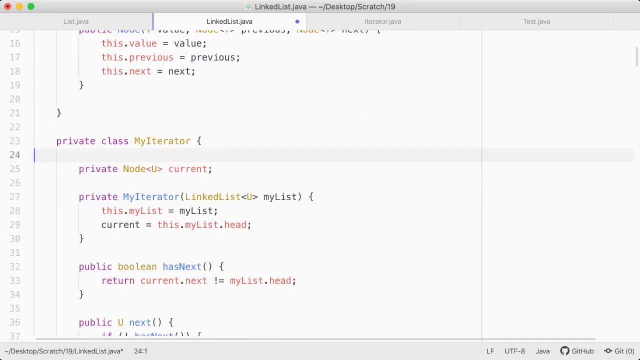 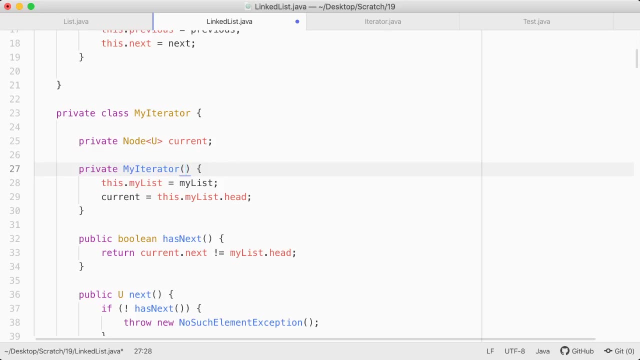 of the class this connection that we were making connection that we were making connection that we were making ourself is now automatic ourself is now automatic ourself is now automatic now the object because it it's created now the object because it it's created now the object because it it's created from from from a non-static nested class is will this a non-static nested class is will this a non-static nested class is will this object will be automatically connected object will be automatically connected object will be automatically connected to the outer object that created it why to the outer object that created it why to the outer object that created it why we do this because the iterator now has 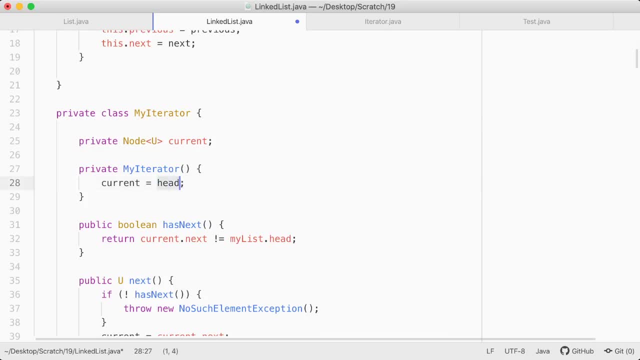 we do this because the iterator now has we do this because the iterator now has access to the instance variable head of access to the instance variable head of access to the instance variable head of its outer object an object of an inner its outer object an object of an inner 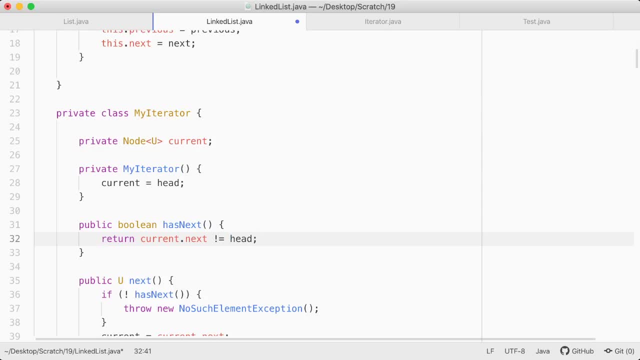 its outer object an object of an inner class is connected to its outer object class is connected to its outer object class is connected to its outer object and has access to the instance variable and has access to the instance variable 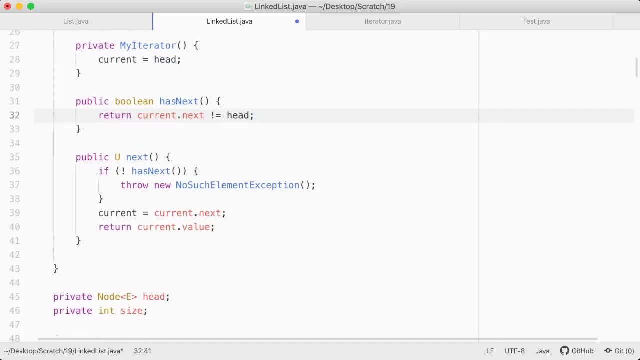 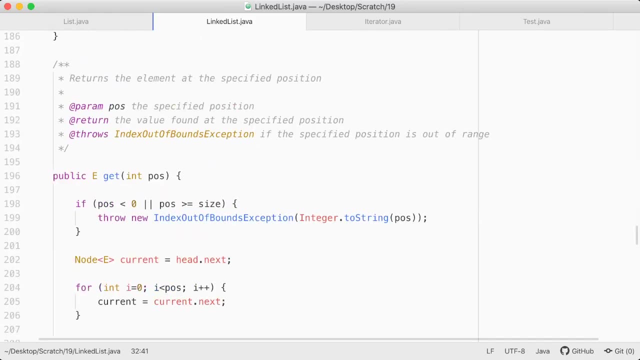 and has access to the instance variable of the outer object okay I'm going to remove my main method okay I'm going to remove my main method 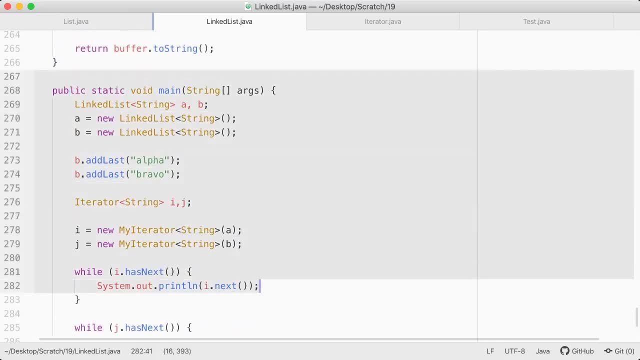 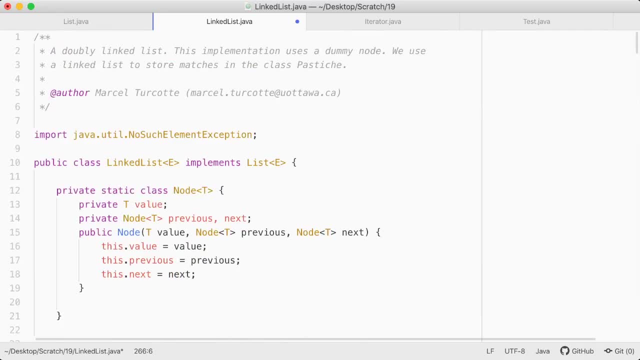 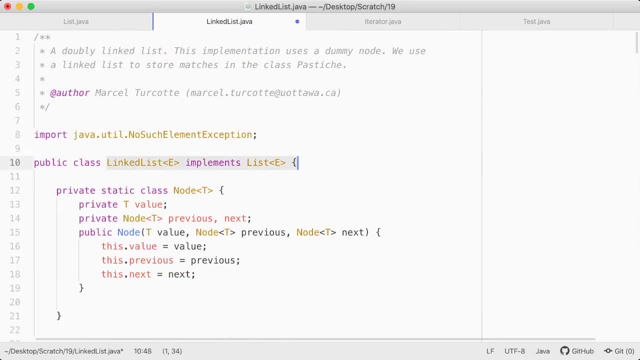 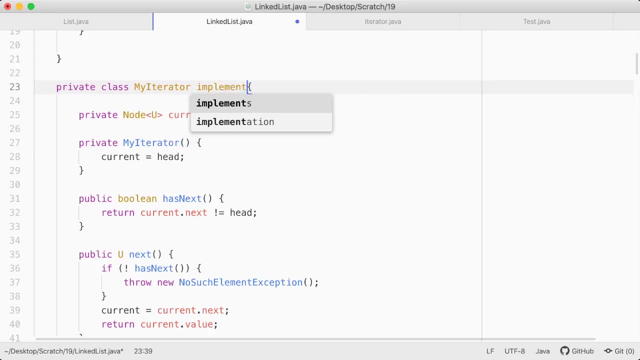 okay so let's review what we have it's okay so let's review what we have it's still the list the linked list is a list still the list the linked list is a list still the list the linked list is a list an iterator aha will implement the an iterator aha will implement the an iterator aha will implement the interface iterator good idea that we interface iterator good idea that we interface iterator good idea that we review the code so it's an object of the review the code so it's an object of the review the code so it's an object of the class my iterator that implements the class my iterator that implements the class my iterator that implements the interface iterator 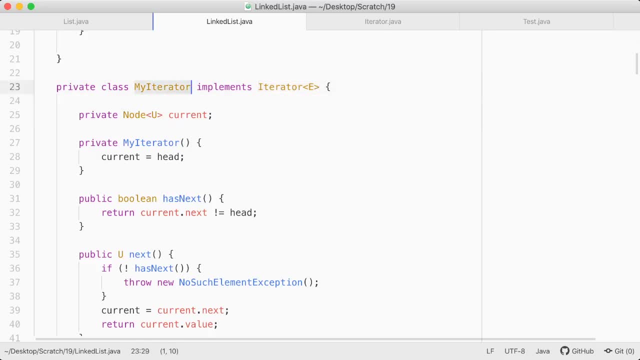 interface iterator interface iterator this object no longer needs a type value 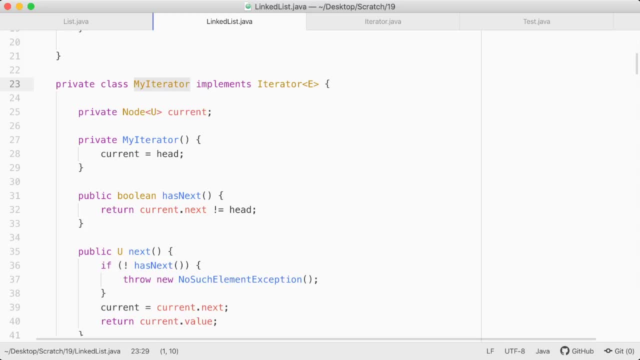 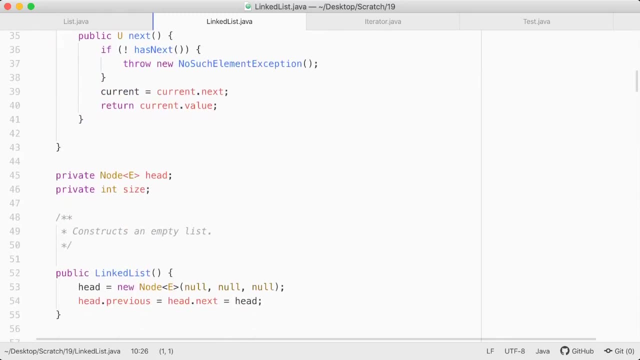 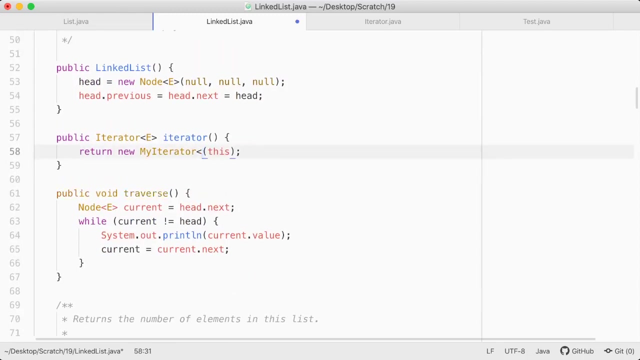 this object no longer needs a type value this object no longer needs a type value because it already gets the type from because it already gets the type from because it already gets the type from its outer object and now we also need to its outer object and now we also need to its outer object and now we also need to change this when we create the object change this when we create the object change this when we create the object my iterator because we act my iterator because we act 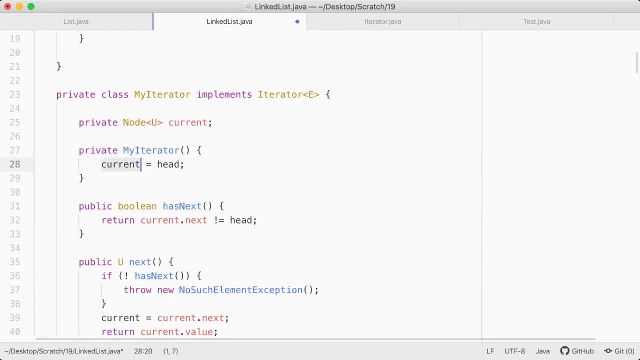 my iterator because we act we actually no longer yes we need a we actually no longer yes we need a we actually no longer yes we need a constructor like this constructor like this 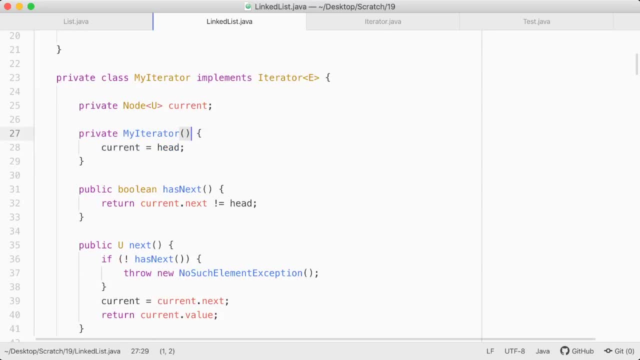 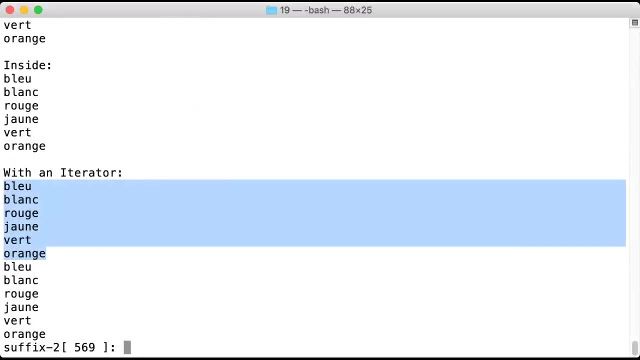 constructor like this but we no longer to tell this but we no longer to tell this but we no longer to tell this this my iterator this my iterator this my iterator who's the other object it knows it who's the other object it knows it who's the other object it knows it okay so okay so okay so we have made many changes now 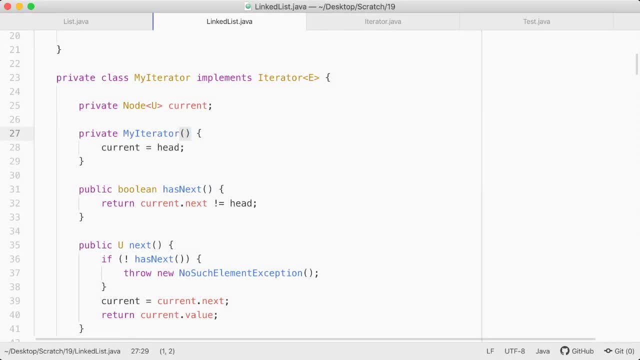 we have made many changes now we have made many changes now okay okay okay was was was a bit careless here 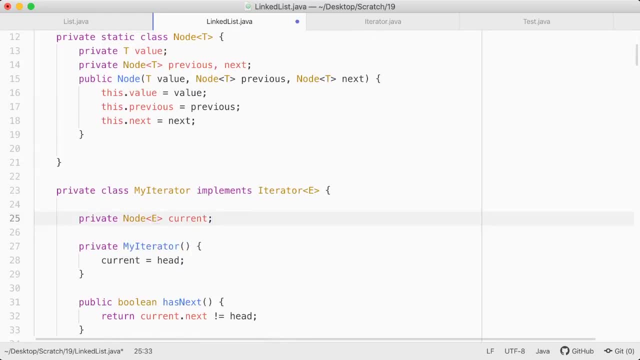 a bit careless here a bit careless here current is pointing at nodes is pointing at nodes is pointing at nodes to store values of type e 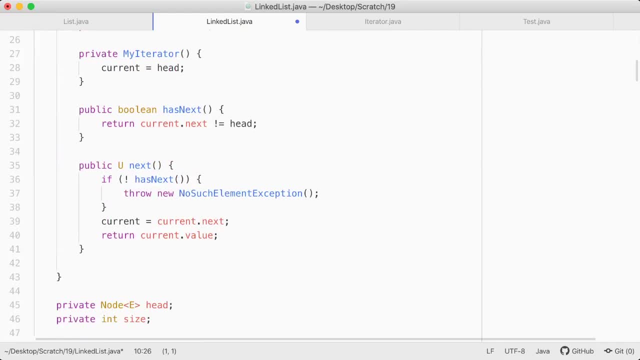 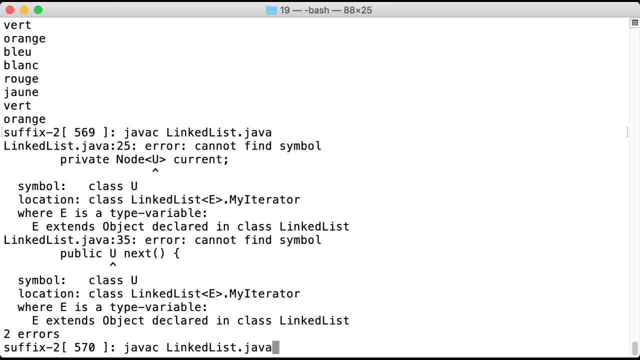 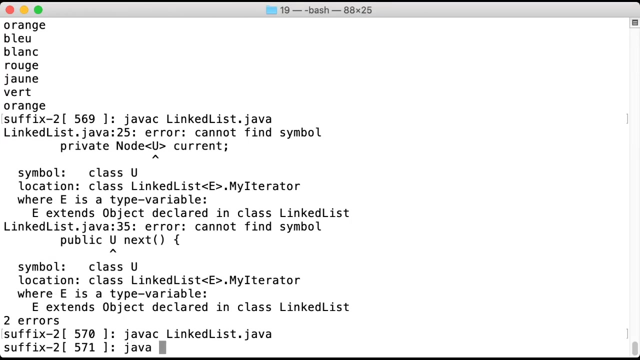 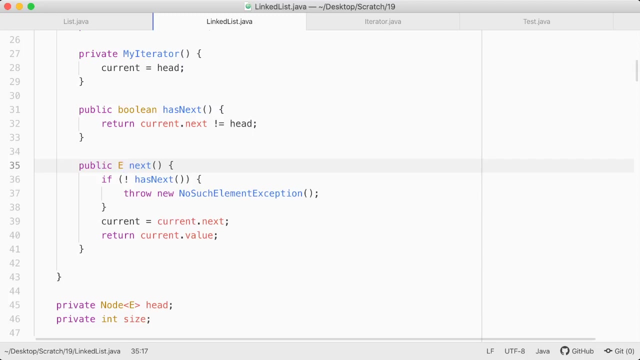 to store values of type e to store values of type e just like my outer object just like my outer object just like my outer object when i'm returning something it's of when i'm returning something it's of when i'm returning something it's of type e does it work does it work yes it does yes it does yes it does okay so a fairly okay so a fairly okay so a fairly simple but deep idea 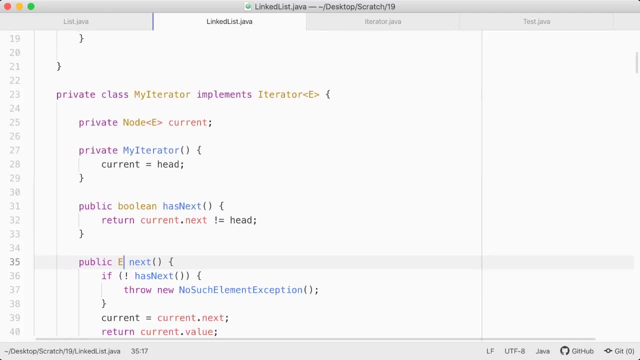 simple but deep idea simple but deep idea in java we often need in java we often need in java we often need to have a nested class that will be 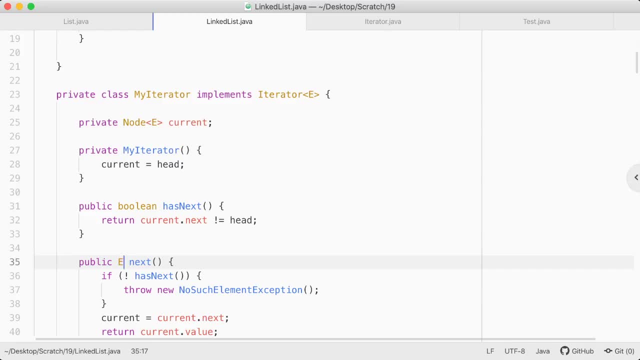 to have a nested class that will be to have a nested class that will be creating some implementation 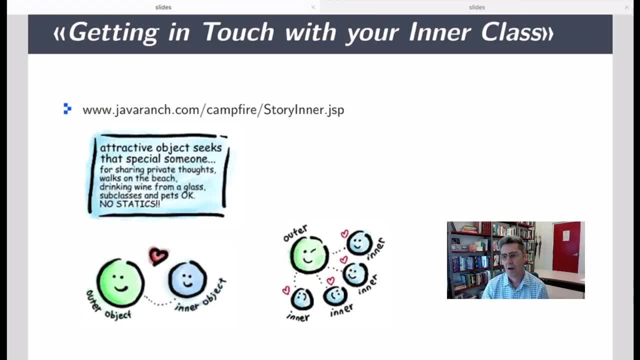 creating some implementation creating some implementation we want this we want this we want this object to be connected to the outer object to be connected to the outer object to be connected to the outer object 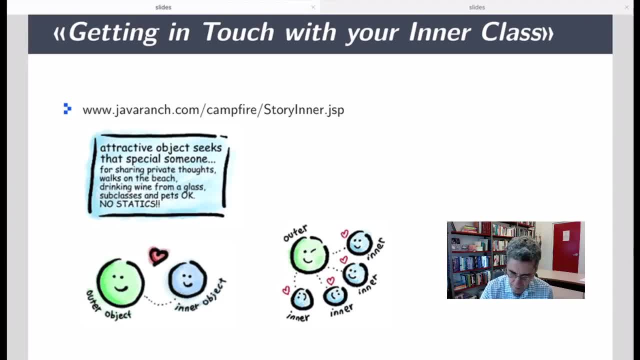 object so here so here so here let me let me let me show you show you show you the inner objects are objects of the the inner objects are objects of the the inner objects are objects of the class class 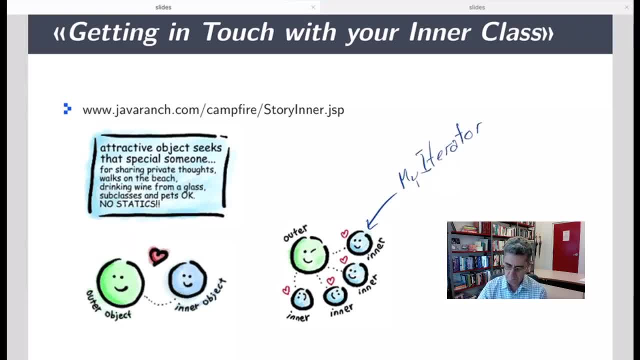 class my iterator the outer object is an object the outer object is an object the outer object is an object of the class linked list of the class linked list 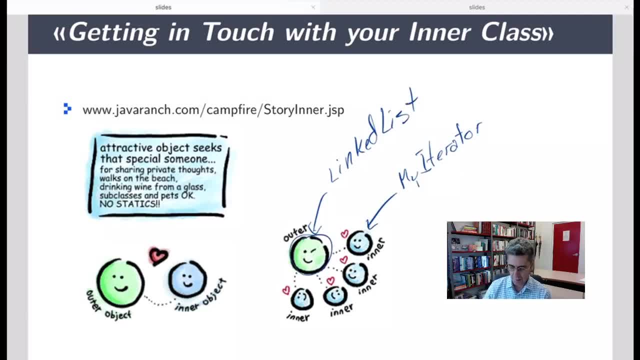 of the class linked list it's the object of the class it's the object of the class it's the object of the class linked list my of the class linked list that is my of the class linked list that is my of the class linked list that is creating these my iterator objects okay 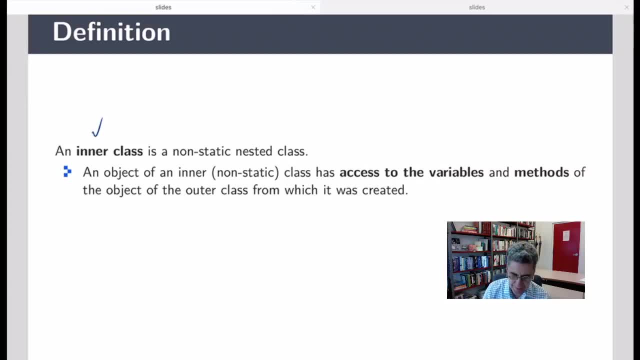 creating these my iterator objects okay creating these my iterator objects okay so an inner class has access to the variables and the 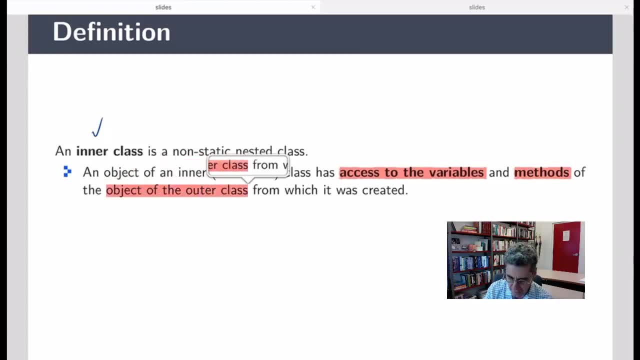 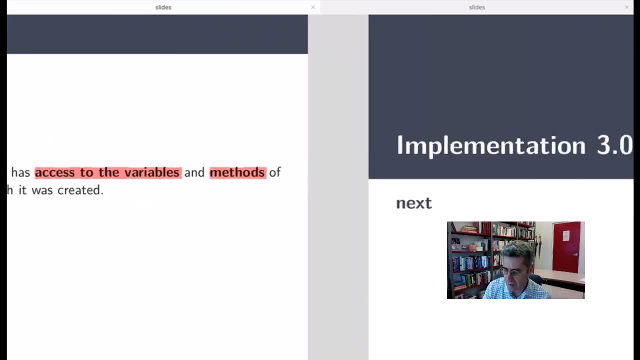 has access to the variables and the has access to the variables and the methods of the object of the outer class methods of the object of the outer class methods of the object of the outer class and such an object can only be created and such an object can only be created and such an object can only be created in the context of an outer object okay 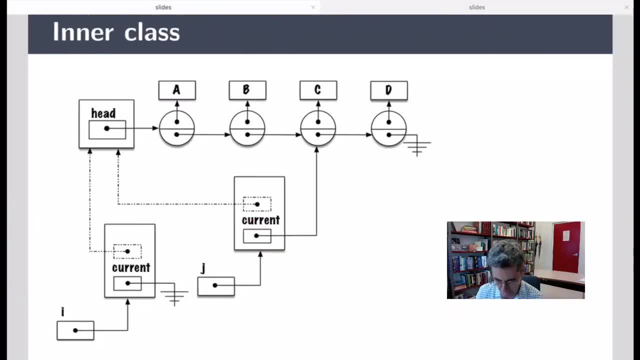 okay okay just moving forward showing you here so just moving forward showing you here so just moving forward showing you here so before we had to create this connection before we had to create this connection before we had to create this connection between the iterator and its list between the iterator and its list between the iterator and its list ourself ourself ourself if if if we drop the keyword static then the my we drop the keyword static then the my we drop the keyword static then the my iterator object needs to be created from iterator object needs to be created from 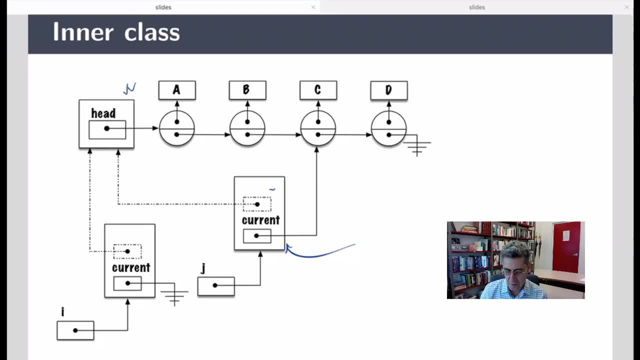 iterator object needs to be created from an instance method of the outer object an instance method of the outer object an instance method of the outer object and Java will take care of making this and Java will take care of making this and Java will take care of making this connection between the iterator and its connection between the iterator and its connection between the iterator and its outer object its linked list it will be outer object its linked list it will be outer object its linked list it will be done for us we say that we need to done for us we say that we need to done for us we say that we need to say that the namespace is shared meaning that say that the namespace is shared meaning that say that the namespace is shared meaning that when a method has next of a my when a method has next of a my when a method has next of a my iterator is talking about head head is 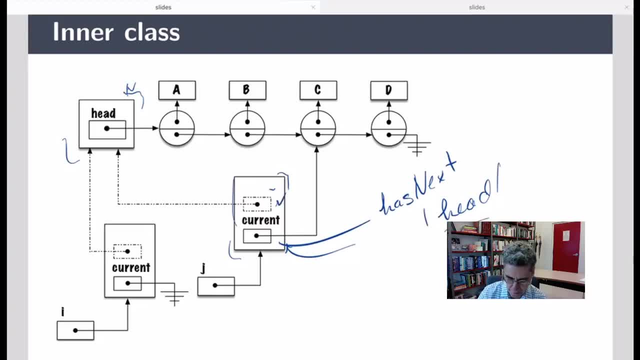 iterator is talking about head head is iterator is talking about head head is not a variable of the object my not a variable of the object my not a variable of the object my iterator head is a variable of its outer iterator head is a variable of its outer 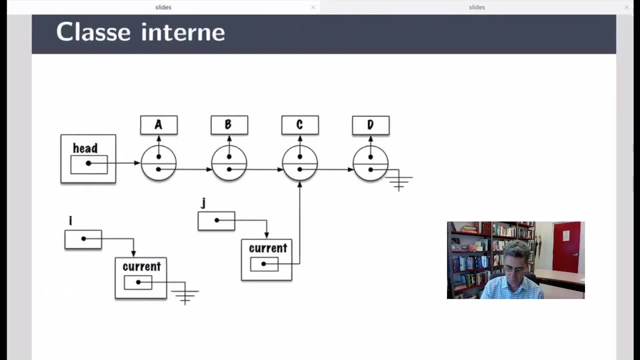 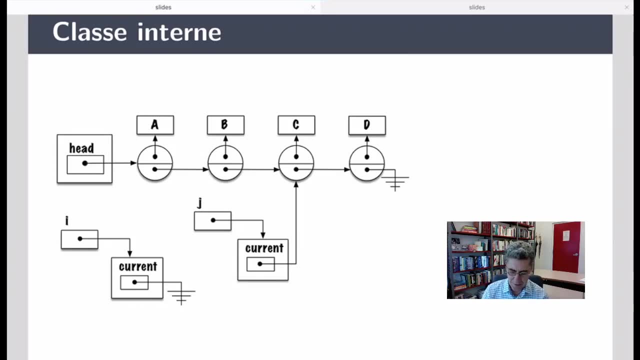 iterator head is a variable of its outer object okay so this is our final object okay so this is our final object okay so this is our final implementation it's a implementation it's a implementation it's a inner class the iterator is an object inner class the iterator is an object 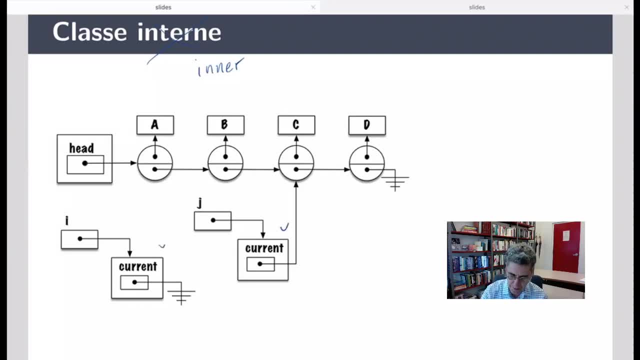 inner class the iterator is an object of an inner class this allows us to of an inner class this allows us to of an inner class this allows us to create as many iterators as we want for create as many iterators as we want for 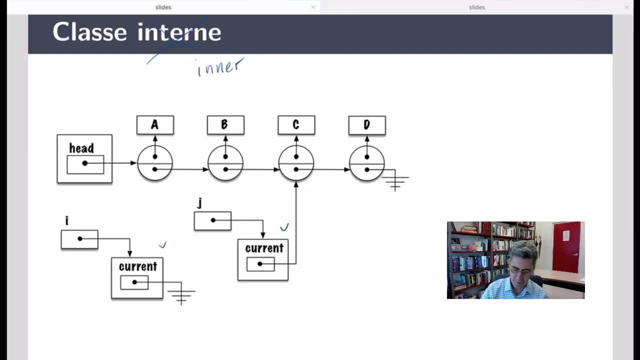 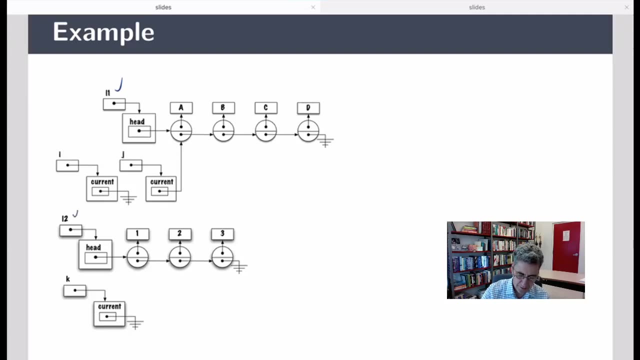 create as many iterators as we want for a list each one of them because they're a list each one of them because they're a list each one of them because they're from a non static nested class has from a non static nested class has from a non static nested class has access to the variables of the other access to the variables of the other access to the variables of the other object that's what what that's what we object that's what what that's what we object that's what what that's what we wanted this allows us to have multiple wanted this allows us to have multiple wanted this allows us to have multiple lists and multiple iterators so here I lists and multiple iterators so here I lists and multiple iterators so here I is associated with the list create is associated with the list create is associated with the list create designated by l1 because I was created 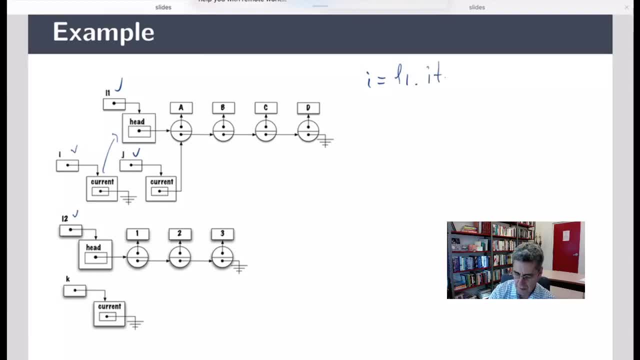 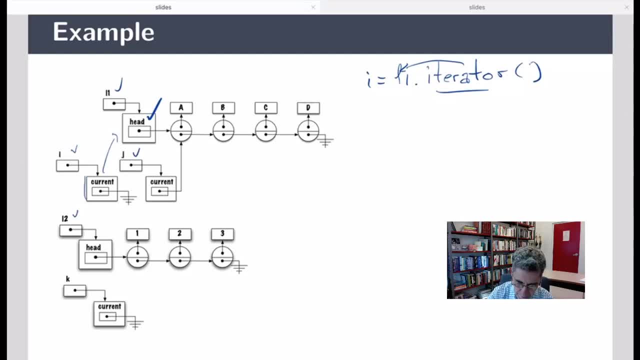 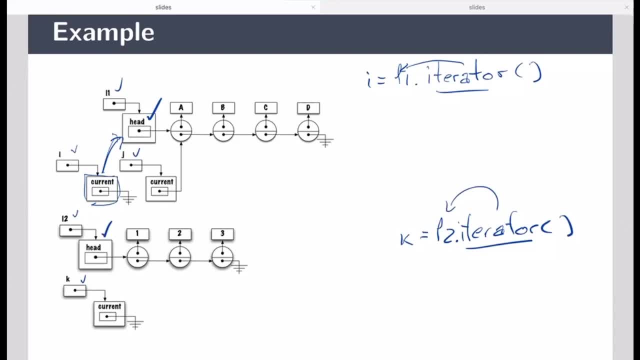 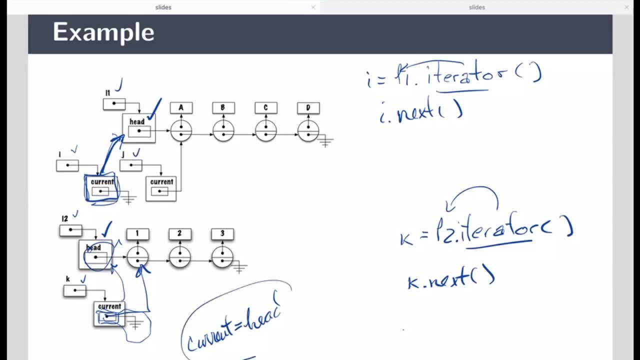 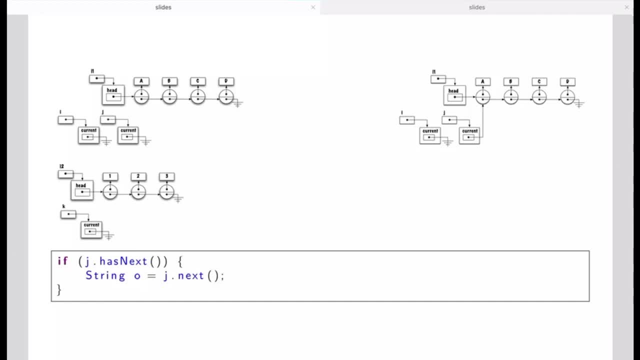 okay so here is it true that j dot is j dot has next true yes copy head into current 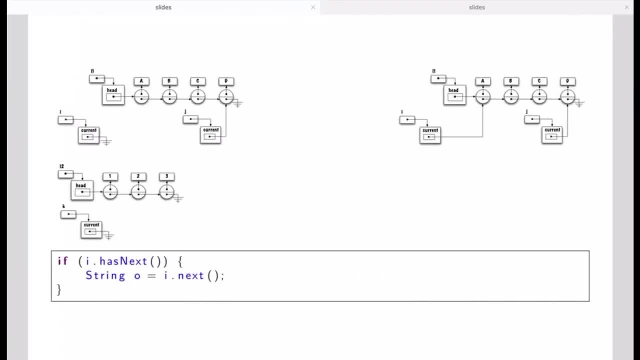 is it true that i dot next is 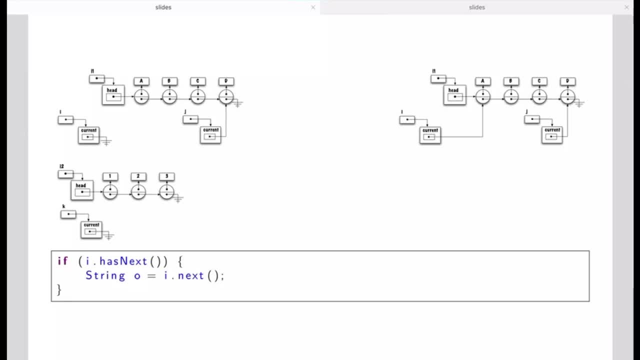 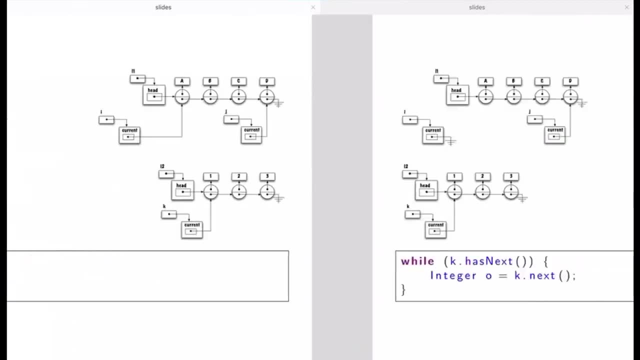 valid not is returning true yes we call next it moves forward 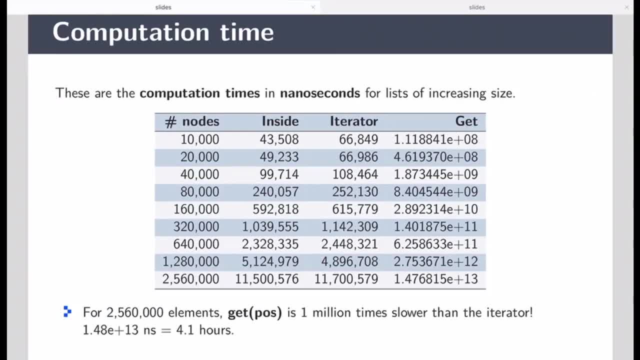 etc okay and this is very fast i've now created 2014 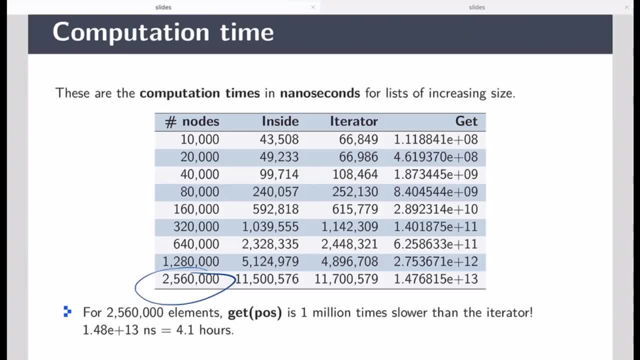 2,500,000 nodes we see that the implementations that are 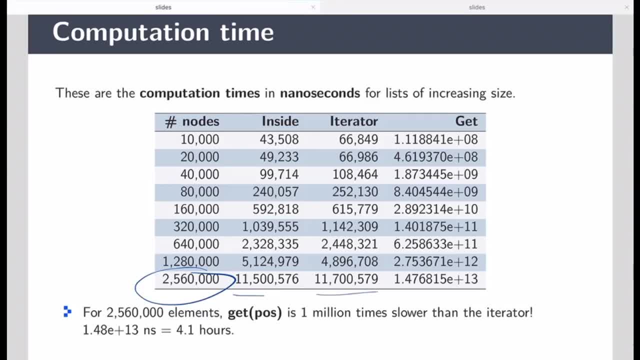 inside the list and using the iterator are now very fast still yet the implementation that is using get in that case was taking 4.1 hours so this is really a valuable value 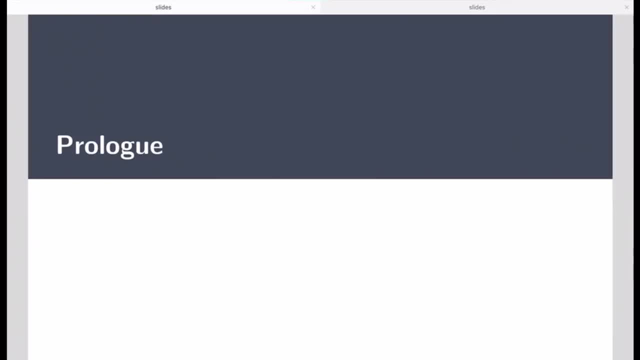 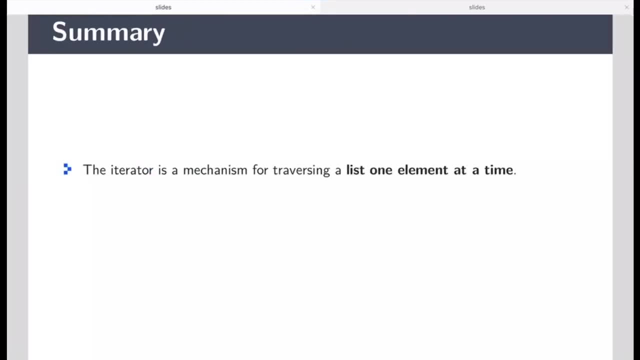 um thing to have so hopefully um you will appreciate how this has allowed us to think about a lot of concepts that are related to object-oriented programming 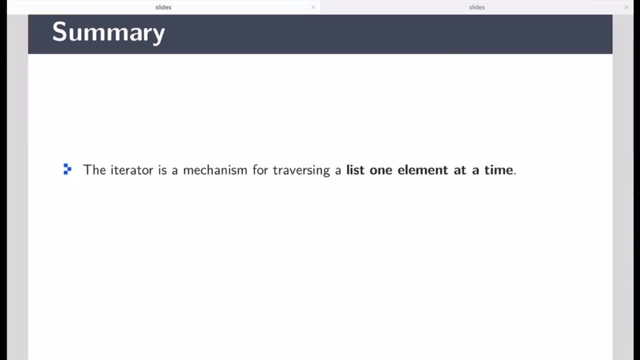 we've been able to create a mechanism that allows us to traverse the list 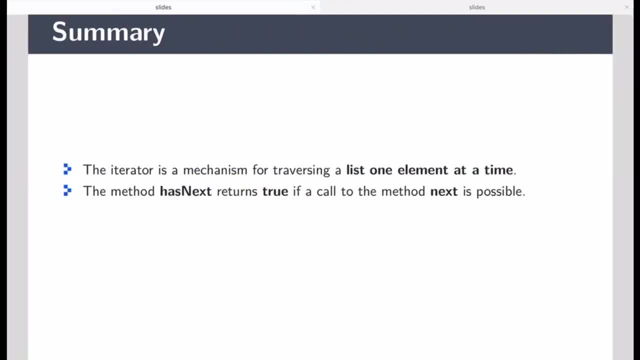 one element at a time the method has next returns true if a call to next is possible 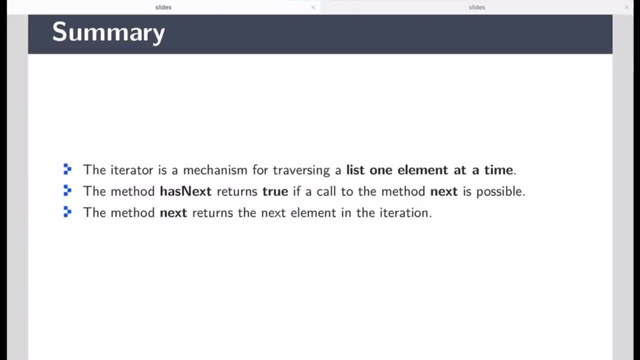 the method next returns the next element in the iteration in order to create our final implementation we've used an inner class this is a nested non-static class and the the idea is that an inner class has access to the variables of the outer object that's why we we use an inner class 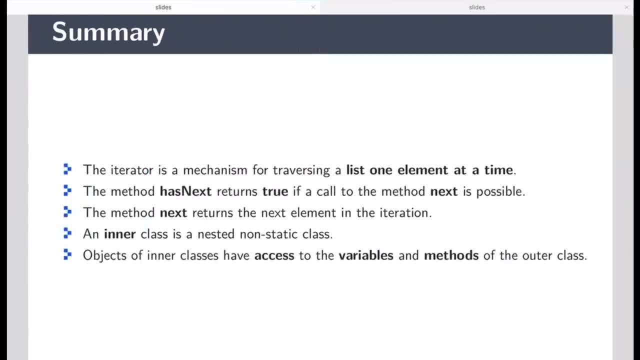 the method next returns the next element in the iteration in order to create our final implementation we've used an inner class this is a nested non-static class and the the idea is that an inner class has access to the variables of the outer object that's why we we use an inner class the method next returns the next element in the iteration in order to create our final implementation we've used an inner class this is a nested non-static class and the the idea is that an inner class has access to the variables of the outer object that's why we we use an inner class the method next returns the next element in order to create our final implementation we've used an inner class this is a nested non-static class and the the idea is that an inner class has access to the variables of the outer object that's why we we use an inner class you should appreciate as well that the class node has no methods it doesn't need to access the variables of the outer object that's why we keep it static 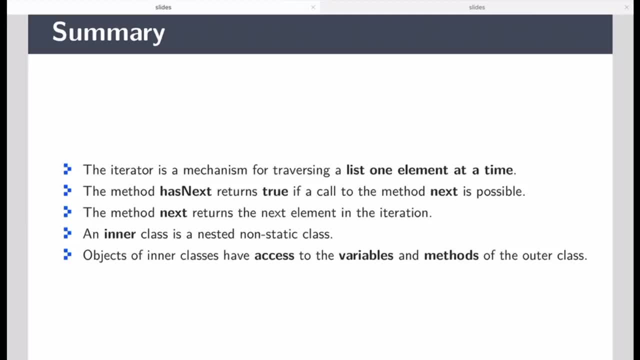 it would create further problems down the road if we were to make the class node not static 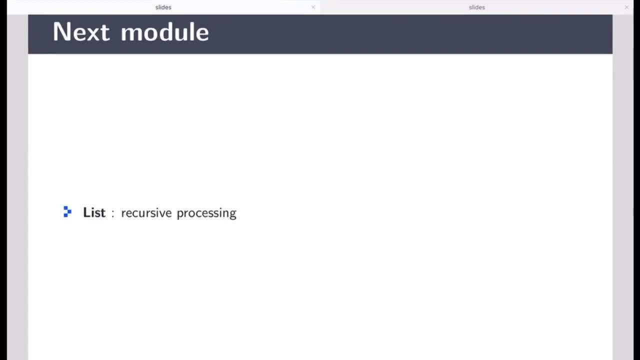 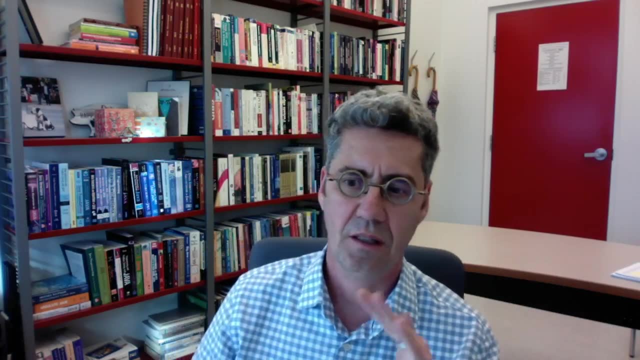 okay so that was it for this lecture in the next lecture we're going to be okay so that was it for this lecture in the next lecture we're going to be talking about recursive list processing so it's going to be 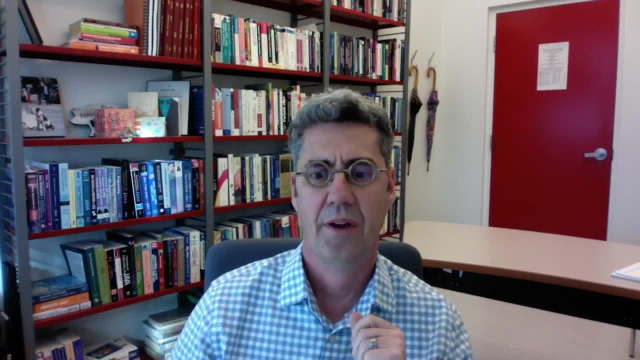 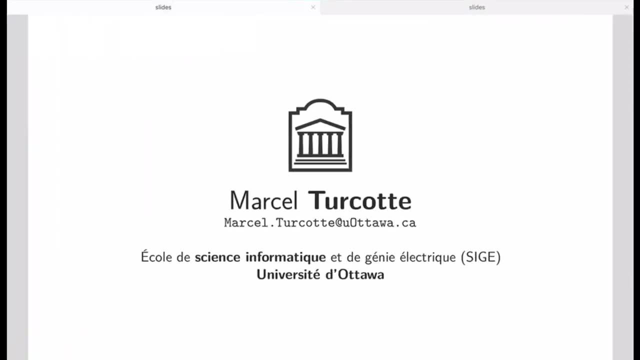 essentially another way of traversing the list but that time we're going to be using recursion